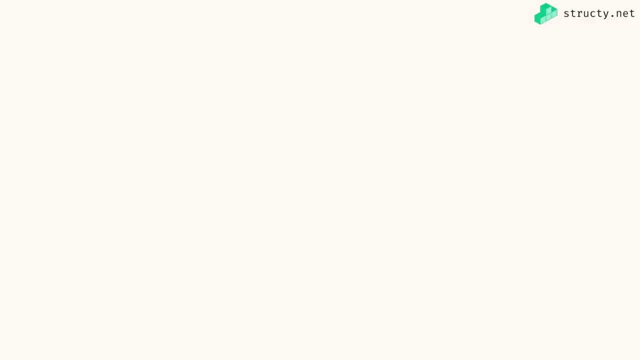 what a linked list is at a high level bird's eye view. The first thing we need to know is that a linked list is a type of data structure, right, So we're organized as data And, in particular, a linked list is made up of many nodes. So, as our first checkpoint here, we need 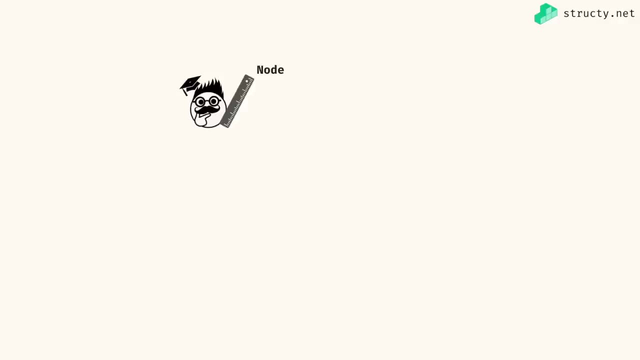 to first understand what a node is. you can think of a node as just a container for some data. So when we conceptually visualize nodes, really think of them as some circles that I can put some data inside. Here I'll put a letter or character inside of my node, But of course you can store. 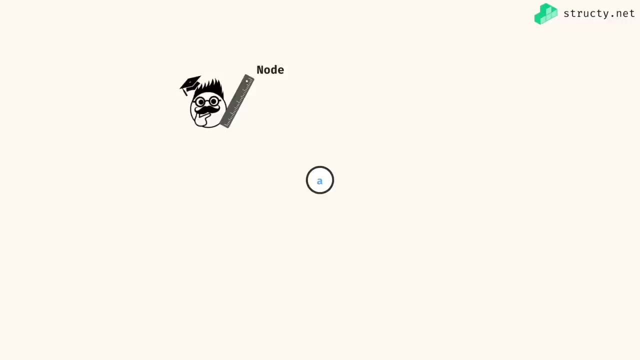 any data you like. it could be strings, numbers, booleans or even other objects, right? And I'm saying that a linked list contains many nodes. So let's say I had a bunch of nodes and they can all contain different pieces of data. So I have the characters ABCD stored in different 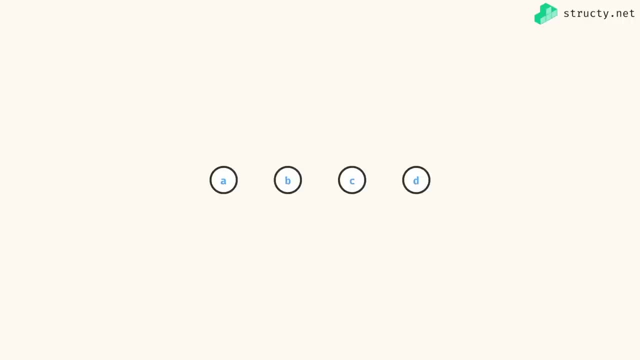 nodes over here And if I wanted to make these nodes a linked list, then what I need to do is add some links. In other words, if I have a node like a, I can make it point to the next node, the data set that is a points to B right. I can also say that 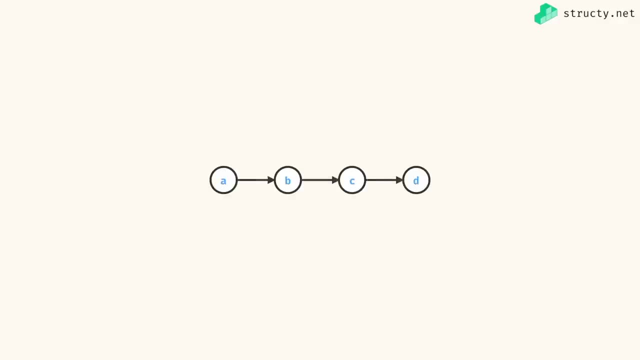 B points to C and C points to D- right, And the term we actually like to use for this is really saying that a is next is B. right? it's going to be very common, a linked list terminology and a pattern we're definitely going to see in the code later on, And now you can already see. 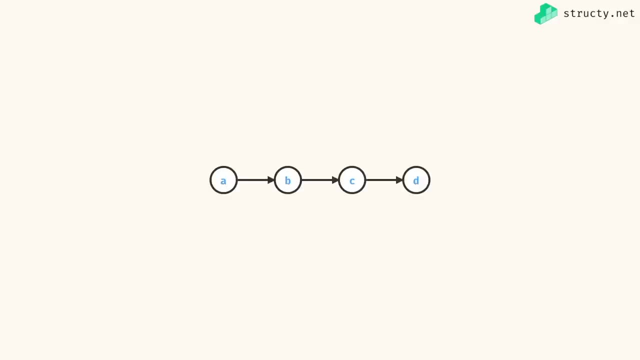 why you call this data structure a linked list. right, I have a bunch of nodes linked together And- important thing to note here- it's about the last node D. right, D is the last node in our linked lists And so, under the hood, we can really represent. 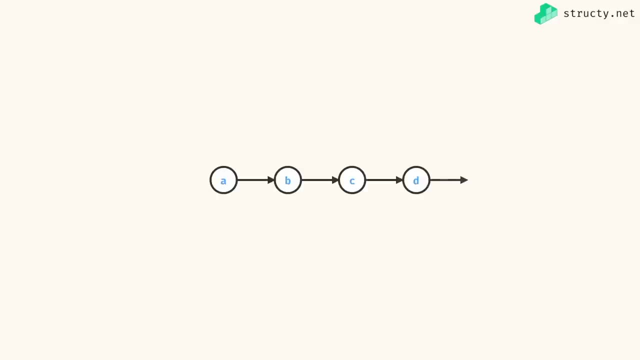 it being the last node, by having its next pointer pointing to nothing. Or, more programmatically, you can have its next set to null, right, the null pointer, and whatever your language of choices. So sometimes during this course, I'm going to explicitly choose to draw out. 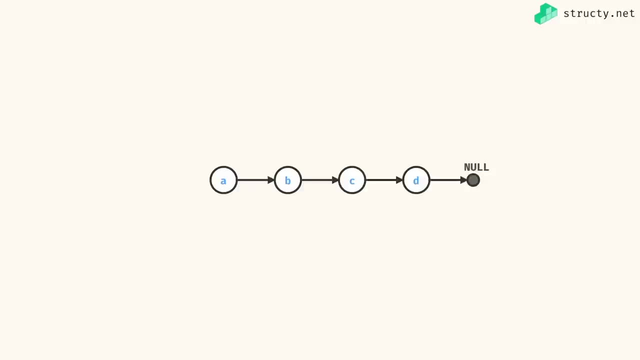 the null node or the null reference, just so we can build some very robust code All right. now that we know what a linked list looks like, I want to introduce some other terminology that you're going to hear right, So when we refer to 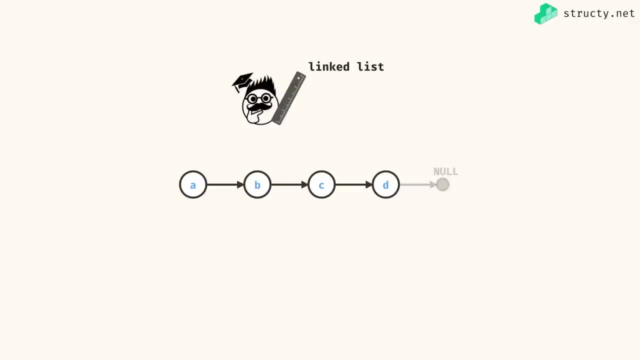 the very, very first node of a linked list, that is, the a node in this diagram, I consider that the head. it's a very common term. In a similar way, we can refer to the very last node in a linked list as the tail right. So if you hear those words in problems, we're referring to the. 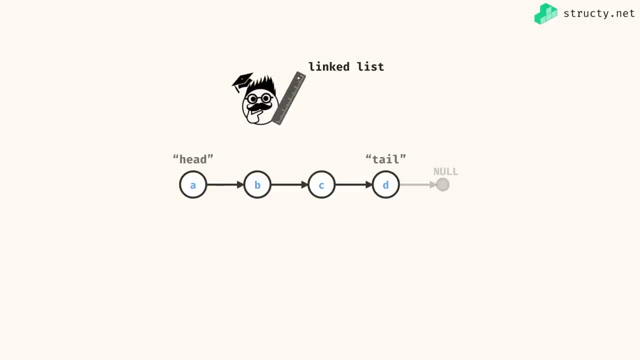 first node and the very last node respectively. right, If you think about it, because I have this sense of different nodes and you know a first node and a second node, we can think of a linked list as an ordered data structure. In other words, if I started at the head of the linked list, 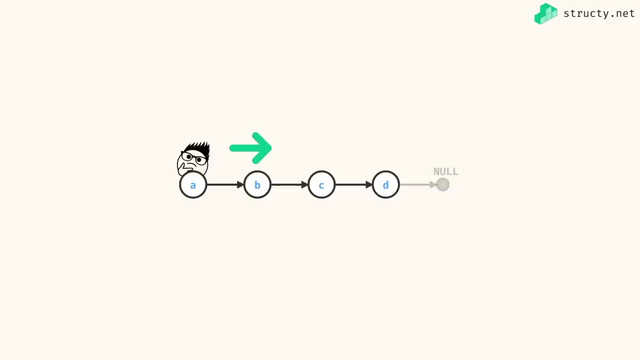 I can just look at this nodes, next pointer, and I can go to the B node. so I can just move to the right And once I'm at the B node I can see that B has an x. that goes to the C node and the C node. 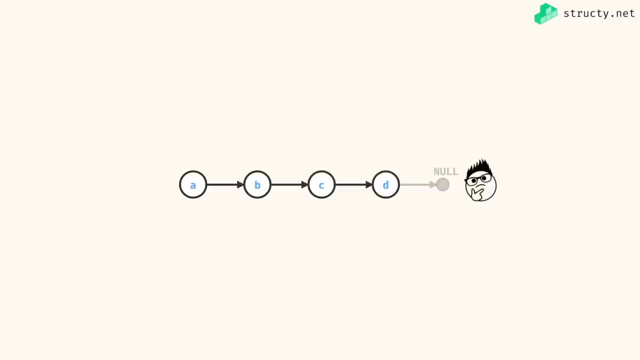 goes to the D node And the D node goes to the null node, which must mean that I'm at the end of the linked list. So it's a very, very key characteristic about a linked list. right, A nice property to leverage about a linked list is that it's an inherently ordered data structure. 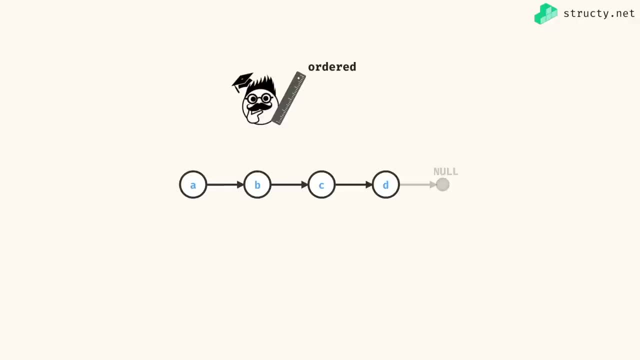 right, If you want to refer to, like, the positions of these nodes and we do that programmer thing of starting at zero, I can see that the head has a position of zero, B has a position of one and then we just go sequentially throughout, right? So there are four nodes within this. 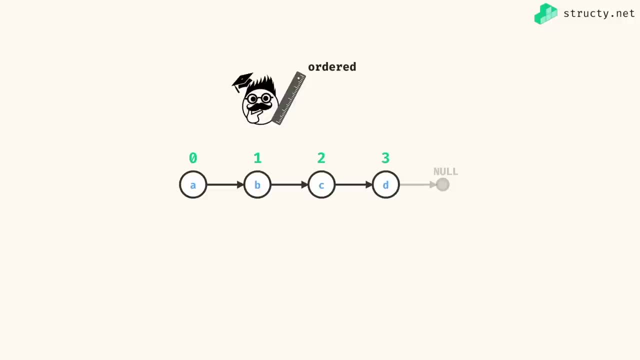 linked list, I can see that the position of the head is zero and the position of the tail is three, And so so far we're probably not seeing the full value of a linked list. like when would this data structure have some real utility over other data structures that? 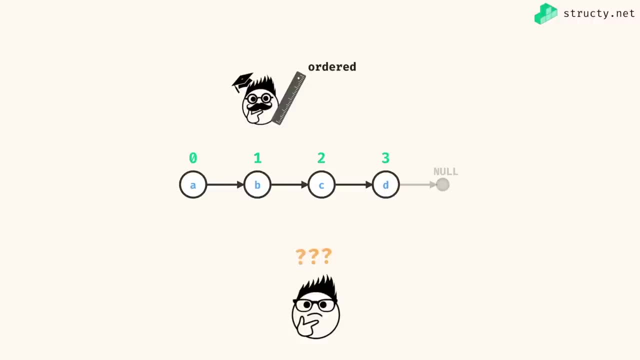 we know about. In other words, you're probably wondering how a linked list is going to work. link list compares to an array, because an array is also an ordered data structure. So let's do that comparison right now. So here I have my linked lists up top, And if I wanted to represent 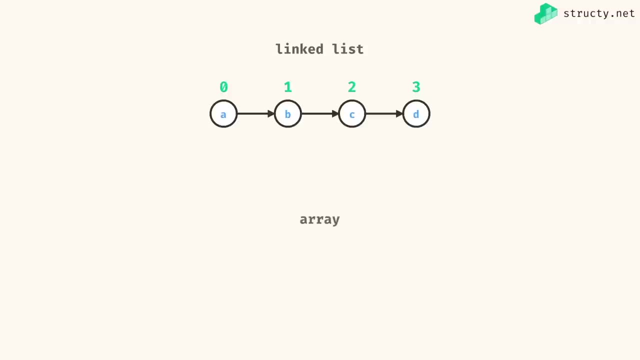 you know a similar data structure, but in an array form. it would look something like this: right, I have an array in memory And I know that that array has some indices, right, So there's a really clear analogy here. I know that the indices of an array correspond to the positions of the 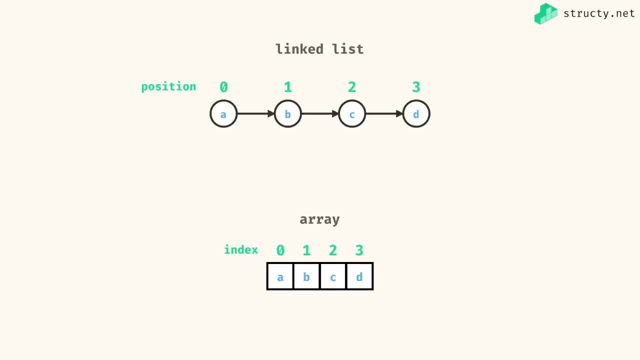 nodes of a linked list. right And obviously my linked list is going to be a linked list. It's made of many nodes, whereas my array has many elements. The most important difference between an array and a linked list is that an array must be stored contiguously in memory. 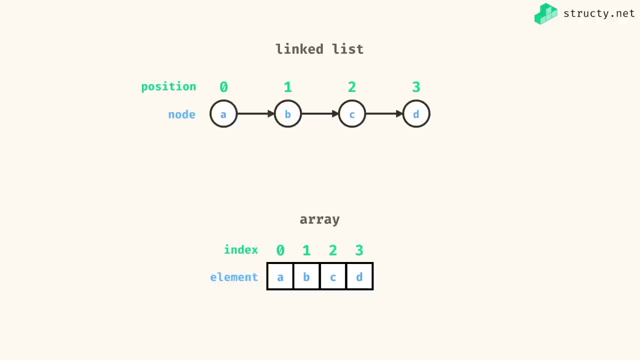 that means all of your elements in an array are going to be stored like right next to each other in your computer's memory, And that has a lot of consequences in the runtime of different operations across your array, right? So let's say, right now I wanted to step through a scenario. 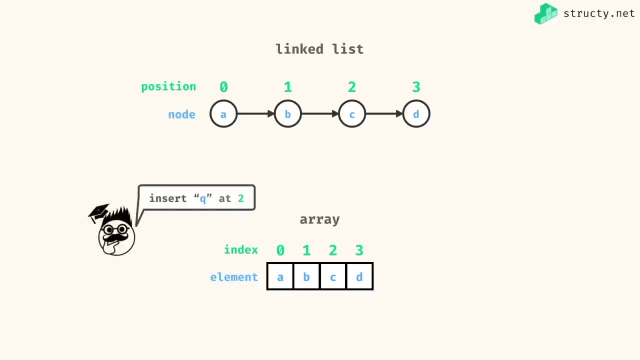 let's say I have the goal of inserting a new element, q, at index two of my array And the key specification here is: I want to insert q at position two. I don't want to overwrite the current element at position two, right. So at the start of this operation I have four elements in my array, ABCD. 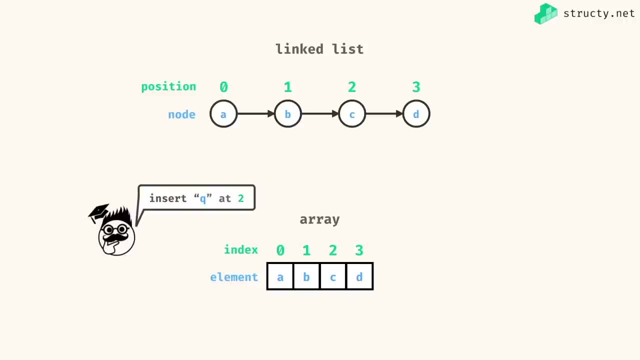 After I do my insertion of q, I should have five elements in my array and they should go a, B, Q, CD, right, because I'm inserting some new element at index two. So how would this algorithm work? Well, let's say I have a new element at index two of my array and I want to 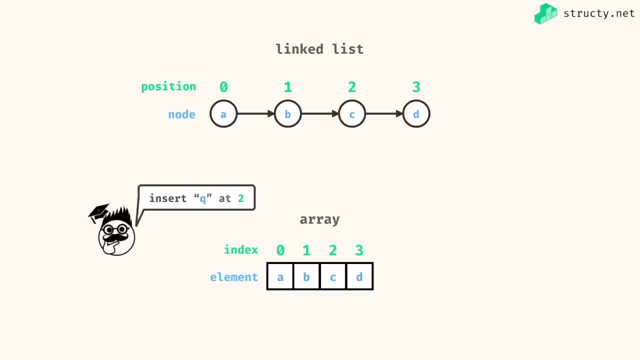 run at a high level in an array. Well, typically, all you need to do is obviously find the index two, which is right here, And I know that this is where I need to put the new q element. But I can't just overwrite this value of C, because I want to do an insertion, not an overwrite. 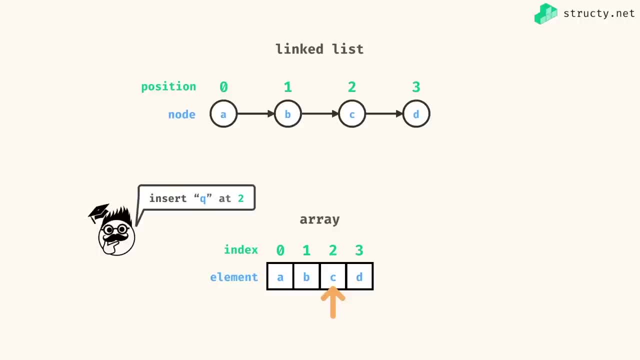 And so what happens under the hood in your programming language when you perform this insertion operation? Well, we hope that there's still some empty space in the array and it should occur after D, right? Assuming that there's still space in this array, I would need to shift all of 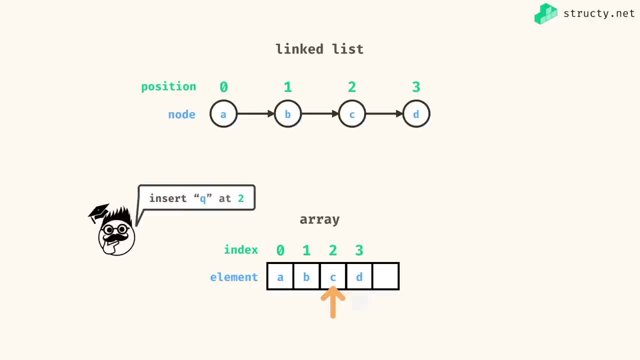 the elements to the right over by one index. In other words, I need to put D to the right, I need to put C over one position to the right And now I have perfect room to add this q at index two Right, And of course, now D would be occupying a new index of four. logically, 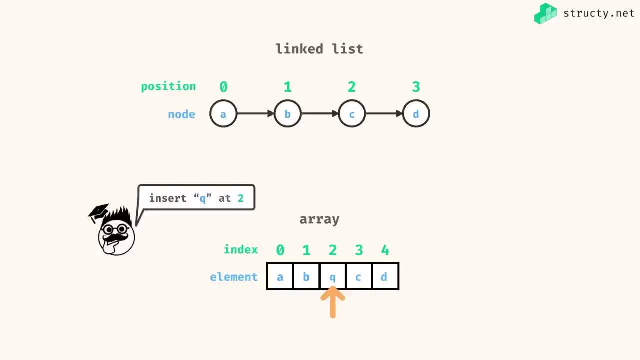 But the important step we took here was to actually insert somewhere in the middle of an array. That could mean that you need to shift over a bunch of different elements in your array, right? so in this very small example I only had to move over two elements of C and D, But let's say you had 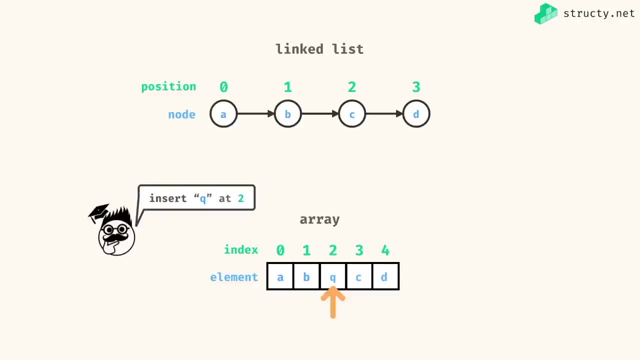 a very long array And there were I don't know 1000 elements after your insertion index. you would have to shift all of them over one by one And that is a relatively costly and slow operation for such a simple move of inserting q right. So we say that when we insert into an array 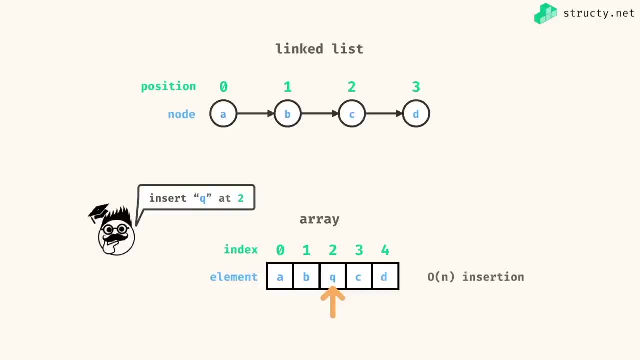 that does have an O of n insertion time. right, In the worst case, if you insert at index zero of an array, that is, you're inserting a very first new element, you would have to shift everything over by One Index in the array. And since there, 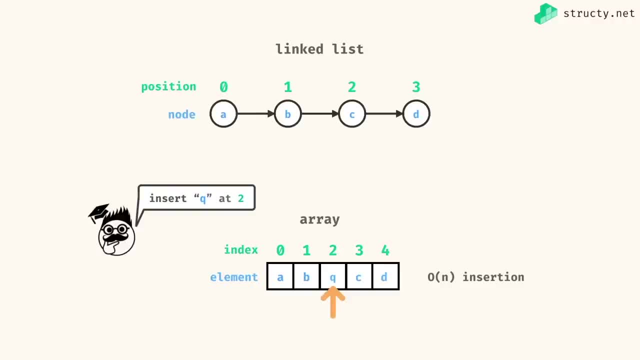 are n elements in the array, you're doing n different shifts- Awesome. Now let's compare that to a similar insertion operation for our linked list. So let's say I still wanted to insert the value of q at position two of my linkless. Well, that means I need to create a. 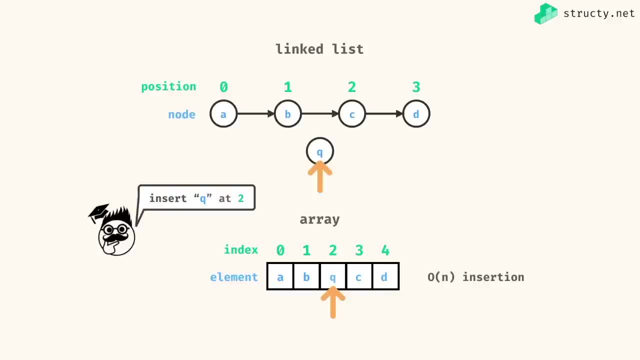 new node in memory, And what's great about a linked list is it is not required that the nodes are contiguous in memory. In other words, we can have these, like nodes exist anywhere in the space of our computers, a memory addressing, And that's kind of a very low level statement, But the consequence of this is I don't need to do any. 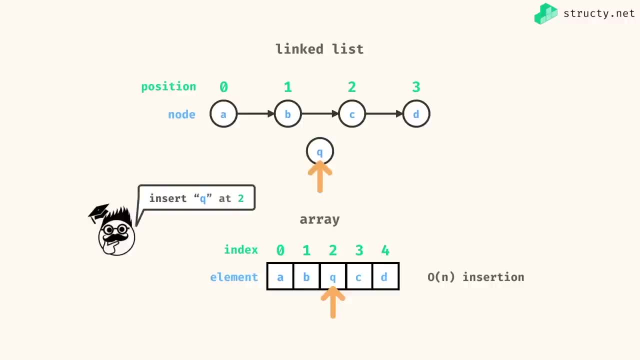 shifting when I perform this insertion. In other words, how does that work? Well, if I want Q to become position two of my link lists, now that I've created the new Q node, I just need to adjust B's next pointer. So I'm going to look at node B and reset its next pointer to point at Q. 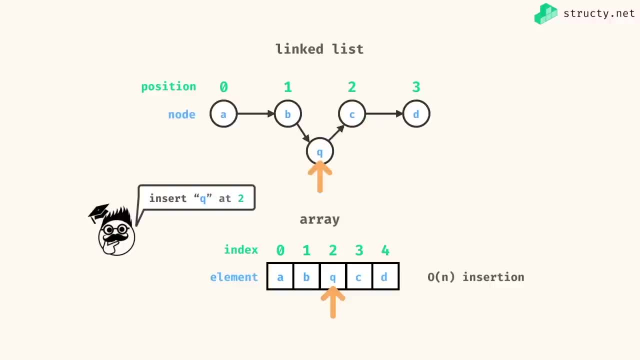 then I set Q's next pointer to point at C, And with those small changes I've actually changed the logical order of nodes within my link list. it would now be this right: Q occupies position to, C occupies position three, and so on. And what's really great about? 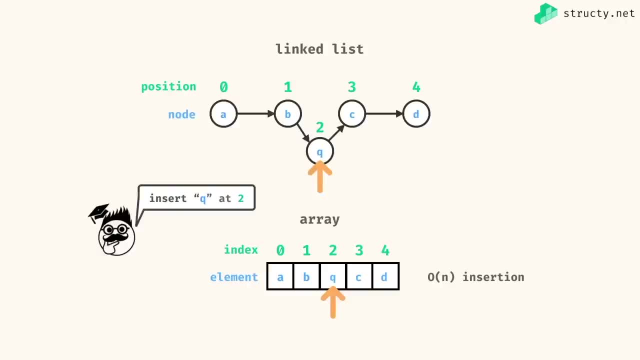 this is, let's say that there were many nodes after my insertion position. let's say there were a third of nodes. let's say there were a third of nodes after my insertion position- 1000 nodes- but I wouldn't have to actually modify all 1000 nodes that came after my insertion. 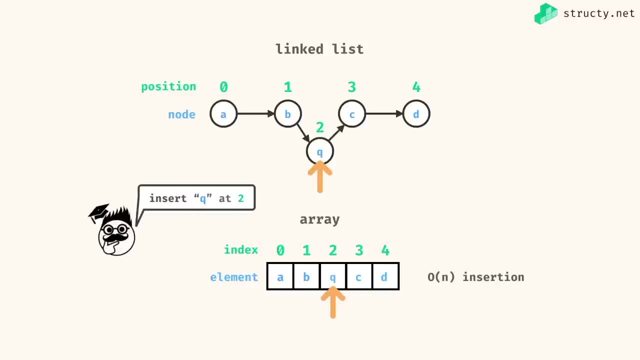 point. I just need to change about two pointers every single time. And because that's a constant number of operations, I will say that a linkless insertion, if we write it correctly, will be constant O of one time. So here we see a very tangible difference between our linkless data. 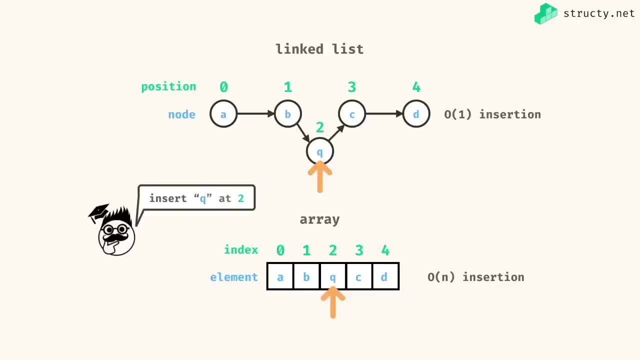 structure and our array data structure, And there are many more different pros and cons between these two, But for now we'll leave it at that And we can chat more about them as we go throughout the course. I'm sure it's going to come up, But what I want to do for now is talk about the core, core, core. 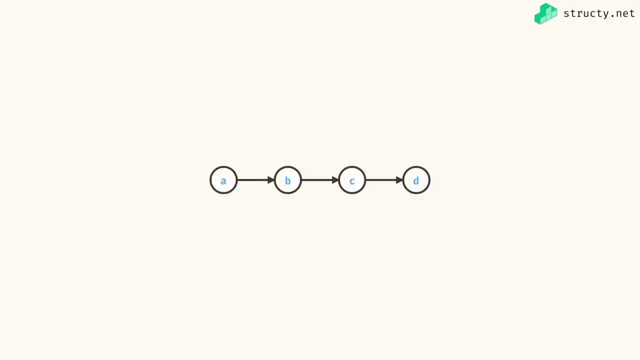 a link list algorithm that's just traversing through a link list. In other words, how can we just touch and process every node within a link list? Well, the important thing to know is, if you wanted to like, give a link list to someone, or, in other words, programmatically pass a link list. 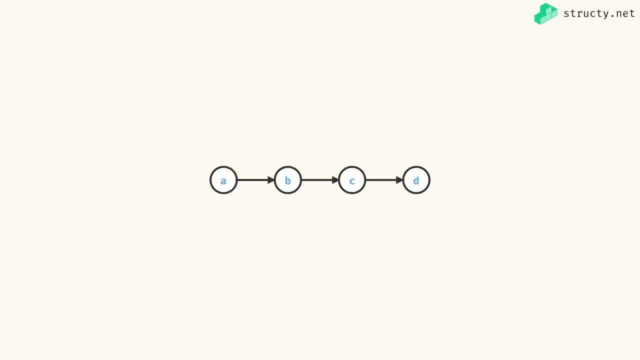 into a function. you really only need to pass a reference to the head node of a link list, Because if I give you the head node of a link list, you're going to have to pass a reference to the head node of a link list. By accessing the next property of every node, you could have access to the full. 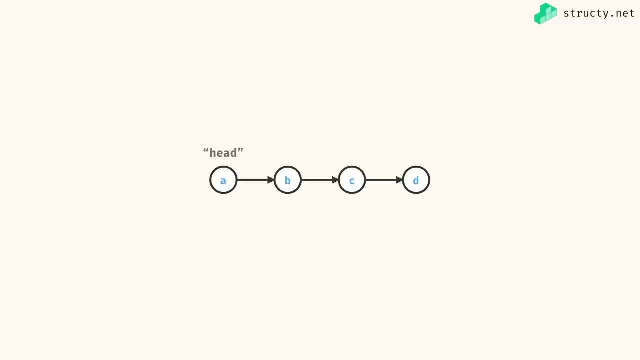 sequential list, right, And so to actually implement a traversal algorithm on a link list, we just need a handful of variables. Most importantly, we need, like a current variable, a current reference to look at the current node of the link list. we're iterating. 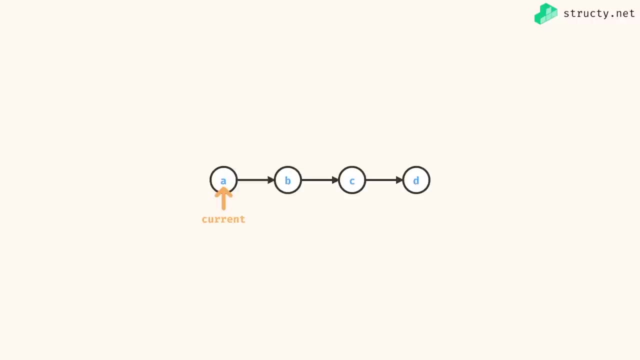 through right. So if I have this current node of a and I wanted to go to the next node, I can just look at current dot, next right or something similar In the programming language of your choice. I can just set current equal to current dot next. 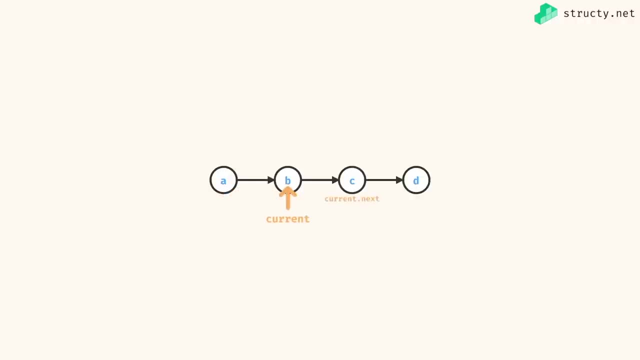 then I would be at the B node, And B also has an x, So I do that again at the C node. I can just keep continuing this process right, assigning current equal to current dot next, until at some point. once I'm at roughly the tail, current would be D, And so current dot next would be this: null. 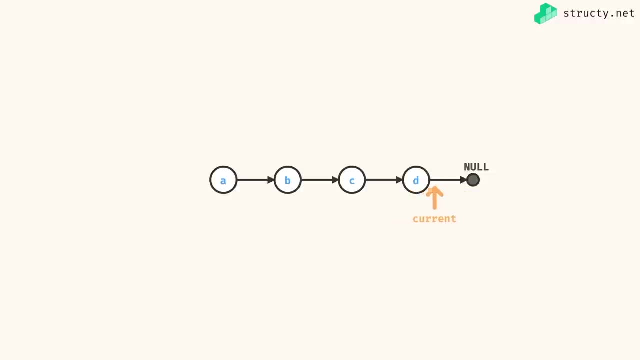 node or this null reference, And if I set current equal to next, I'll be right at null, And that can be a perfect condition I can catch. In other words, we can stop the algorithm when current is equal to null. we know that at that point would have visited every node of the linkless. 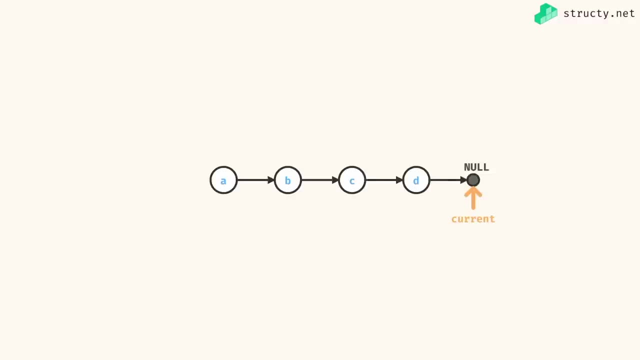 So as I went through this high level trace, I was kind of speaking upon this algorithm as if it was an iterative solution, And I'll also show you how you can solve this one recursively. it's really the same line of thinking. At this point I would want to actually hop into some code So we can see. 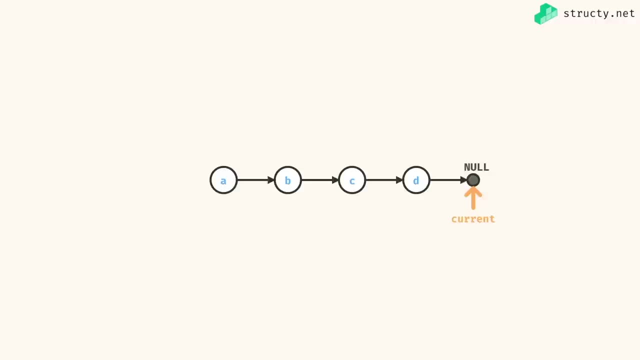 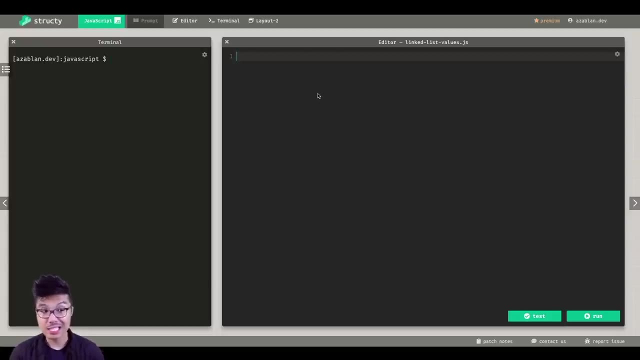 the nuts and bolts: implementation of a link list as well as the core traversal algorithm through a linkless. Alright, do this. So here I am in my text editor. I'm going to be doing this in JavaScript, although you should be able to follow along in your language of choice. So the first thing I want to 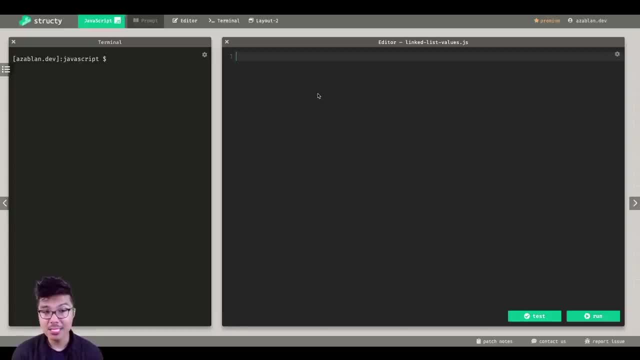 do is just manually build a link list And to start I'm going to need to create a node class, right? So we're going to stay a little bit object oriented here. just create a node class. So for me, JavaScript, I need to give it a constructor And in terms of the properties we're going to need, 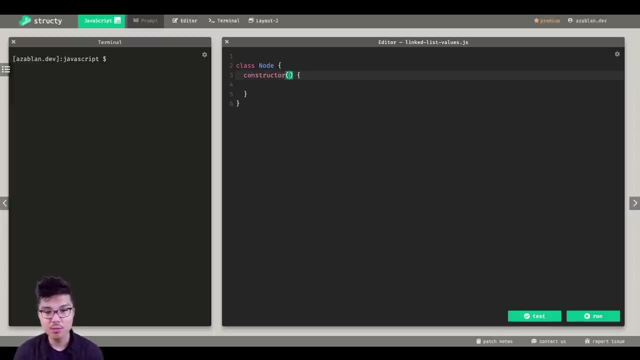 to store inside of an instance of node. I only need two things: I need to store the actual value, But I also need to store a reference to the next node in the link list. if there even is a next node, right So to my constructor, I'm just going to take in the value So I can say this: dot val. 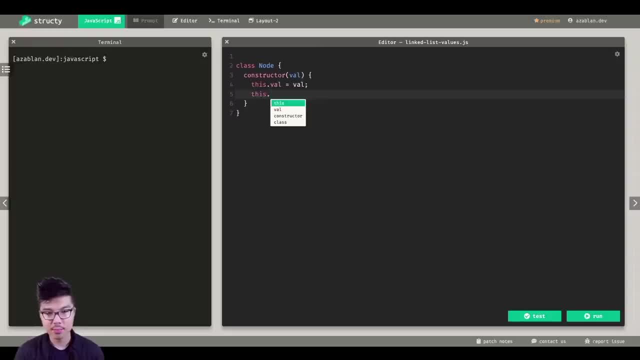 equals Val And I'm just going to always initialize my next to be null right. I can just manually reassign this next property And if you have this class right, and that's all, you need to start creating some link lists, albeit manually. So let's say I want to construct a link list, I'll just 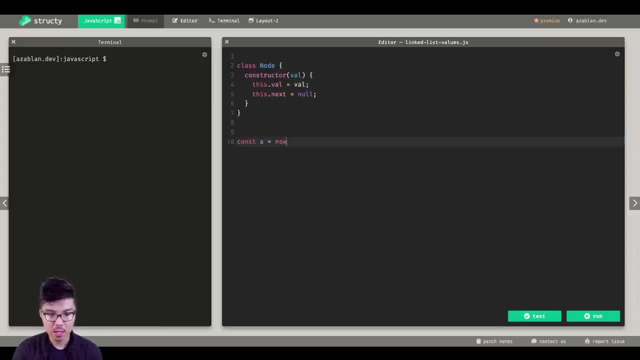 do instances of nodes. I can create node A, make it a new node. I need to pass in the value to be constructed. I'll just give it some characters here, maybe some capital letters this time. So the character a. I'll create a bunch of nodes like this, So I'll have my B, my C and my D. 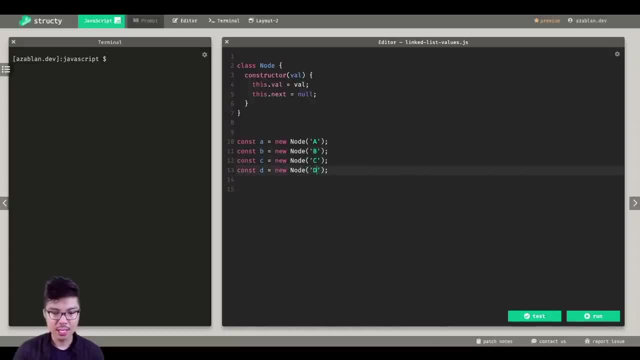 I'll give them some corresponding values. Naturally, I'm storing strings or characters within the values of my link lists, But you can make them. you know numbers. if you want, it's no big deal. But I want to do now is actually: 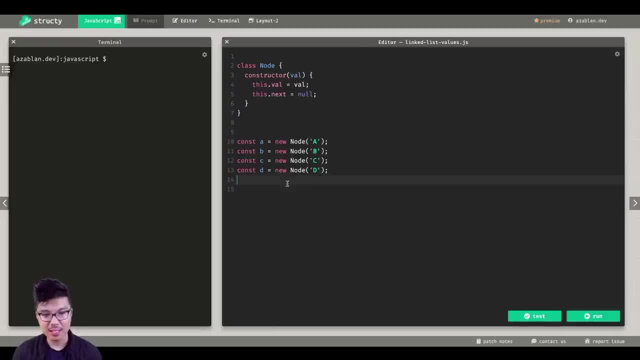 link these nodes together. that way I can just have a link list. I can start writing a few algorithms on right. So typically this part would be kind of taking care for you. already If you're on an interview, you can assume that you're taking in a properly structured. 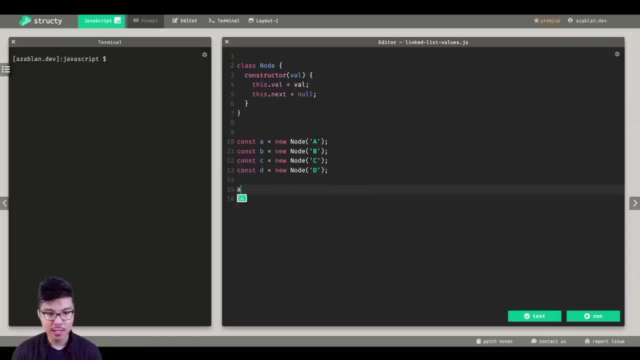 linkless. But if I want to just like test some code for myself, what I can do is say things like A's next is going to be equal to the B node, right? So I'm making A's next property now become the B reference, So I'm actually linking these two nodes together, right? 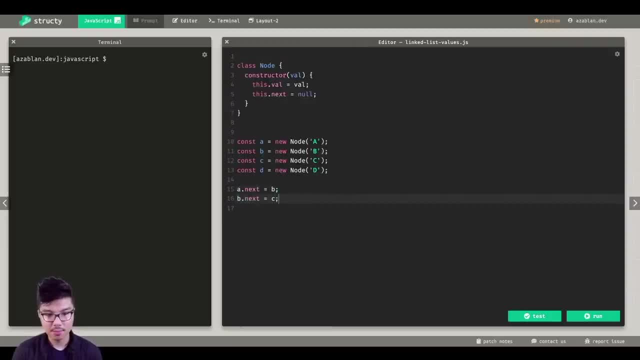 A's next is pointing to be in the same way, B's next is pointing to C, C's next is pointing to D And there is no other nodes in my link list. I'm going to leave D alone because I know automatically D's next would currently be pointing to null, which does represent the tail of my link. 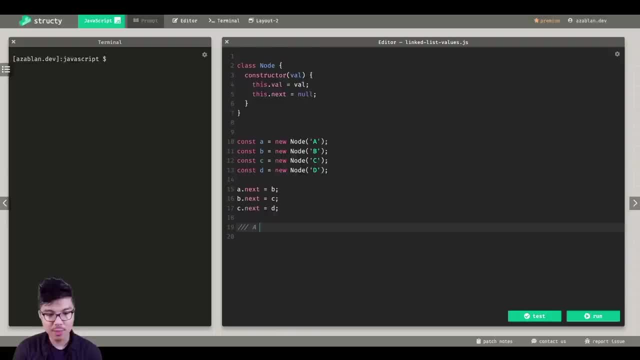 lists. So like visually I think, of this sort of structure. I have A is my head, that points to B, which points to C, which points to D and technically D points to like null. So I'll be explicit here and just draw. 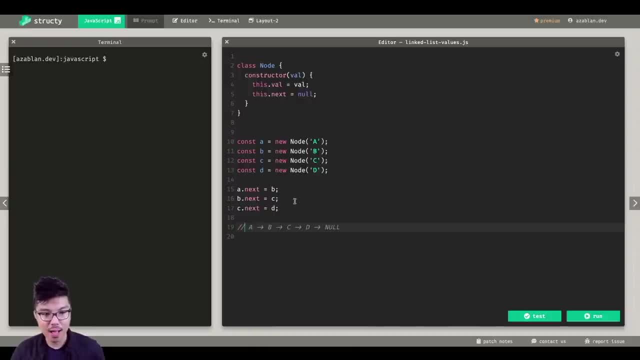 That one out Nice. So now that I have my link list ready to go, let's go ahead and write our traversal algorithm on it. That is, I just want to iterate through every node of the linkless and maybe just print out the value- something very, very foundational here- And so I'll maybe choose. 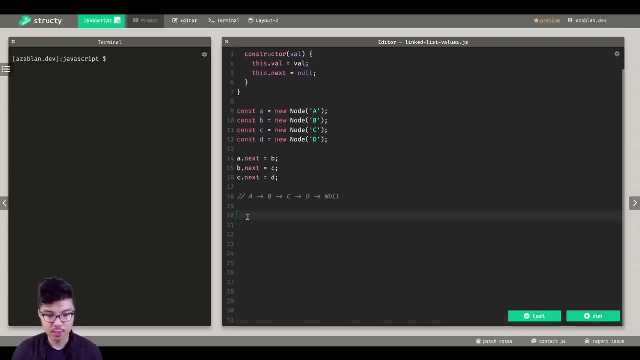 to make this its own function. I think that'd be the best way to go about doing this. So I'll create a nice function here. I'll call it just print linked list And it's going to take in the head of a link list And I'm going to stay kind of abstract here And I just like to call it head. 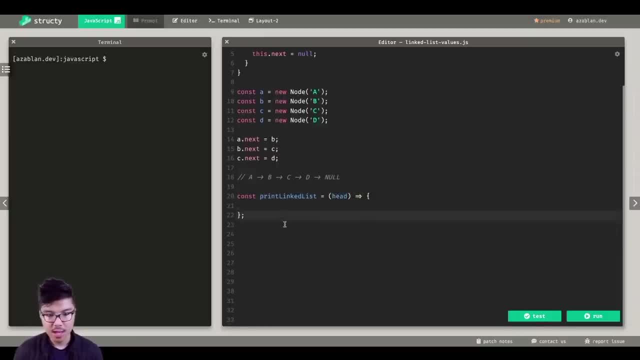 right, There's my nice empty function And in terms of how I would actually want to call this function, the client would have to call print link lists and give it like the real head of the link lists, which for me in my little example here is just a reference to the A node Cool. So I'm 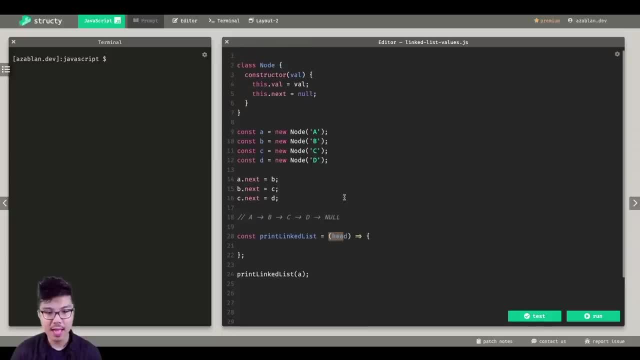 actually receiving the head node, which is an instance of node as the head of my link list here, And so let's go ahead and now set up our algorithm. So we're going to really just implement the algorithm we just traced out on the whiteboard. 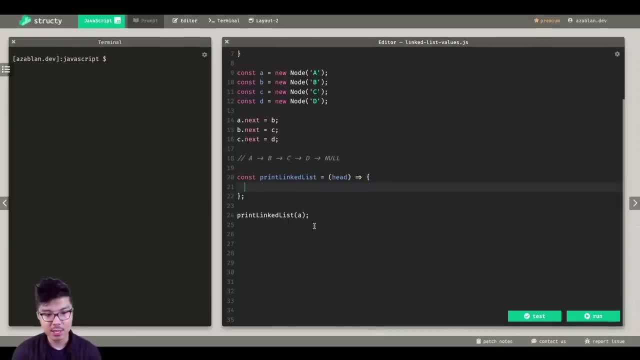 So if I want to just traverse through a linkless and print out every node, I'm going to need to continually update a current pointer. So I'll say current equal to the head of the linkless, which means I'm really starting at the very beginning of my linkless And then from there, how far do I? 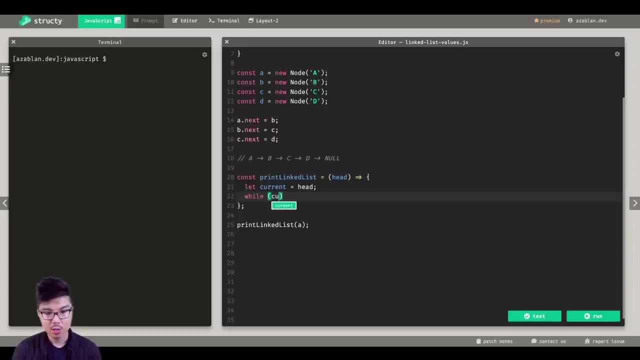 need to go. Well, you want to keep running this algorithm while your current pointer is not equal to null, right is not equal to null. then there's some stuff to still iterate through. Now we get into the meat of the algorithm. If I wanted to like print out or process my current node, I'll just console. 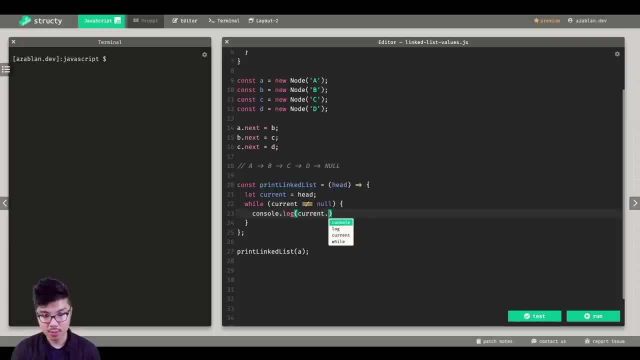 that log here. I'm going to print out this current nodes value, Right And notice: I'm writing all this logic in terms of current because I hope to update current properly at the end of every iteration, right. So now that I printed out currents Val, what I want to do is update what? 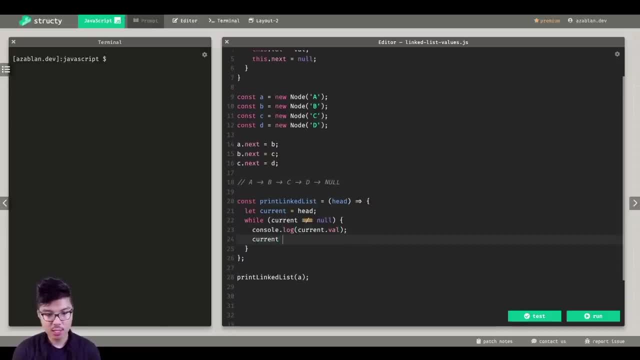 current is pointing to. So what I should do is set current equal to current dot. next, And don't be fooled here. this is a very simple variable assignment. Alright, so let's run this code And then I promise that I'll trace through how this actually operates. It's very short code. 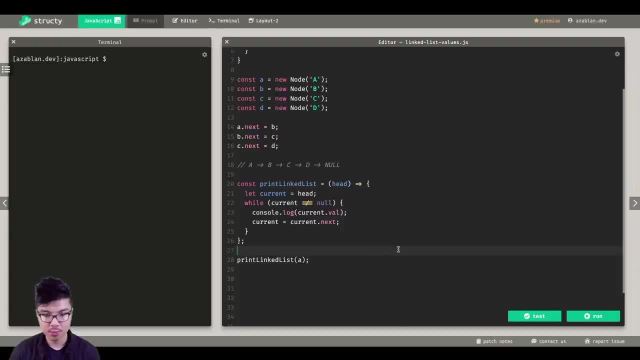 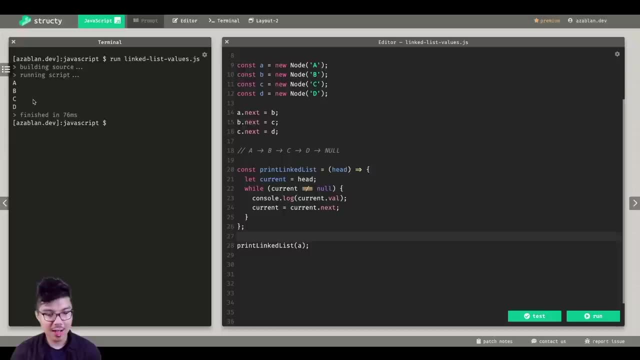 but really the foundation of most linkless algorithms. So let's give that a run over here And I hope, to print out my characters, ABCD, Awesome, And there I have them. So how does this code work? Well, let's try to update and annotate this drawing as we step through. 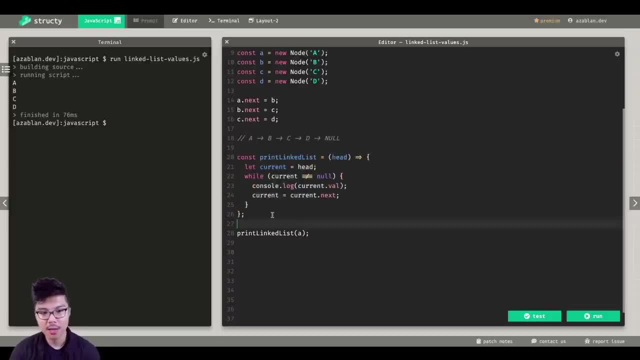 code here, right? So I know that in the context of my function over here I'm really only going to track a really important variable of current And that starts at the head of my linkless, which is passed in as the a node. So technically, give myself some room here. 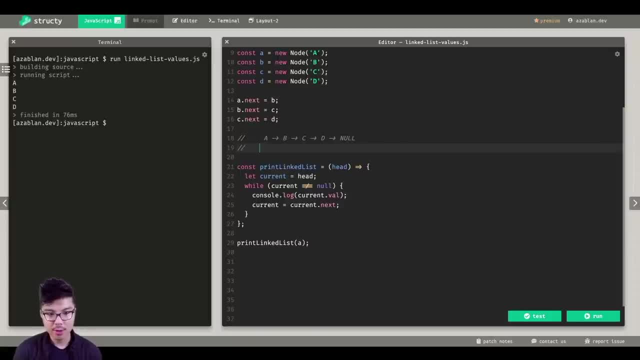 I would say that the current variable starts by referencing the a node, So kind of represent, like that. it's aligned horizontally right, Cool, And what I want to do now is consider my condition. So my condition is checking, all right, while this current variable is. 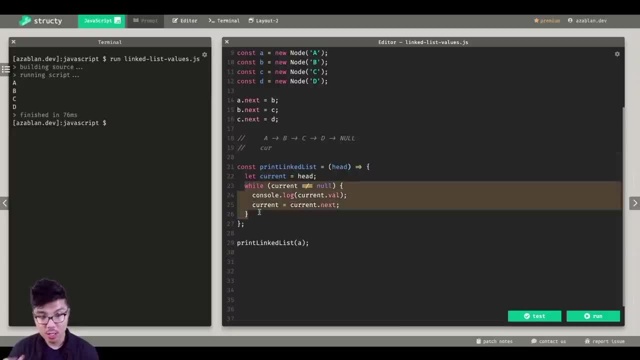 not equal to null, then run the code inside of the while loop. So if I check that on the first iteration that condition is true, right, current is not equal to null, So I can run the code inside, which means I just print out the value of the current node, right. 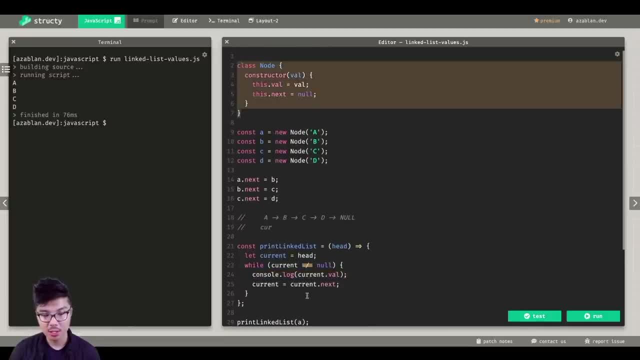 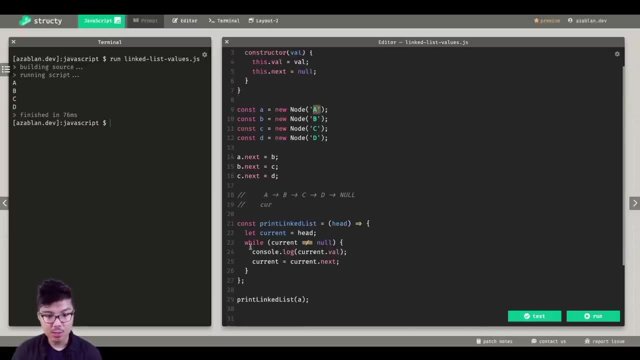 Since current is an instance of node, when I do console log- current dot Val- I would be printing out the a that was initialized inside of it. So that gives you my first iteration. Now here's the important part. Right now I know that current is a, So in this moment that means current dot. next would 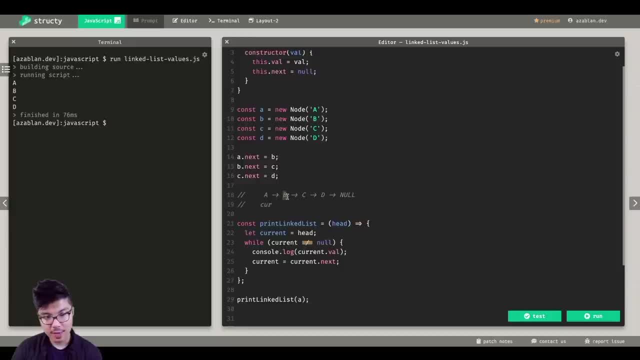 be actually referring to the B node. So if I set the current equal to current dot next, it has the effect of literally moving this over to the B node. Now I can check my condition again: is current, not equal to null. that's true. So I print out my current value of B. 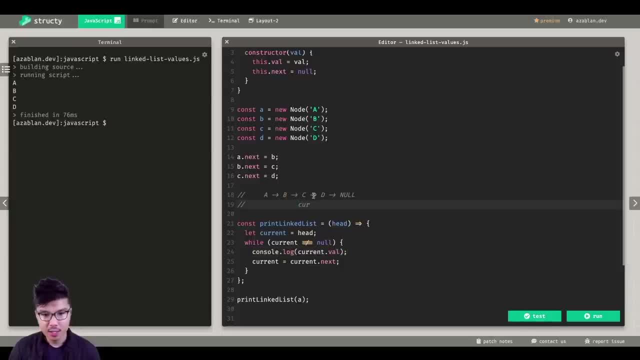 and then go to the next. At this point the process just continues, right? The C node is still not equal to null, So I printed out over here and go to the next node of D. And this is still true, right? 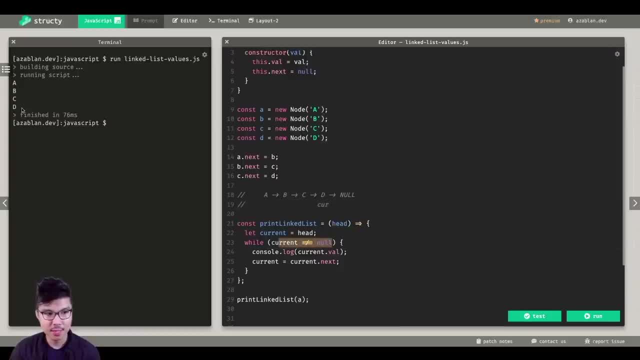 D is not equal to the null, And so I print out D And I actually proceed. another iteration right. So right now, current is the current dot, next is null. So this would literally happen. I set my current equal to null. But things work out great here, Because when I 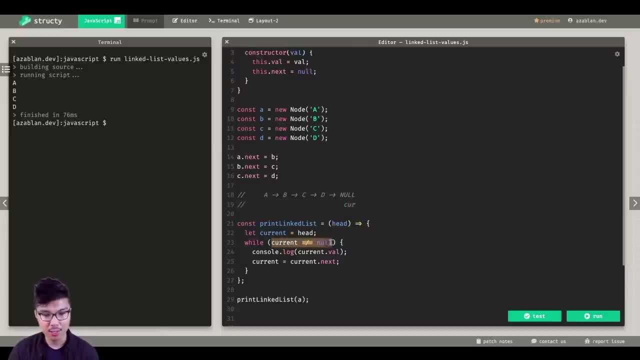 check. this condition I'm going to check is current not equal to null. In other words, is null not equal to null And that's false. So I exit my y loop Right And that's how I'm able to print out every node of my link list: right, ABCD. 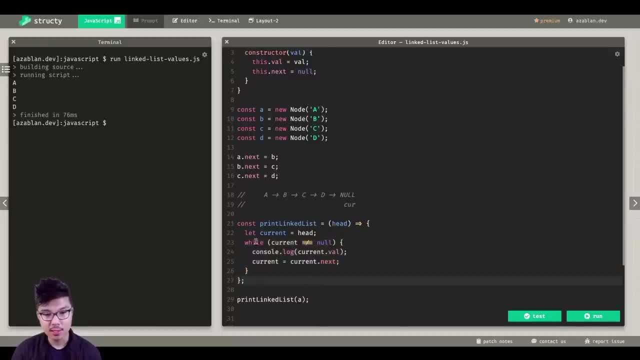 So I think something to draw your attention to right now is how we write this condition. I think the best way and the most robust way to write this code is to check while current is not equal to null. The most common mistake I see people make is: they know, like generally, 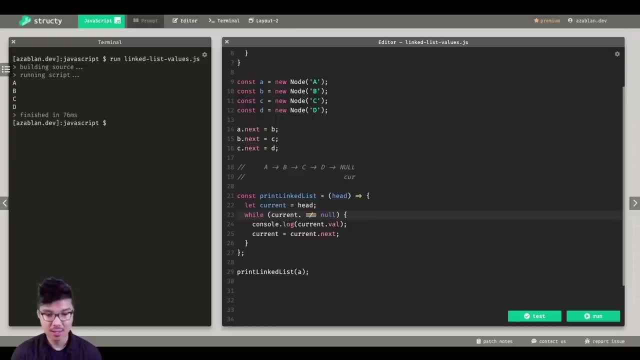 that your condition should be about like roughly the tail of your link list, And so they might try to say, well, current dot next is not equal to null, right. But that would actually cut your iteration short If I ran that. I would only really print out ABC, Right, Because when I'm at the D node, right, I would be. 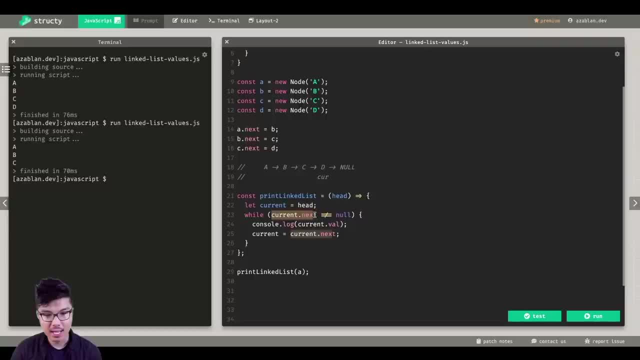 checking All right, before I even print out D. what's these next? Well, these next is no, so I won't even print out D, which is bad right. So generally, when you try to write your algorithms, especially about linkless, try to write it as like present as possible. 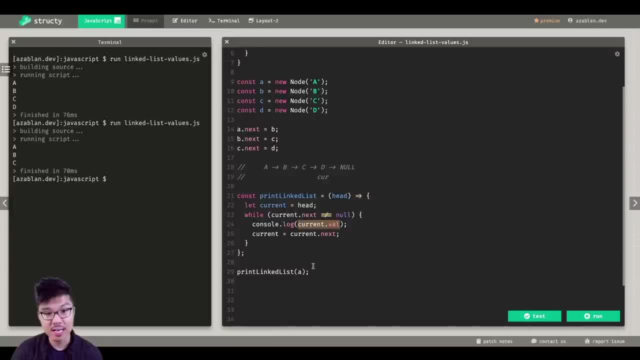 right. So I'm not going to do any premature checking of the next node unless I really really have to. instead, it's better to actually go to the next node and then exit when you actually are at the null pointer right, the null node. So let me return this back to its former glory And we'll just make 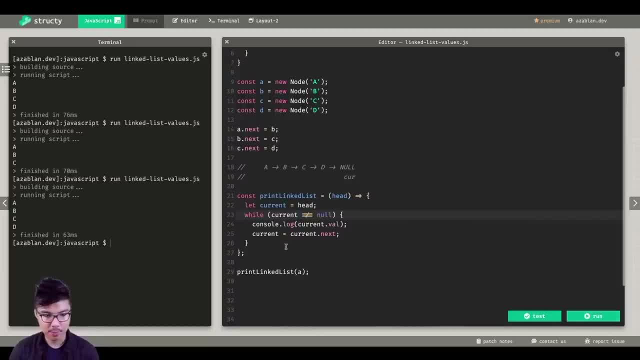 sure that this still works. This our classic implementation of a linkless traversal. it's going to be the baseline code for almost all of your linkless algorithms. Let's take this a step further And I'll show you how you could write the same logic, but recursively. 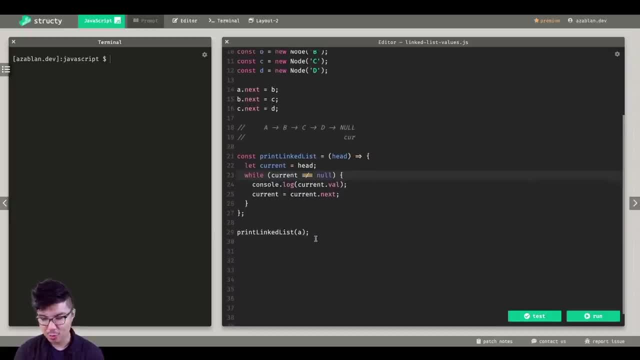 It's really the same logic. you just turn it into a recursive call and a base case, right. So let's go ahead and do this one together as well, And I promise in the next section I'll give you a nice problem to work through. And so if I want to frame this one recursively, 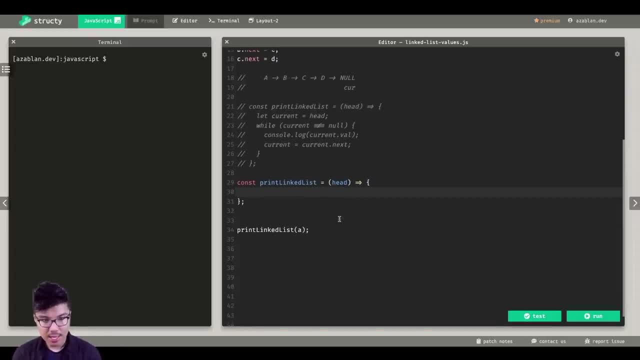 what do I need to do? Well, I like to start with my base case. your base case should basically be an analogy for, like the condition you wrote inside of your while loop. In other words, when are you done with the algorithm? Well, I'm done with the algorithm Once I'm looking. 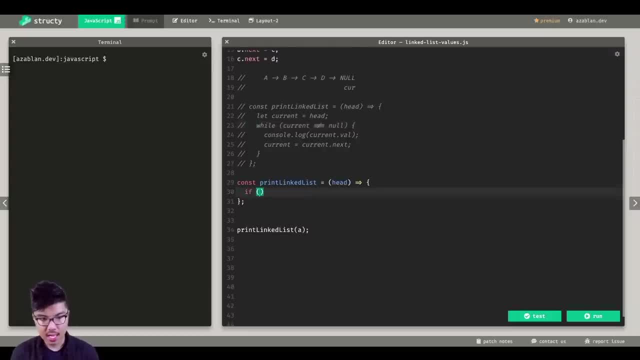 at null right. So I'm going to say: if head equals null, then I'm done, So just return. Notice that here I'm keeping this argument named as head because I think of a linkless as containing many linkless. In other words, a is the head of this linkless. But if I look 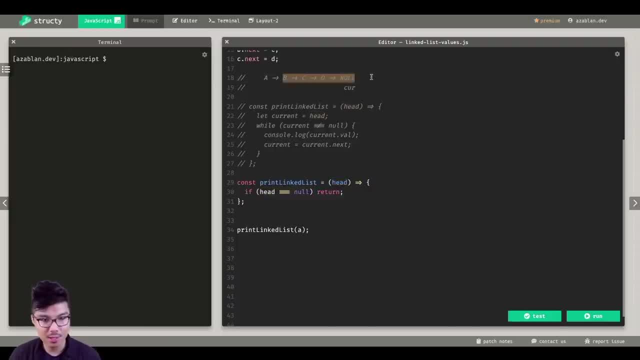 at the sub list inside, B is the head of its own linkless as well right, And C is the head of a smaller linkless still. So I think that's okay terminology to use, For example, for a recursive function. it really shows that you're buying into the recursive nature. 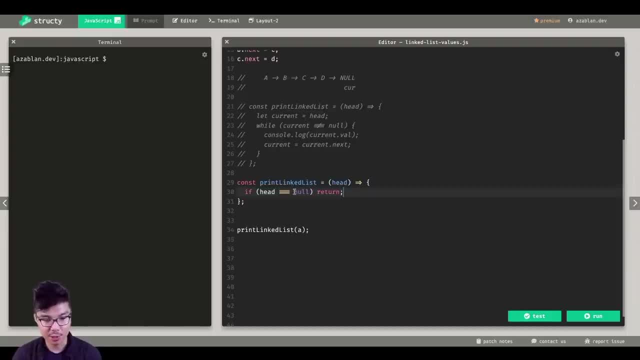 here, right, Awesome. So I'm going to stop running and just return out once my head is looking at null. So that'd be once I'm at this point, right. But in the recursive case, what I want to do is actually process this node. So if my head is not equal to null, right? 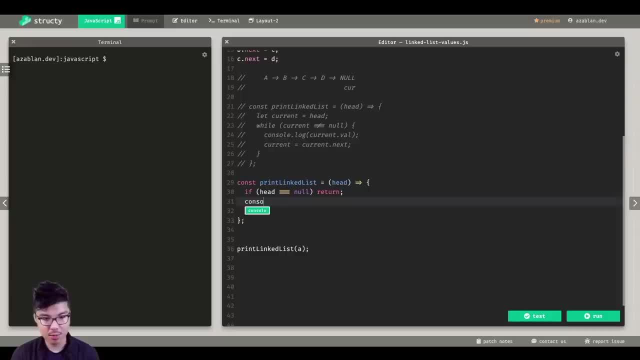 now. then I'm over here, right, What I should do is just print out this nodes value, right? just like I did before. All right, I'm just reframing current is head And if I want to actually progress to the next node, like I did in my iterative, 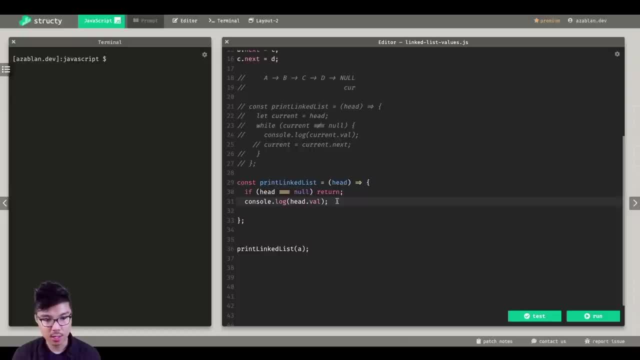 solution. I just do a very proper recursive call here, So I'm going to call: the same function actually makes a recursive. And what should I specify as this argument? Well, I just want to give the next node in the linkless right, so I'm passing in head dot, next Right and 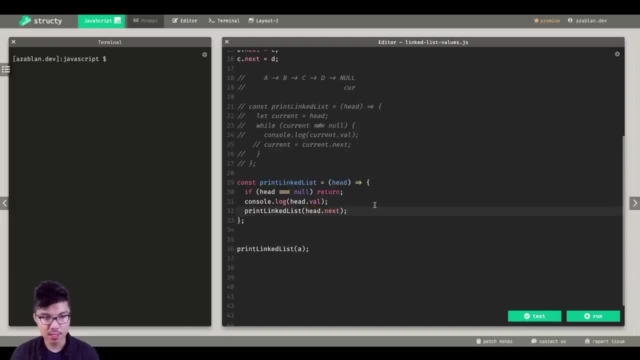 that would be all I need to do for this one. Very, very short and to the point. So let's run this recursive function, then I'll help you trace through it a little bit more. So it's working. The trace looks almost the same, But I think it's good if we do it side. 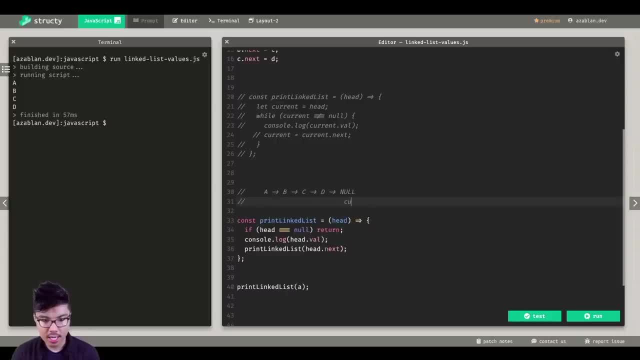 by side with the code over here And really the key argument we need to trace through is the head over here. So on our top level call really passing in the a node as head. So I check my base case here is head equal to null. that's false. So I go into this console. 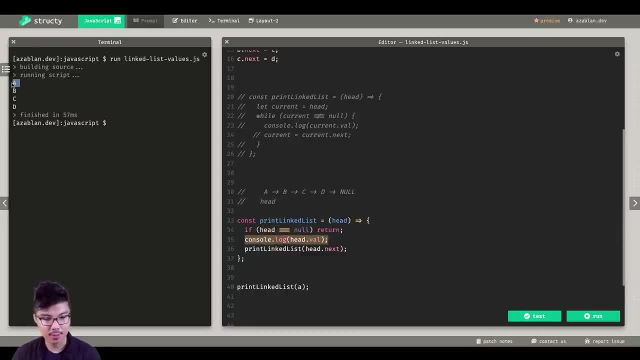 that log, which means I print out the value a awesome. And now I make a recursive call upon the next node in the linkless. So if head is a, then head dot next refers to B. And since I'm making a call to that next node in this next stack frame, head is B and I check the. 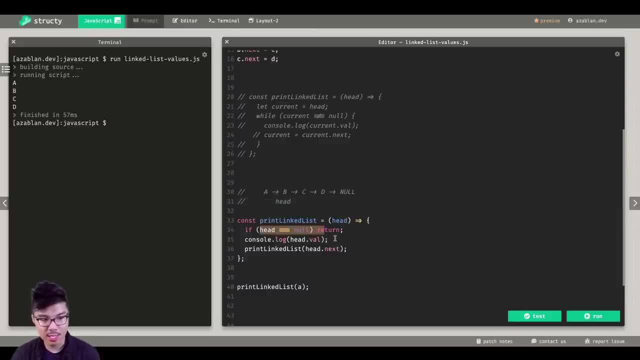 condition again, is B equal to null. that's false. So I just print out B over here and then make another recursive call on B's next, which is C, right. And this process continues all the way down to, let's say, when head is D, right? I check now. this condition is D. 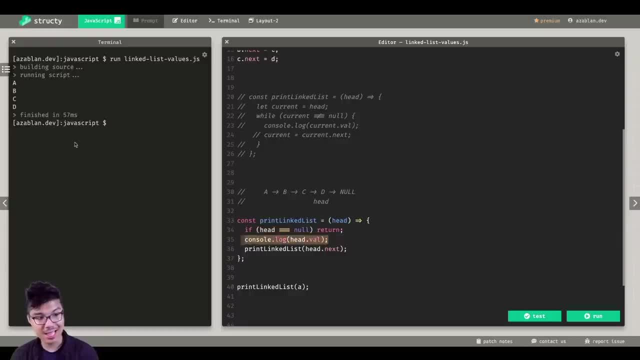 is equal to null. that's false. So I go ahead and print out D, which is like the last logical note in my link lists, And I would make another recursive call upon DS, next right. So if head is D, head next is no, and I would indeed make this call. And now I'm back inside of 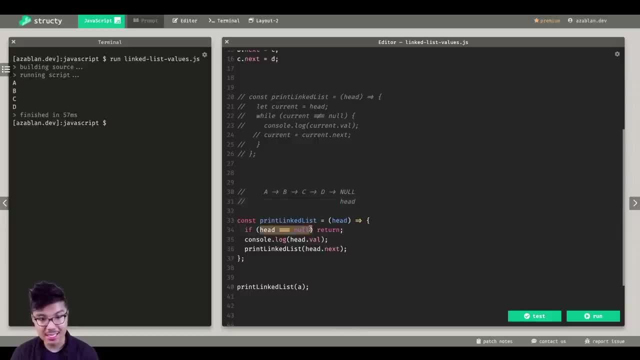 this new call And I check, is head equal to null And that's definitely true right now. So I return. that's my base case And I end my recursion right. This base case is really, really important. So let's compare and contrast These two pieces of code. they really implement the. 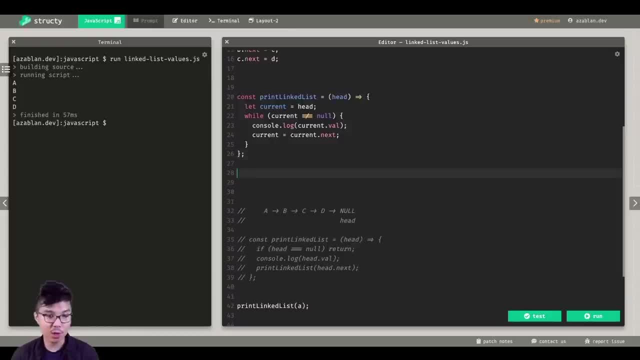 same algorithm And as we go through these linkless problems, sometimes I'll show you both ways to solve it, Depending on you know what style of problem you're solving. you might find the recursive or the iterative a little easier to write over the other, which. 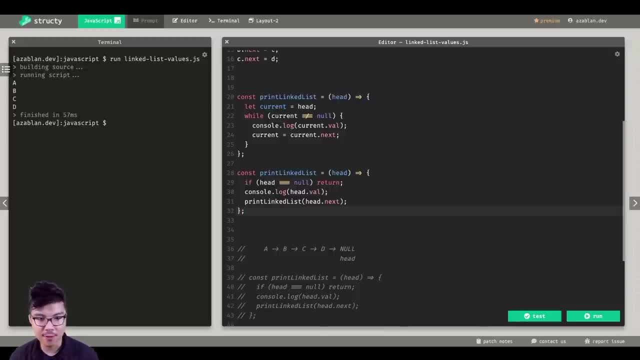 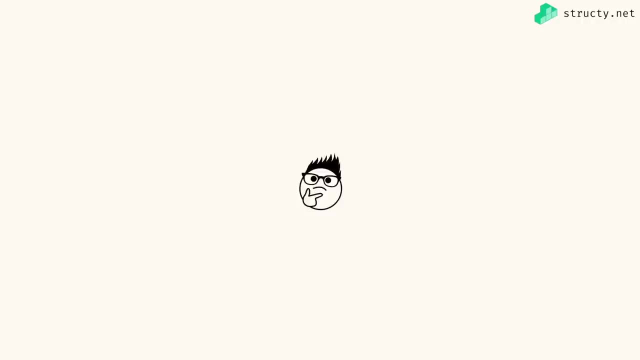 is why I think it's important to practice both. but maybe you know, choose a favorite and decide what you're most comfortable with. But that being said, practice both. Alright, let's head back into the whiteboard. Hey programmers, Alan here right now I want to. 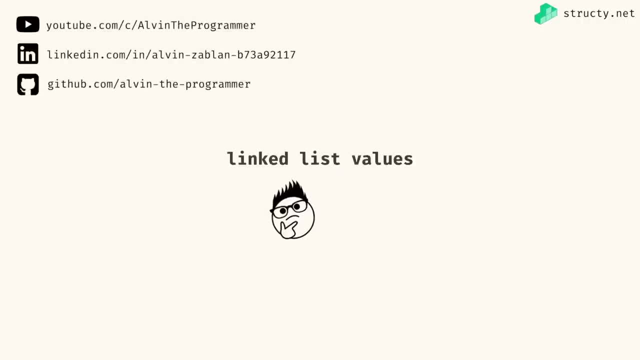 go over a approach for this linkless problem. So hop right in right here, this problem: you're going to be given the head node of a linkless. we want to do is return an array containing all of the values within the nodes of that linkless, and we should do it in order. Bear in mind, in this problem we're given 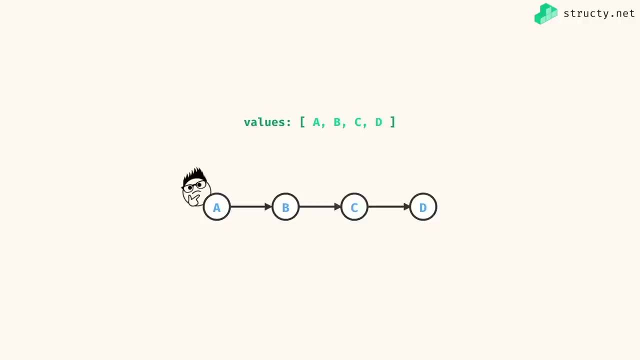 a singly linkless, which means that every node has a pointer to the next node in the linkless. we know that the last node of the link list would have a next pointer that points to null. That being said, how can we go about solving this one? Well, this problems we're. 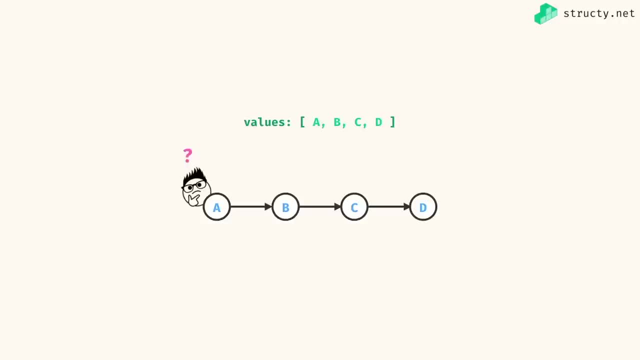 going to have to figure out in order to solve this one right, And so you can either go back and fill in thełauu or, from our experience at x tn, it should just come up. So at this time, we want to try to fill in the baith in order to stitches bind the unneeded nodes. 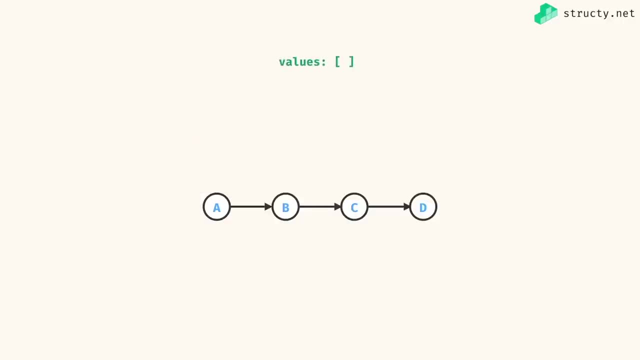 of the node, and lo, let's do that. Let's just say that there is an entry in line And the argument to come in here can be extremely fine. And so, having a포 BRAINE, which is the sum of all the nodes in theких, it means that we're perhaps just going to have to for 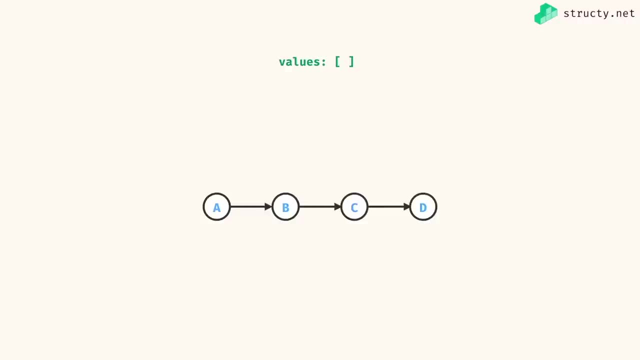 the string to change the number of lines we'll be sending. This is going to graphp Stephan's holders, which is going to be living in here. it's going to say that we can't have all of our nodes in aQuery. We can only have valid in here, and we want to put it to the right. 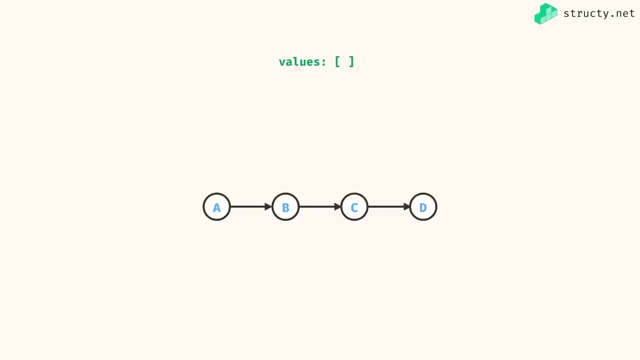 need a variable or just a pointer. We're going to start at the head of the link list, right? Bear in mind that our function only takes in the head, but I know the head is like the ultimate starting point of the link list And eventually I could access everything. 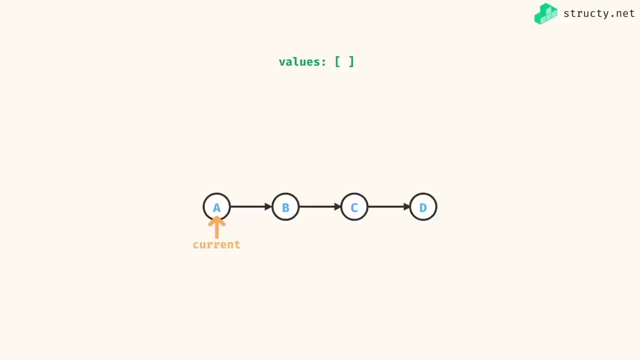 throughout the entire list. So I'm going to set my current equal to the head And what I can do off the bat is just check currents value and add it to my running collection. So I have the a value inside of values. now, And since I have access to the current node, 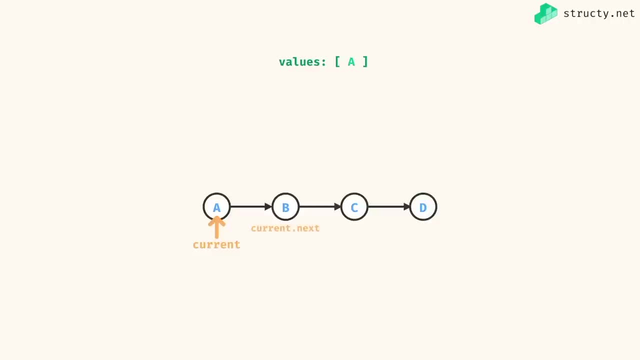 I know that if I access its next property, I would have access to the next node of B, So what I can do is set current equal to current dot next, basically just moving my pointer to the next node. like this Same thing as before, I can add my current value into the. 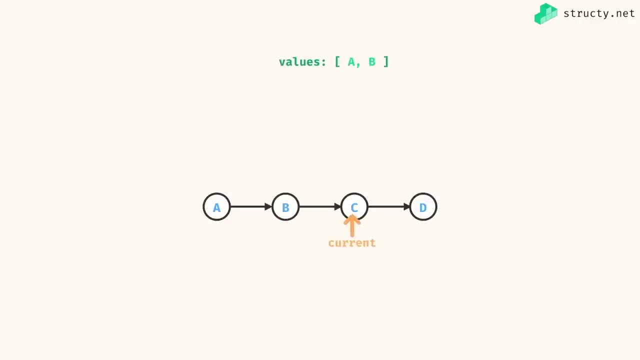 collection. I'll just proceed in this way. right, Same thing for C: set current equal to current. next, And things get interesting once we approach the tail of this link list. So I'm currently at the D node And I go ahead and add that value into my values list And 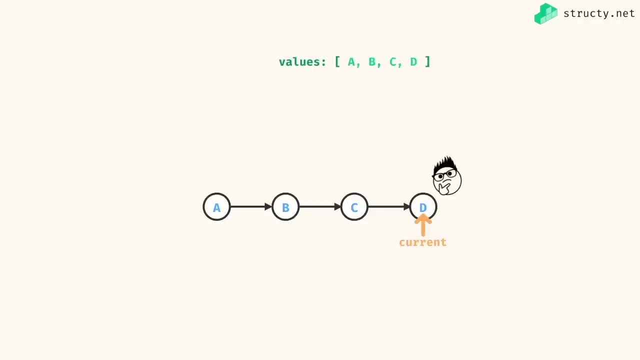 what we'll have to do now is consider the scenario when it's appropriate to actually stop our traversal. Well, bear in mind that these next actually points to null, So maybe I'll draw that explicitly just for this drawing. So these next is just pointing to null, which? 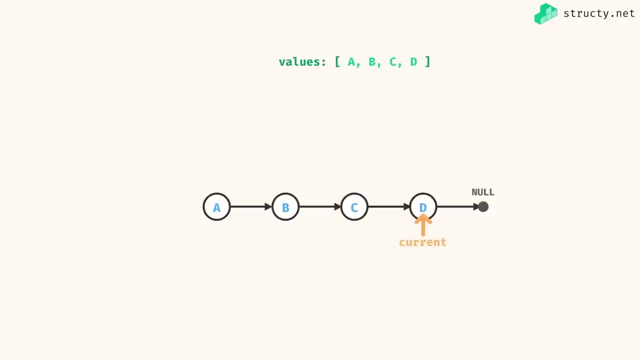 means if I continue this algorithm in the general sense. so I set current equal to current. next, that means my current pointer now points to null, And I think that would be a perfect stopping condition, right? So once current is no, we know that we've hit the end of our. 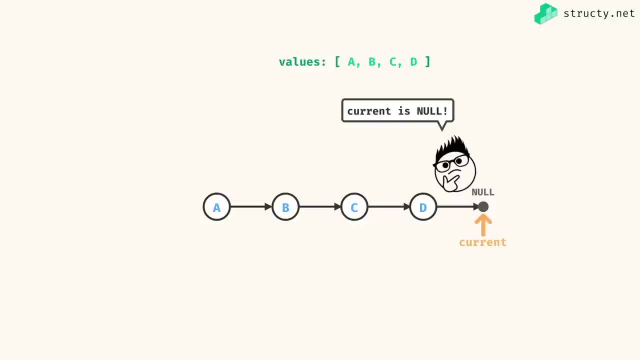 link list. So we're totally done, And if you look at the order of our values, it is indeed the correct order, right? What can we say about the complexity of this algorithm? Well, if we say that n is just the number of nodes in this link list, then the type- complexity. 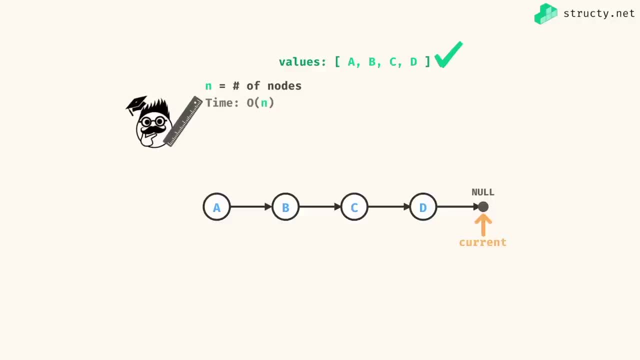 is going to be O of n, right, Because we're just are really iterating through every node once And our space complexity, if we consider the output array, that would just be also linear in the number of nodes over here, And so I'll tell you what this looks like. a pretty 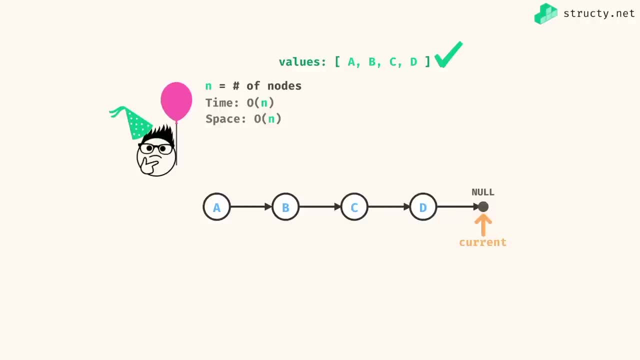 good strategy that we can go ahead and implement. We'll implement it in two ways. First, we'll implement it in two ways. First, I'll show you the iterative version and also show you how to implement this one recursively- Really, both the iterative and the recursive code. 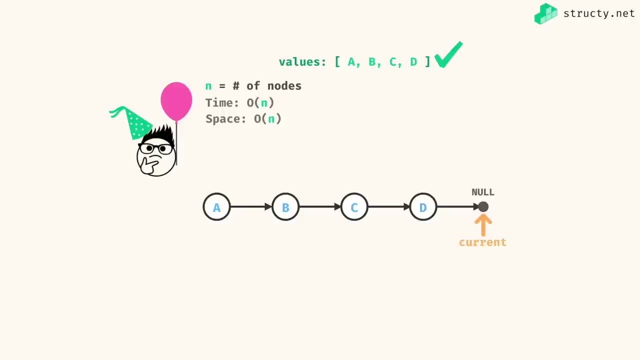 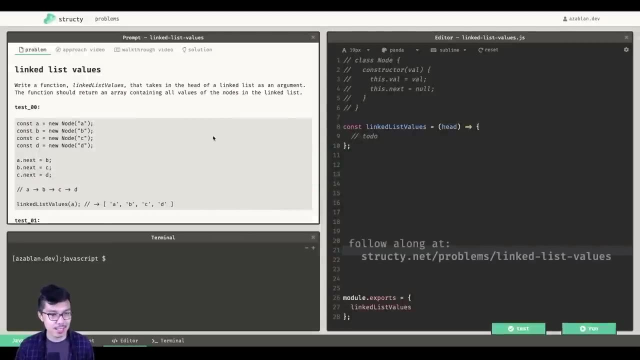 use the same sort of mechanisms, So I'll see you in the walkthrough video. Hey programmers, Alan here right now I want to go over a JavaScript solution for this link list values problem. So we'll jump right in And we'll start by implementing, I think, the iterative version. 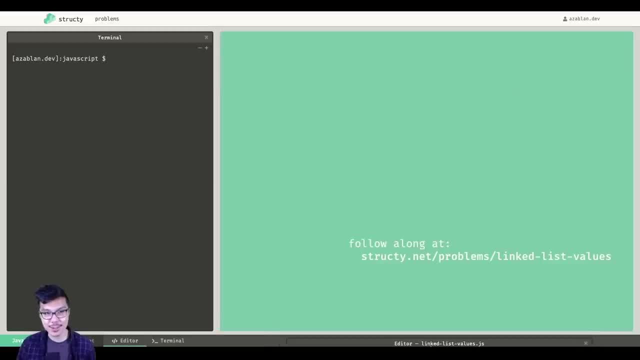 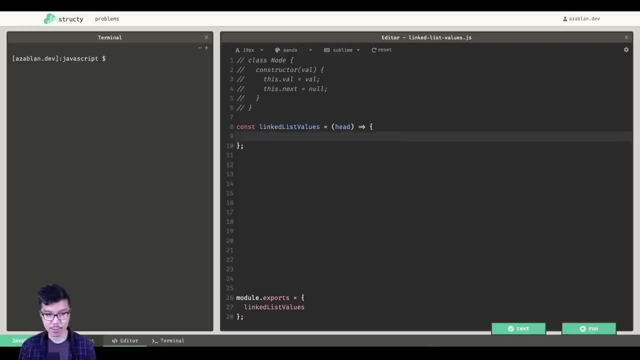 that we spoke about in the approach video. So if you haven't watched the approach video, definitely make sure you check that out First. right, And so I'll get the ball rolling over here. what I want to do is use a pointer. 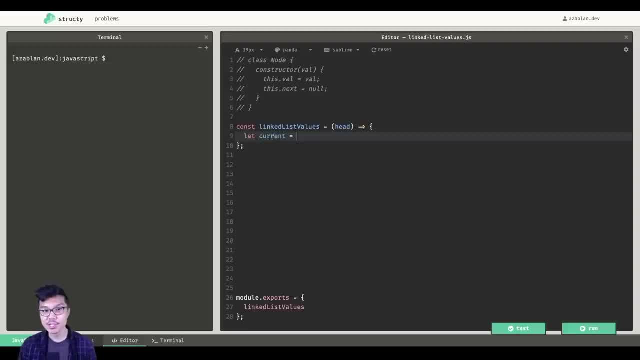 really just a variable for me, right? So I'll say: let current- I'm going to initialize it to- be the head, And I know that the most important pattern I probably need for a linkless is just a traverse in order through a link list, And the way that looks is: I want to keep iterating. 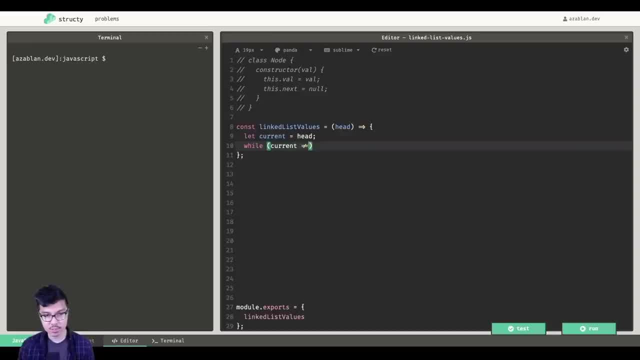 a while. my current is not equal to null, right, so just not equal to null. null would mean the very, very end of my link list. Nice And very standard code I need inside is to progress to the next node of the linkless. 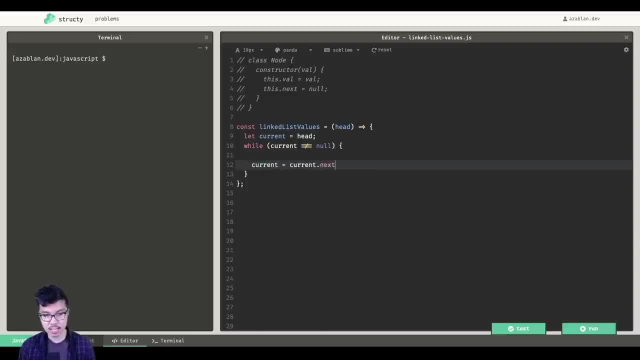 So I said current equal to current dot next. So now I'll think about actually generating the return type For this function. I do want to return an array of all the values, So I should initialize that up top. I'll say let's, or maybe const values goes an empty array. 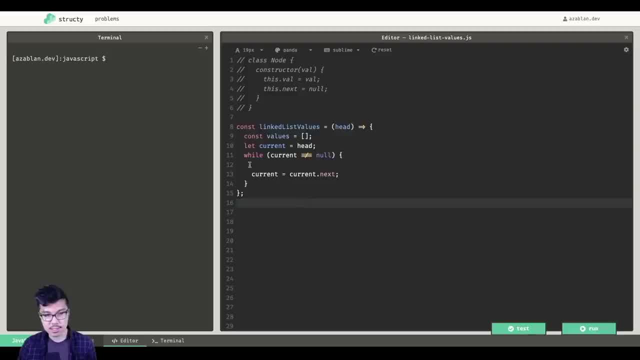 And then, as I actually iterate through all of my nodes of the link lists, at the tippy top of this, while loop nodes value, right, every node has a dot val and also a dot next. So I'll take the current nodes value and just push it into values, right. So values dot, push that single Val And once this: 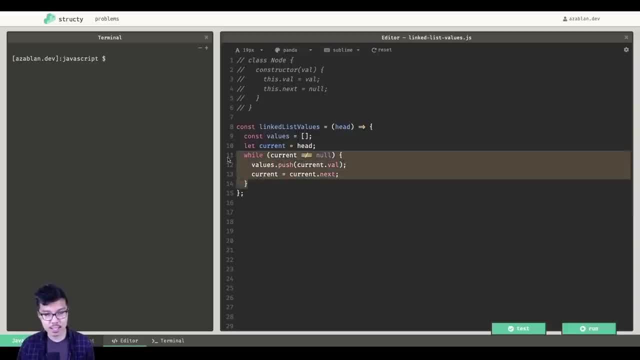 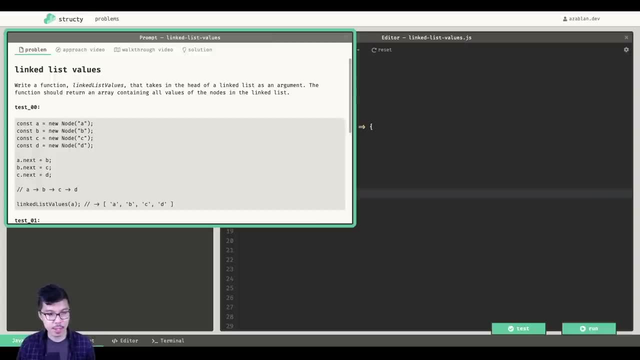 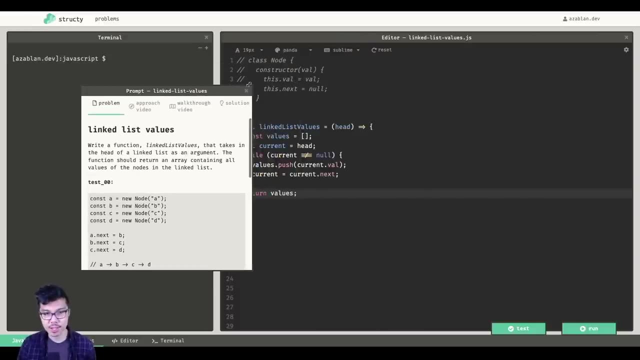 while loop is done running, I must have hit the end of the link list So I can just return the complete values array. So before we run it, one thing I want to always emphasize is, for your link list, a main logic. it's always important that you try to write your logic about just your current. 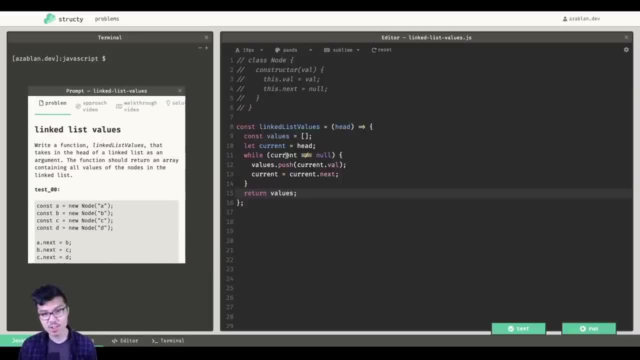 node. So, for example, my condition is saying: while current is not equal to null, it doesn't say like: while current dot next is not equal to null. right, You can probably get away with finessing code like that, But it ends up being more clunky than anything. In other words, whenever I try to 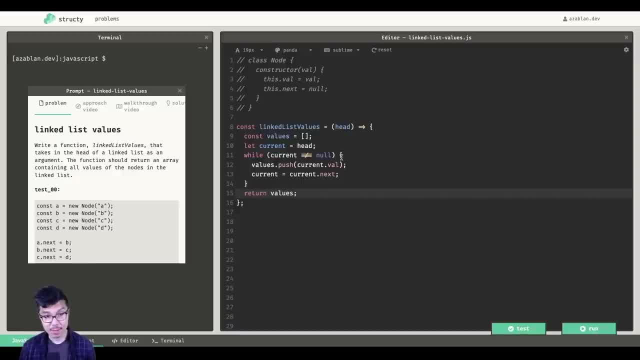 write my logic for a link list. I always try to stay very present, right, So just worry about your current node. So what I don't like to see is patterns like this: right current dot, next dot val and try to just shift your frame. 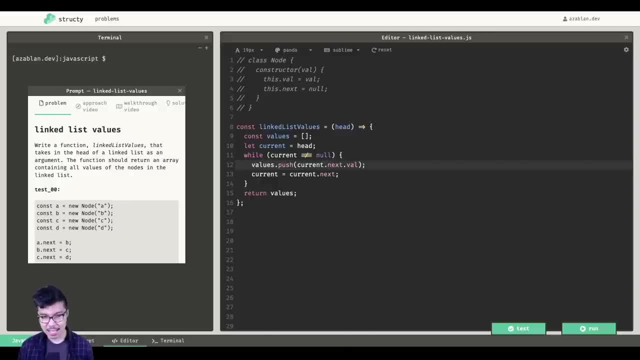 of reference. Because if you do that, then you're actually kind of assuming that your link list has a particular length. So instead I always try to write all of my expressions about simply current right. So while current is not equal to null, then I push current dot val And then I can just 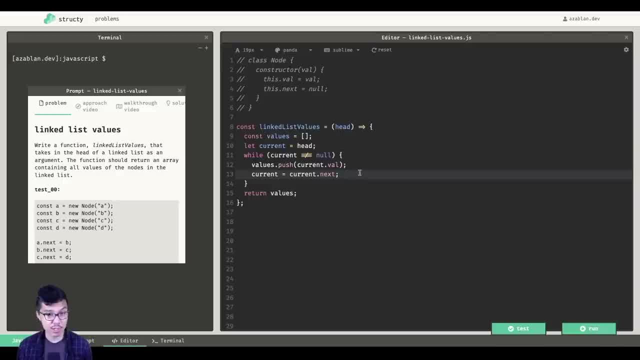 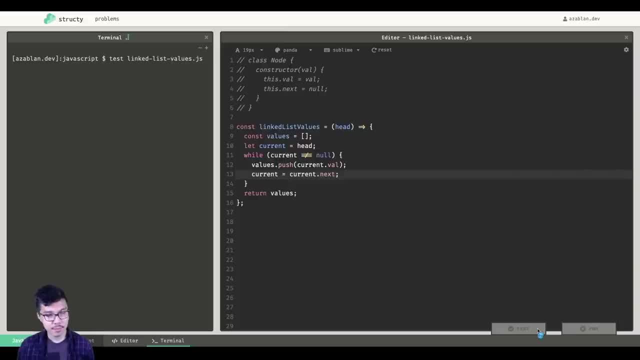 update current to be current dot next, And I can be assured that every node is going to be processed in this algorithm. So let's give this a test run And, if all is well, we can transition into the recursive version. now, Awesome. So how can we do? 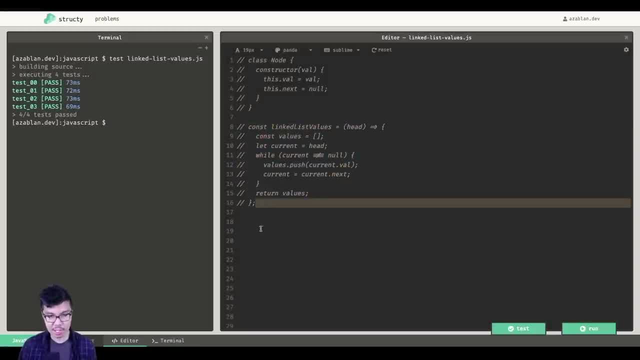 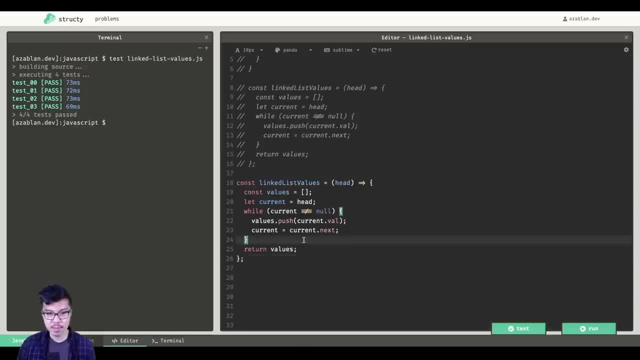 this recursively. I'll just do that down below. So the way I would structure this one- just so I get the most optimal complexity- is really with two functions. So my main function will do almost the same thing. it is going to call a helper function. I'll call this helper function, maybe. 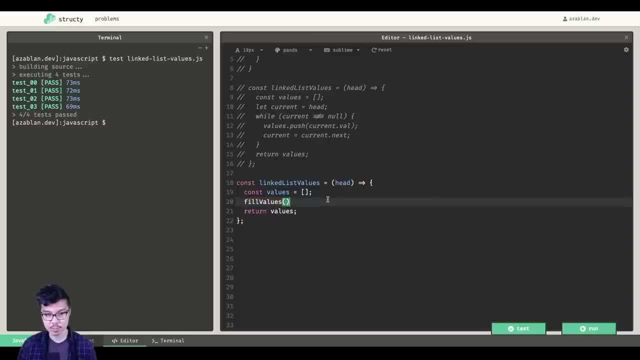 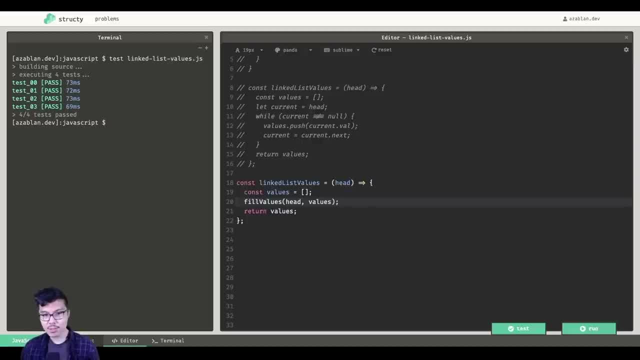 going to do the recursion And also a reference to the values array. So recall that in JavaScript if I pass any non primitive types, so basically things like arrays and objects, they are going to be passed by reference, right. So what I want this fill values function to do is to actually mutate. 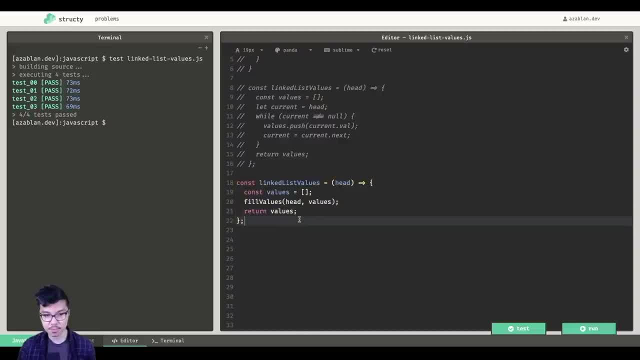 the values array, because this main function is going to return it. So what does that recursive function look like? So we'll say fill values it's gonna take in the head and also the values array. I'll start with the base case here And really what we're trying to do. 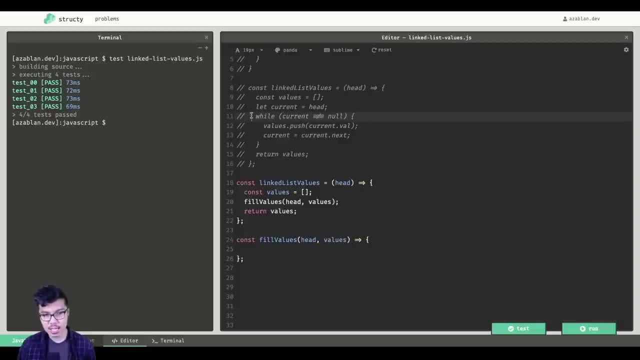 is just translate the same patterns from the iterative code just into their recursive variations, right, And so I know I need to stop my recursion once my head is no right. so I'm going to check. if head is equal to null, then you can stop, So just simply return. 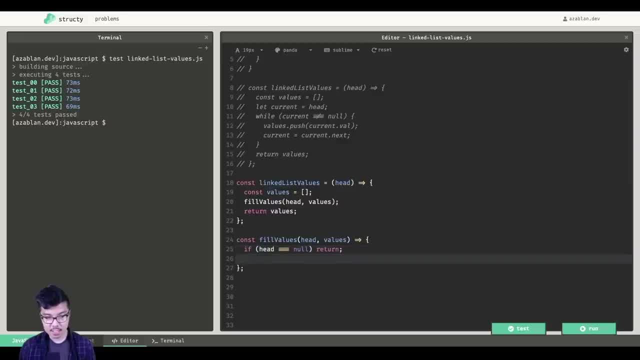 right. really important distinction here is you're going to have a tough time and probably end up with some clunky code if you say if head dot next is no right. So again, I always try to stay very present in all of my code. So don't worry about your next node, just handle. 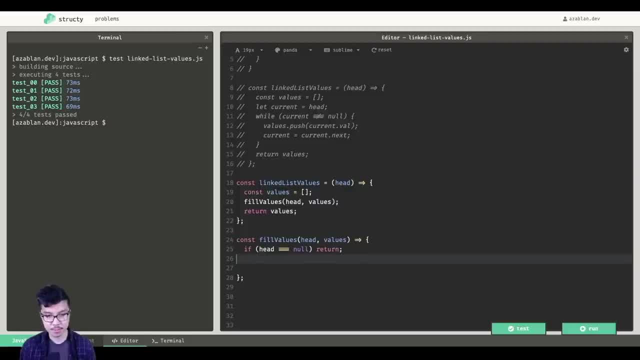 yourself right. Eventually every node will get served here. So if head is null, then nothing much to do, just return and you can stop your recursion. Otherwise I know that head is not null, So it must be a node And I need to take that nodes value and add it to values, right? So I can say: 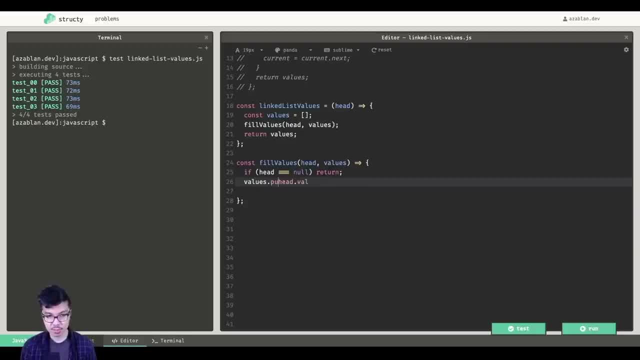 head dot Val and I want to push that into the values collection right. Recall that values is referring to this outer array here. But beyond that, besides this current head, there could be other nodes right in the remainder of the linked list. So I can just call recursively, fill values And instead of pass along. 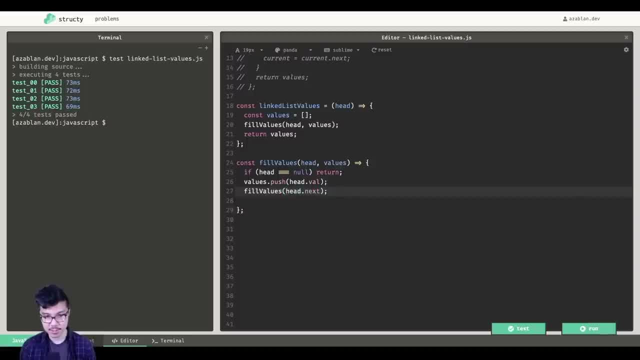 head again. I need to pass along head dot next right And that means in that recursive column kind of jump back around, and now head is referring to the next node and so on, and then its value is going to be added all the way until we get to the very, very last node. Technically, 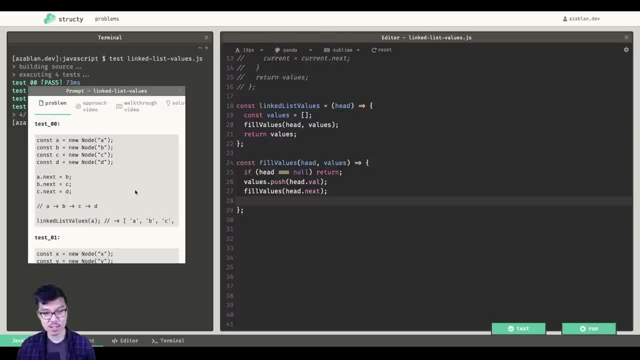 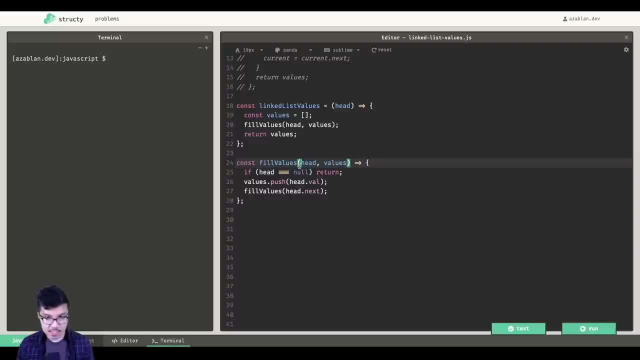 after D, we would hop to these next, which is no, in which case we would exit. due to this base case exactly, And before we run it, just a few issues that I need to fix. I see that missing an equal sign here. 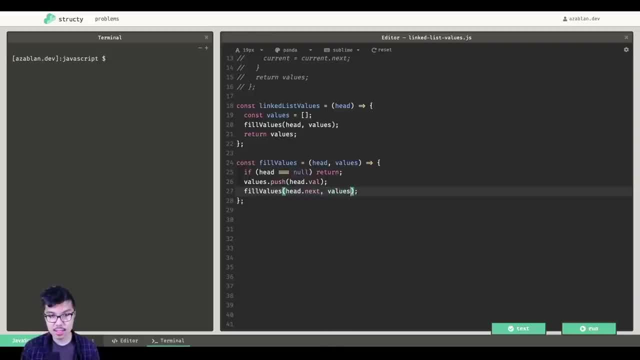 And also when I call fill values, of course we need to pass along the same values array, because I know that every call wants to add its value into the same values array there. So we'll give this a test run. See what we get. Cool, And now you also know how to implement this algorithm. 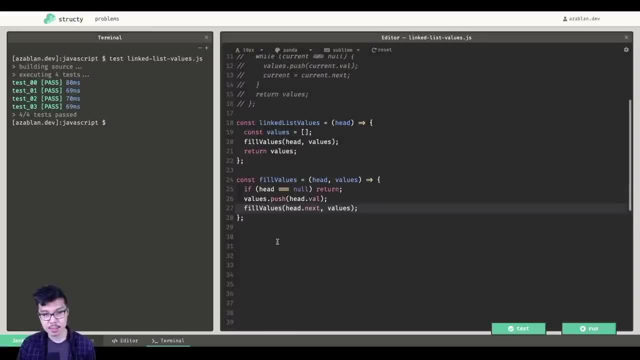 recursively. So the reason I like to split up my recursive version for this algorithm into two functions is so my recursion doesn't actually have to create like multiple arrays, right? Instead, all of these recursive calls are just adding their values to a single array, If I actually 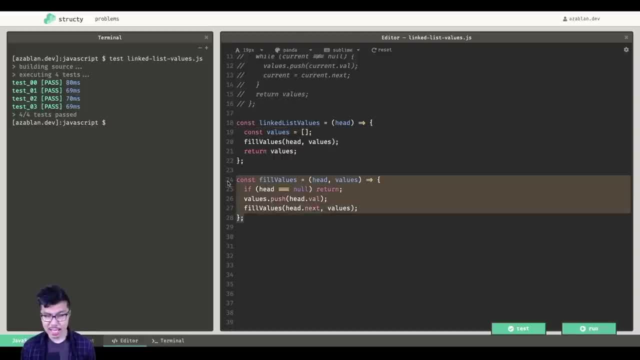 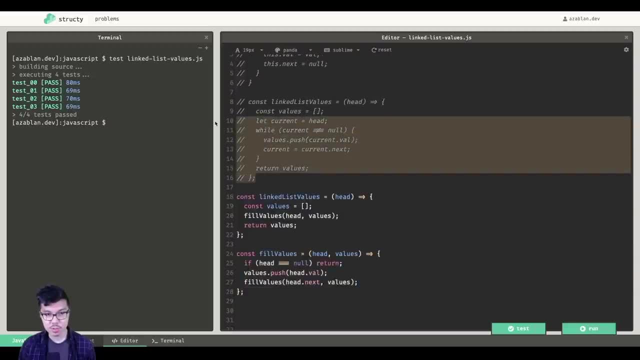 created like copies of arrays all the way through the recursion, I would end up with like an N squared sort of runtime. Cool, So when it comes to comparing these two implementations, they're actually equivalent in terms of their time and space complexity. right Alright. 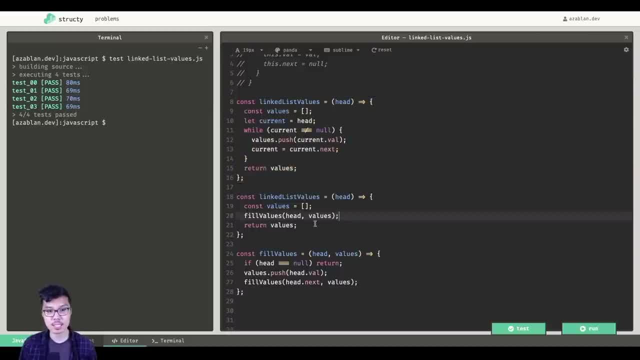 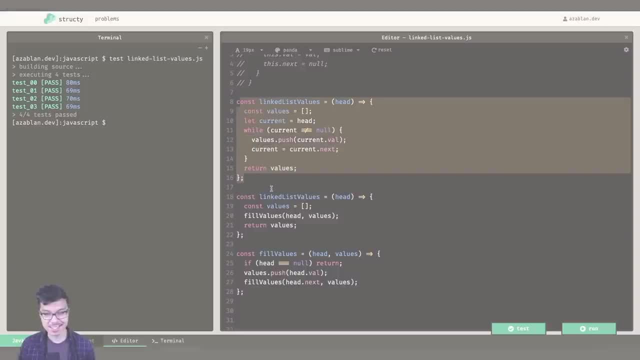 programmers, that's all I got for this JavaScript walkthrough. I want you to practice both the iterative and recursive versions, because they're going to both be a very useful for the next upcoming problems. I'll see you there. Hey programmers, welcome back. right now I want to 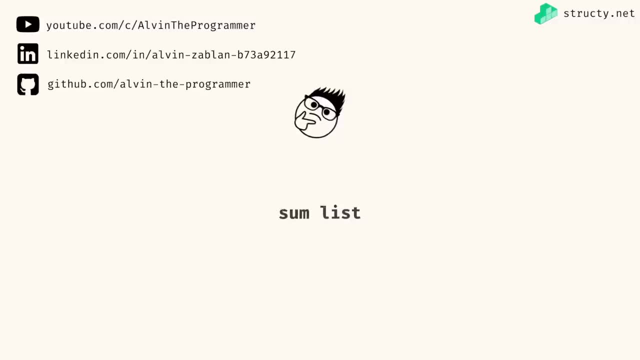 go over an approach we can use for this sum list problem. So in this problem we're going to be given a singly linked list containing numbers as the values. what you want to do is return the total sum of all the values in the linked list. So for this particular input we should return: 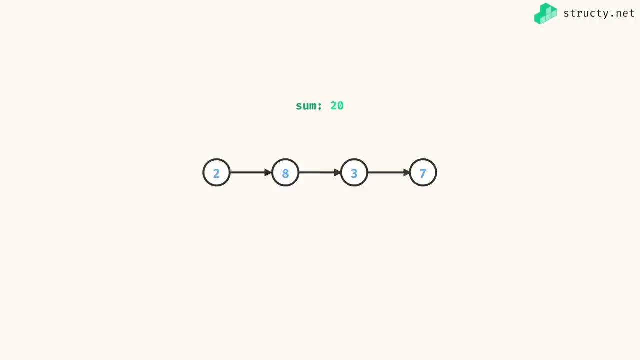 a total sum of 20.. And so how can we go about solving this? really, just reviewing a core linked list pattern, right, All you have to do here is just traverse in order through the linked list And you can accumulate a sum. So let's say we start from the beginning. 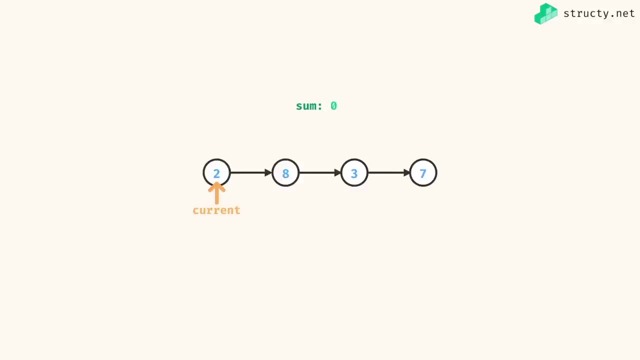 If we initialize some some variable to zero, we can also just use a pointer that starts at the head of our linked lists And what we can do is we can take current value and add it into our sum, just updating the sum. So I take my current value of two, add it. 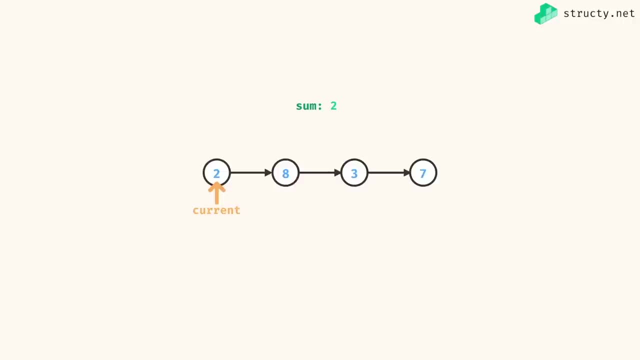 to my sum. my total sum is right now. to that I can set current equal to current. next, I can add this eight into my sum, getting 10.. Next iteration, I can add my three into the sum, getting 13.. Next iteration, I can add seven into the sum, getting 20.. Right And. 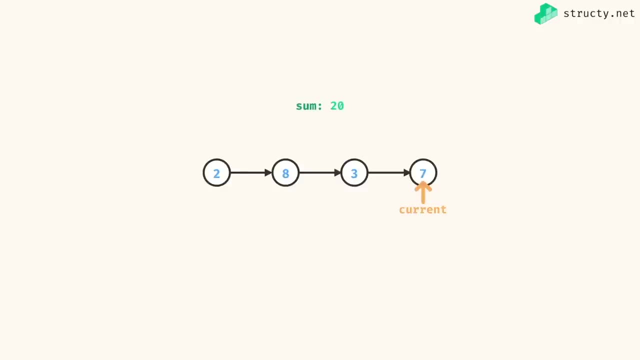 I know that technically, seven does have a next pointer and it does point to null. So let's say I drew that out explicitly. what I can do at this point is actually: I can add my current value to zero And then I can actually continue my algorithm, And I can. 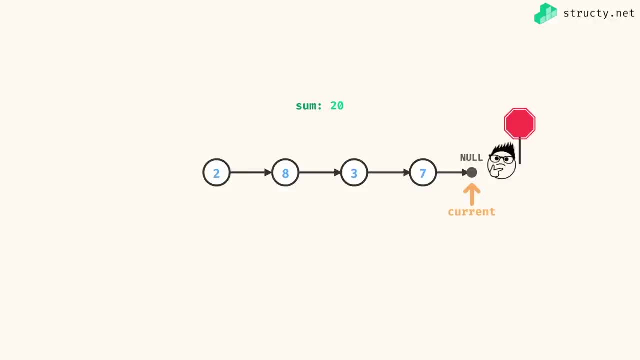 make the stopping condition when my current points to null. right, So in general, we can call this up by saying a loop, like you know, while current is not null. we talked about the complexity of this algorithm. it's pretty straightforward. We're technically just iterating. 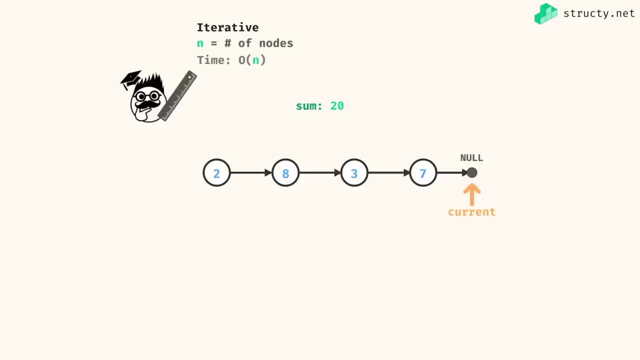 through every node. So if n is a number of nodes, we have O of n time, roughly one iteration of for every node, And then our space complexity here is actually O of one. if we do this iteratively right, the only variables we need to maintain early, just current. 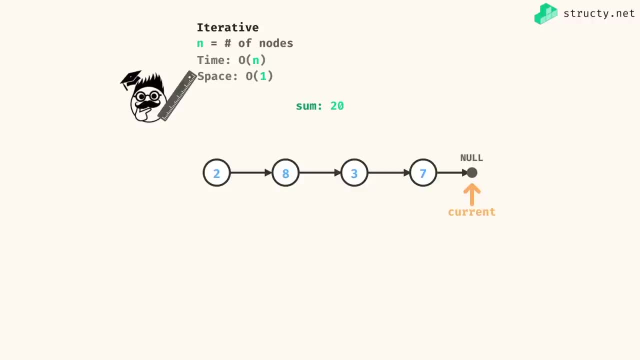 With the sum variable and we're just going to store some primitive values in there. So we have a nice constant space solution over here. So the iterative is really straightforward. Just for you know- complete understanding- how can we solve this one recursively? Well, 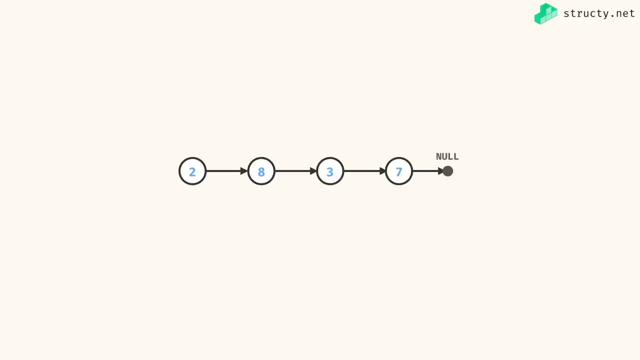 if you solve the recursively, that means you have to, you know, call your function many times And we start with a top level- call on the head node of two, And what this should do is really just call upon the next node. right, so I could should call upon head dot. 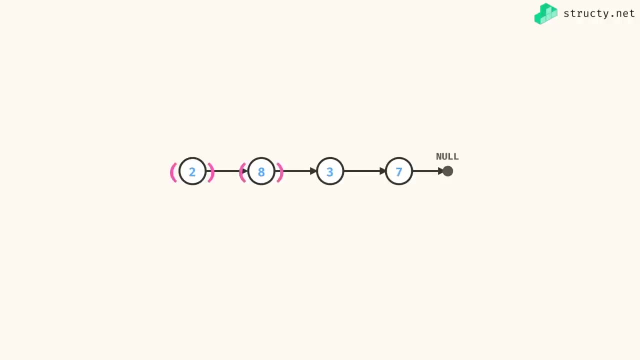 next. So that should give me a call to this eight node, And that should call upon the three node, And that should call upon the seven node, And finally, the seven node should actually call upon its next, which would be the null node, And that will actually act as my base case. I think it's a really great one. What 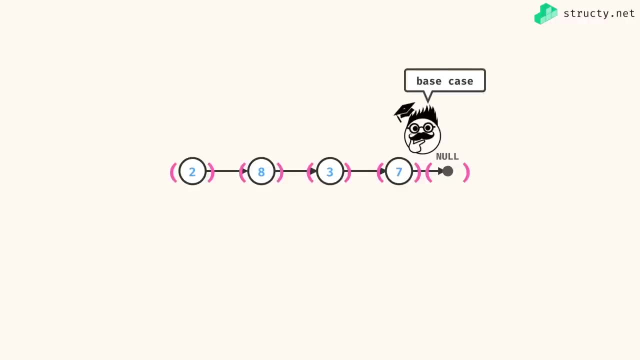 I can do with this base case, right? if my node is null, then I can just return zero, right? Think of null as if it's an empty link lists. what is the total sum of an empty list? Well, that would definitely be zero. So I'm going to plug in this return value, right? 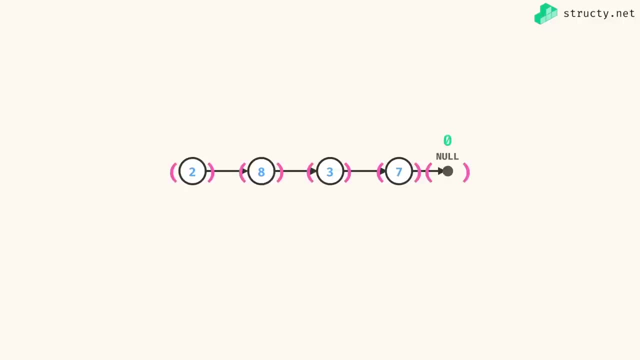 So I'm saying this call to the null node is going to return zero. When we say return, that means return to your caller. So this zero would actually be returned into the seven node. And what the seven node should do is add its current value, right its own value. 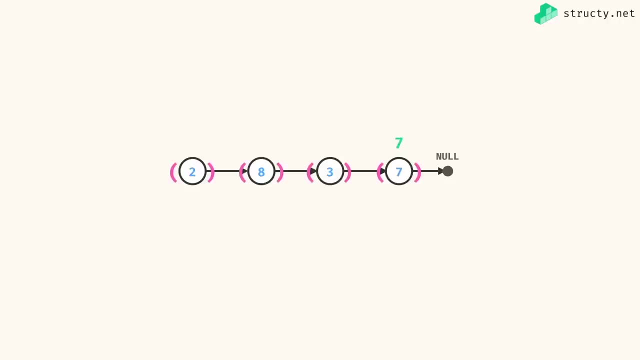 into that number, giving seven, and then that returns up the stack. At this point I returned back to the three node. three can add its value with that seven, giving 10.. And just returning that up, Eight can do the same, giving me 18.. And finally, two can return to the. 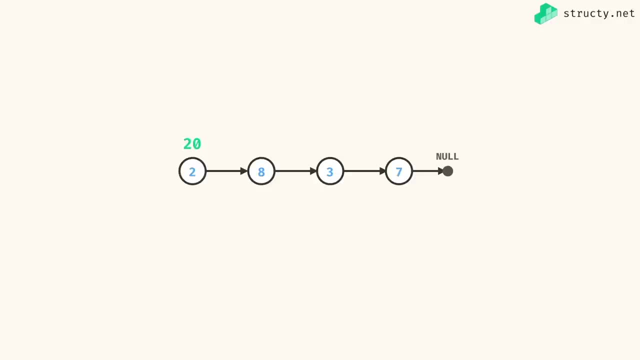 null node So we can add itself into that return value, giving us 20.. And that would be the correct answer, right? So there are plenty of ways to implement this one. If we solve it recursively, we're definitely going to have one call for every node within our 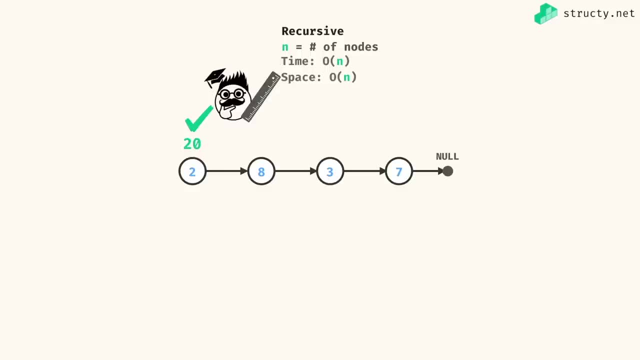 link list. So that'd be O of n time And the space complexity would actually be a little more than our iterative. we would have O of n space here because of the call stack right. Typically, when we analyze our recursive functions, we should include the space utilized for making 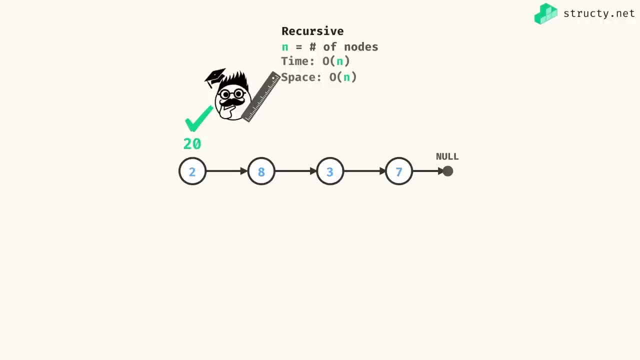 these recursive function calls right. So O of n over here And notice that when we bought them out at our base case we would have you know roughly like four or five things on the call stack. Alright, so those are the two strategies I'll. 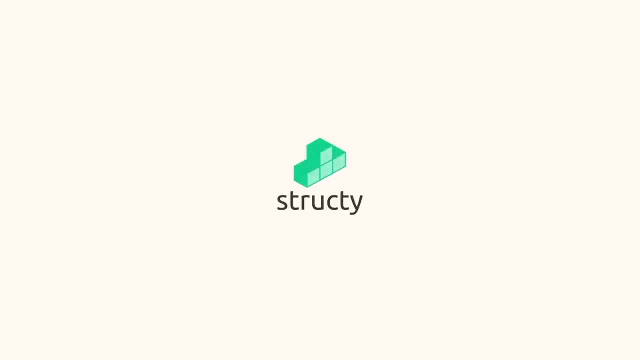 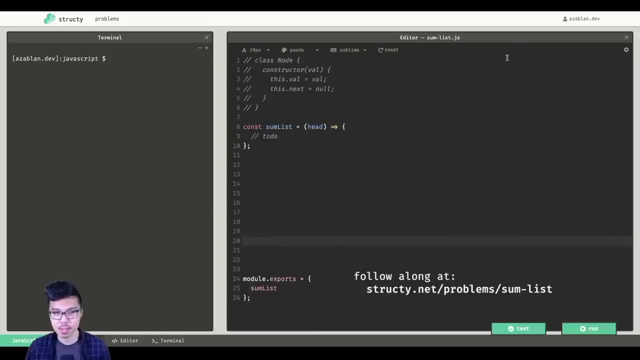 think will code up and I'll catch you in the walkthrough video. Hey programmers, Alvin here, Right now I'm gonna go over a JavaScript solution for this sum list problem. So I think we'll get things kicked off by implementing a iterative version for this. So I know I. 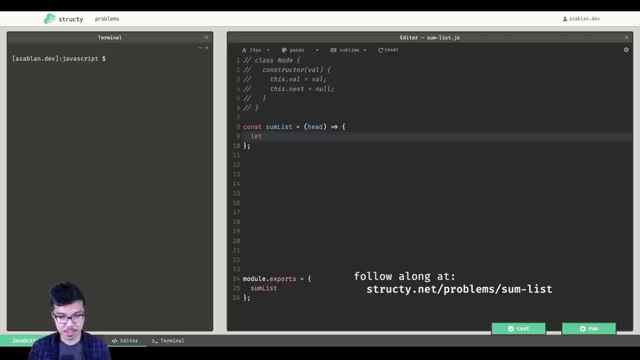 want to create a sum and add to it over time, So I'll create that variable. I'll say: let sum equals zero. I know by the end of this function I'm just going to return that total sum. Now I need to lay down my very- you know- standard code for just traversing through a linkless. 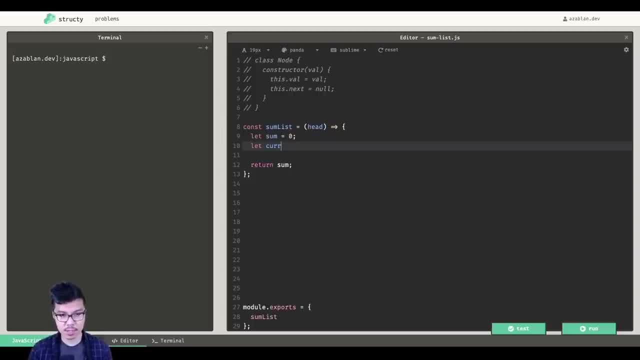 So I'll say: let current. I'm going to keep updating this variable over time And it's going to initialize with simply the head node, And I know that in the loop for this kind of classic linkless traversal, I just want to iterate while current is not equal to null. 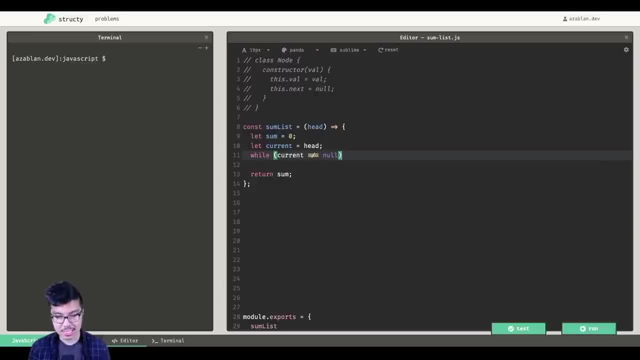 right. If it's not equal to null, then it's a node, So I can actually look to its next pointer. So I know I'm going to need this pattern right. set current equal to current, dot. next, this actually steps through. you know the linkless and sequence, But how do? 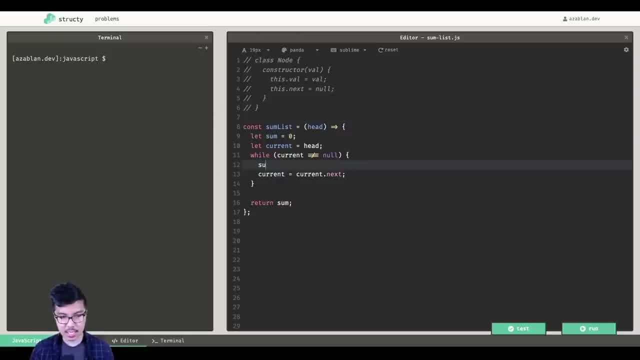 I actually want to utilize my current nodes value. Well, I just want to take it and add it into the sum right. So sum plus equals current dot Val And eventually, once I hit the very very end of the linkless, I know current is going to be equal to null. So I 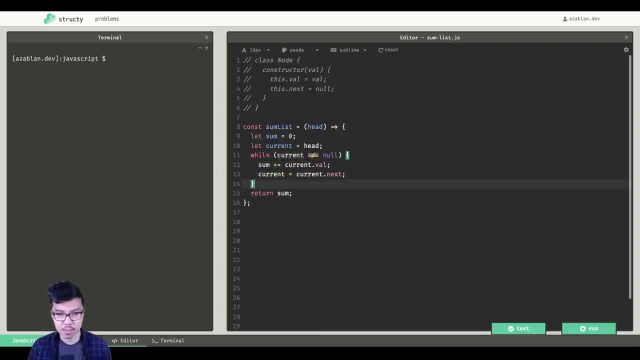 exit the while loop, And then I'm going to add the sum, And then I'm going to add the value, And then I'll just return my total sum. So let's run this just a little variation off of our last problem, just doing some computation along the way, Nice, And now I think I'll 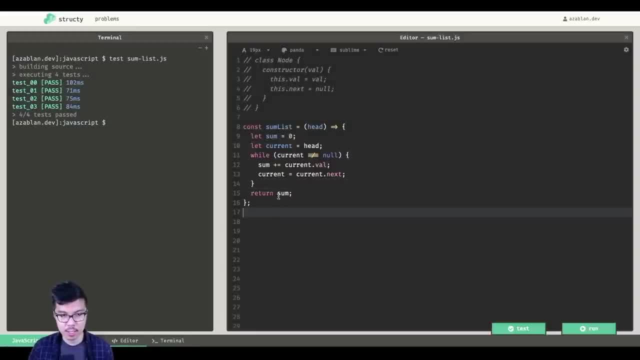 show you the recursive version, which I quite like. So for your recursive version, it's all about starting with a meaningful base case, right? So first thing to think about is: alright, typically for my linkless problems, my base case is about my head being null. 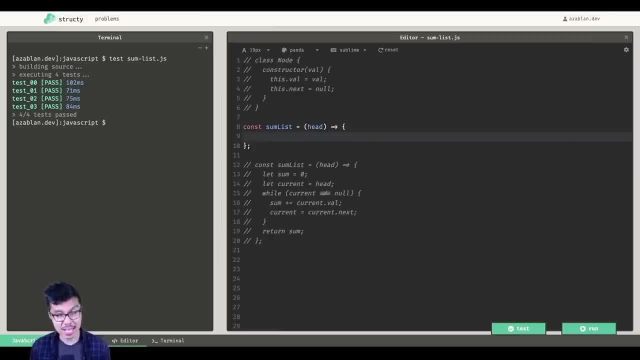 right, And that kind of represents the scenario where this is an empty, linkless right. If it's null, it means it has no nodes. So what's the total sum of an empty link lists? Well, it's just zero. So I'll check if head is equal. 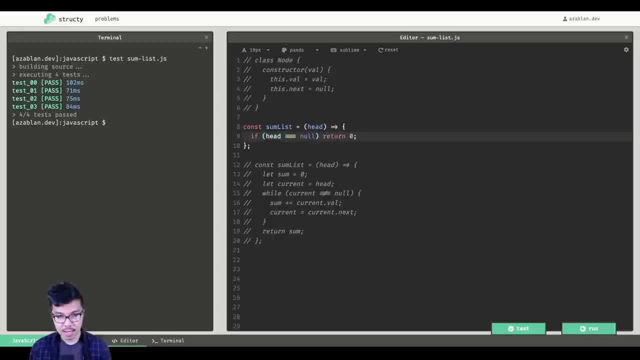 to null, then just return zero. And it's important that I think about compatible types here. I know when my link list actually contains some nodes, then I should return a number, And even in the base case I should return a number. it's just the case that I returned. 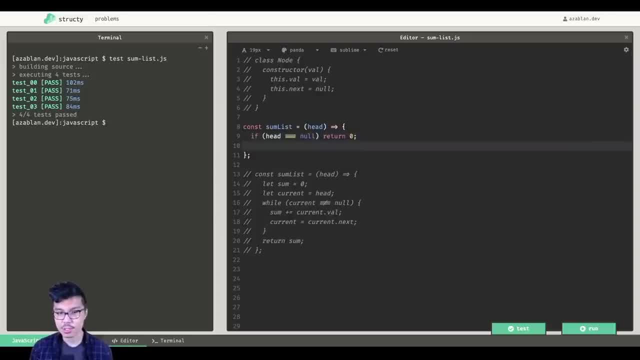 the number zero. Nice, Let's say. now we write our recursive code. right, If the head is not null, then it's actually a node, So I can look at its value. right, It's a head, dot, Val, And what I want to do is take that number and add it to the sum of the remaining. 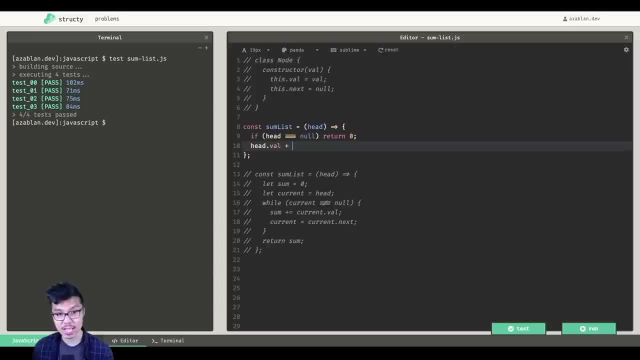 nodes in the linkless. How can I get the sum of the remaining nodes after my current position? Well, that's just about calling your function recursively right And passing along head dot next right. So always try to think about your recursive call for the type of data that 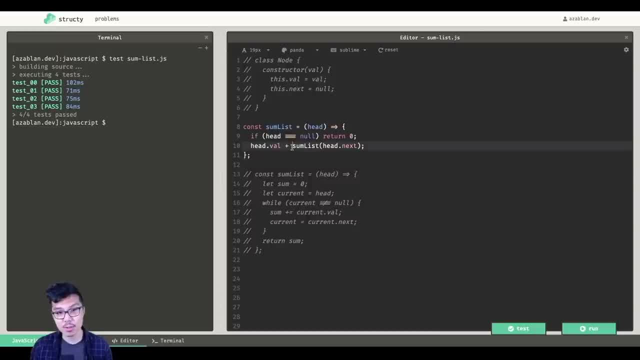 it returns right. It gives me back a number representing the total sum of everything's starting at the next node. I'll take that number, add it to my value. that should give me my complete sum. So I'll just return it. So I'll give this a shot And the recursive 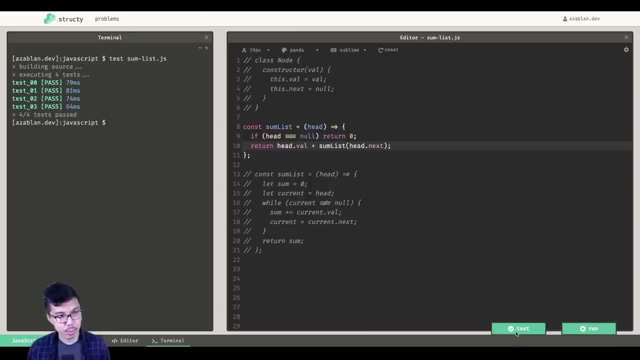 code is quite short. One thing we should consider, though, when it comes to like an apples to apples comparison between the recursive and the iterative. they both have the same runtime right. They both have O of n In the case of my recursion. I have n calls In the case. 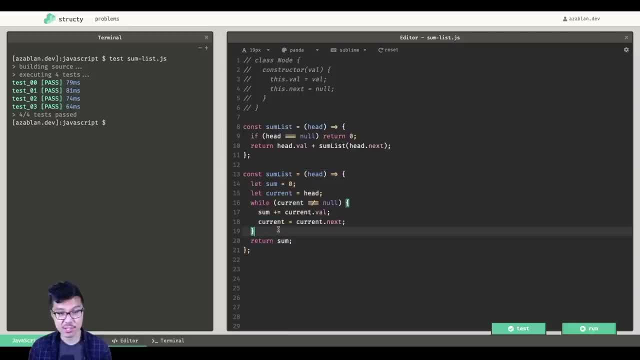 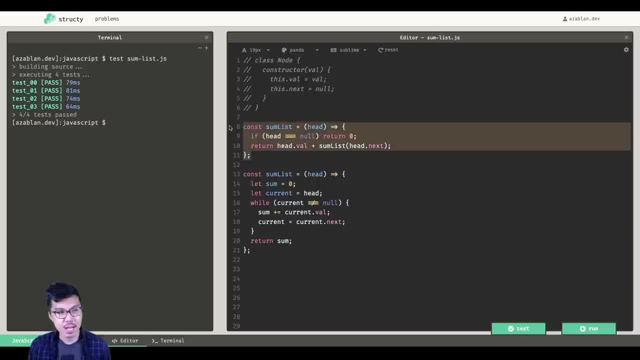 right. That's because for recursion we actually have to add every function call onto the call stack. So I know by the time that my recursion bottoms out at a base case I would have n calls on the call stack, Whereas in the case of our iterative code we would actually use 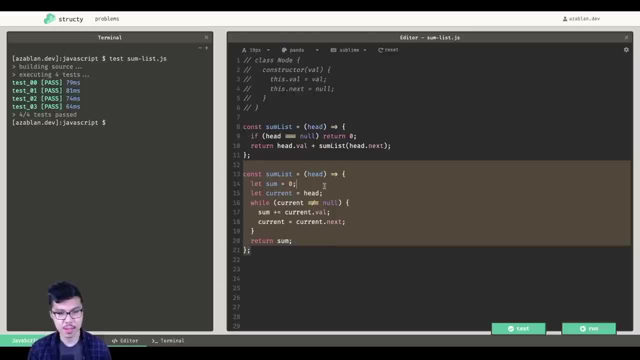 only a constant amount of space. they only use a handful of variables here. That being said, I highly recommend that you practice both of these solutions because, depending on the problems that we solve, you may find a one more natural to use than the other. Hey, programmers, 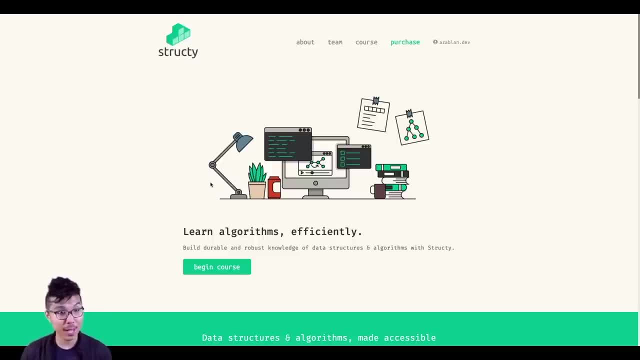 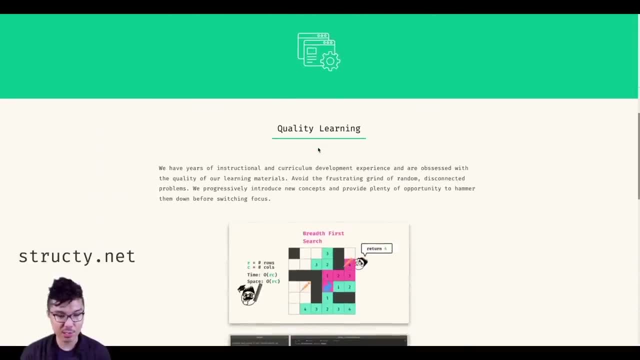 before we continue the course on linkless, I just want to make you all aware of my own data structure and algorithm platform, that is struck tnet. If you haven't noticed already all of the content that you're watching in this course, as well as some of my other material- 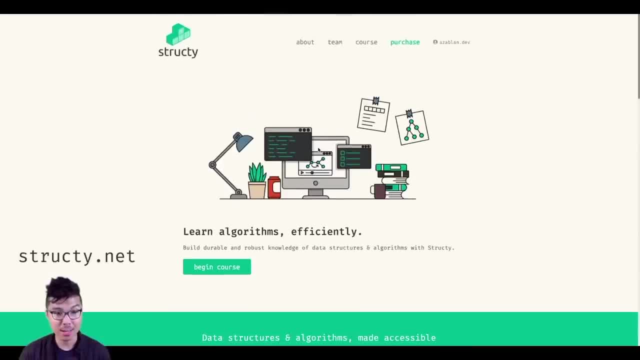 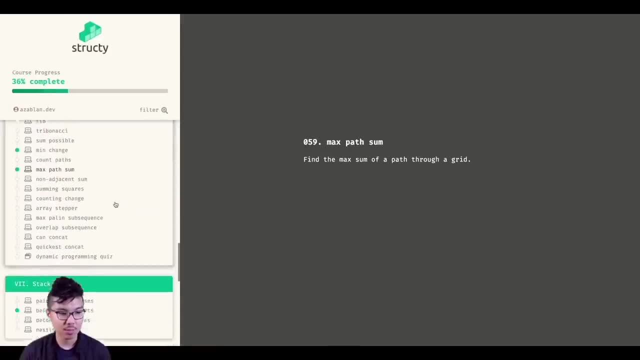 on free code camp is also on struck tnet, with a lot of other topics covered as well. So we go into the course. I cover all those classic- you know, data structure and algorithm topics with tons of videos for every single one. So if you like my teaching style, I think 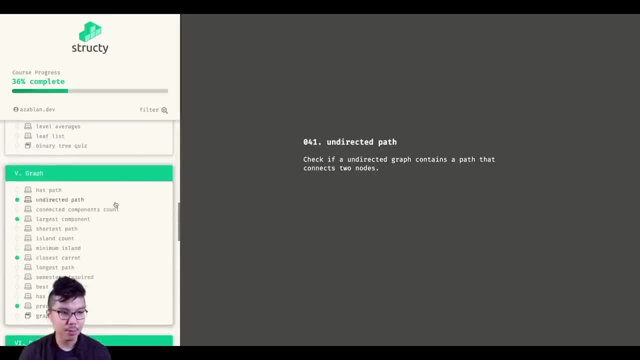 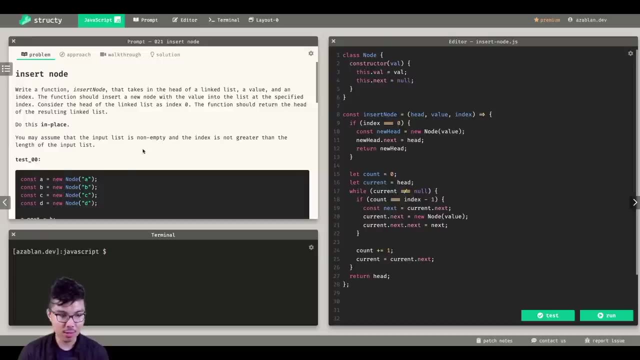 you'll also enjoy struck tnet And if you hop into any particular problem I'll give you a quick little tour over here. So if we go to this insert node problem, like you expect, you can write your code, you can view the problem, you can run your code. see the output. 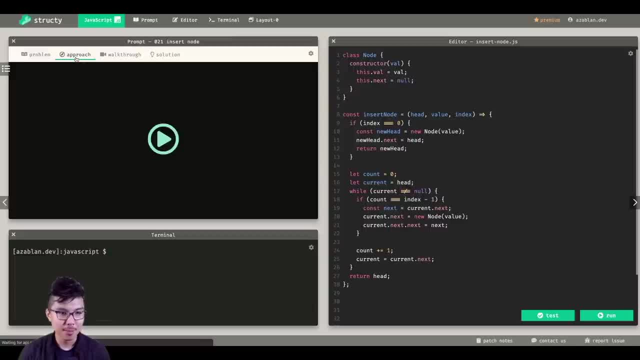 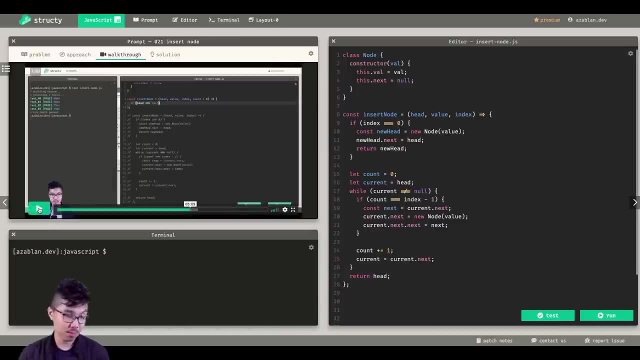 I think, most importantly, what will bring you the most value is my kind of signature of videos right, So you're going to be able to have a high level approach for every single problem. as well as the code Watch There's, you get the nuts and bolts code implementation for every single problem, And even still. 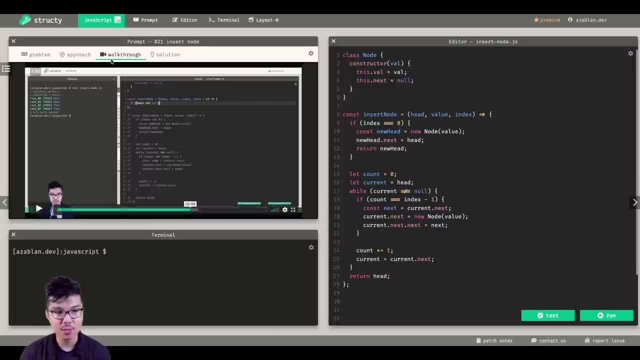 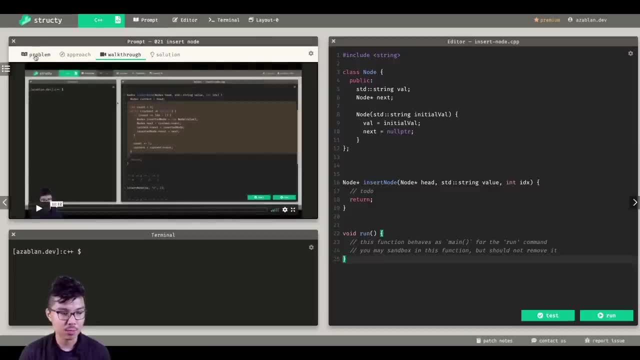 if you're not like a JavaScript. I know that this free code camp video is in JavaScript- you can totally switch the language. So for all of my C++ people in the crowd, doing so- that is switching to C++- would obviously change the prompt in the text editor, But also you'd. 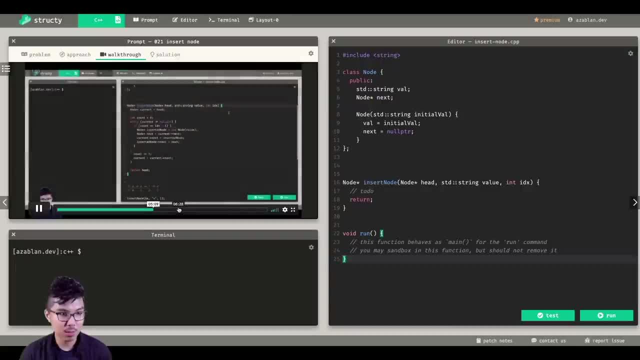 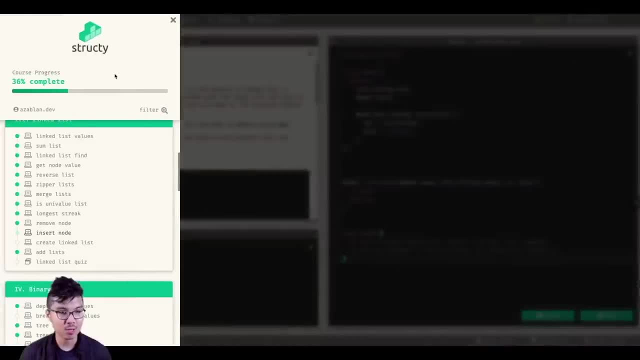 get different videos right here. you see a C++ specific video over here, right? So if you've been enjoying my content and just want to check out more data structure and algorithm material with me, head over to struckty dotnet. I'll leave a link to the. 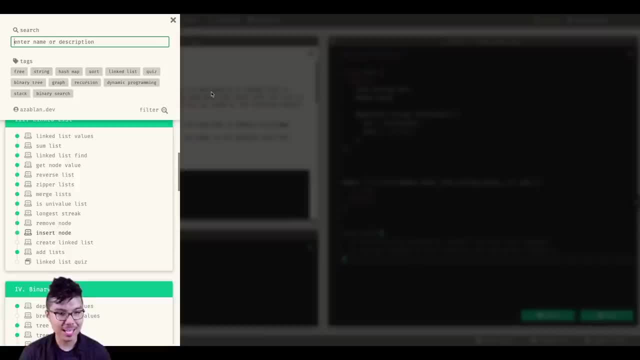 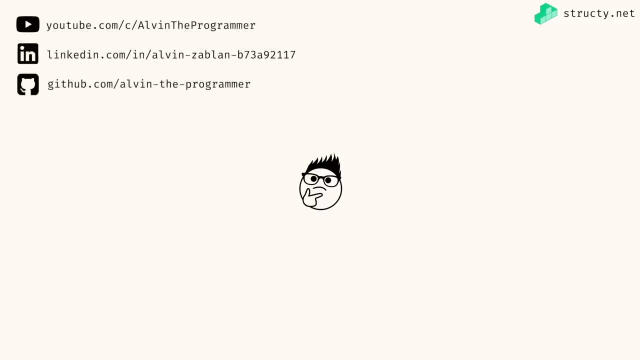 platform in the YouTube video description. And with that, let's head back into our link list course. Hey programmers, welcome back. right now I want to go over the approach we can use for this link list- fine problem. And I'll show you two ways to solve this one. So in this, 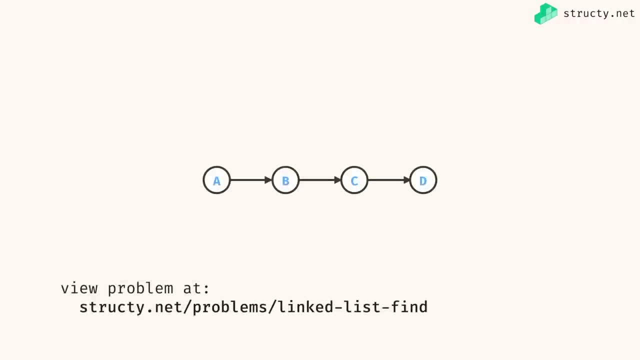 problem. we're going to be taking in a linkless as input And we also have a target value. What we want to do is return true or false, whether or not the target value is contained within the link list. So let's take this행it list And we want to make sure that when we're 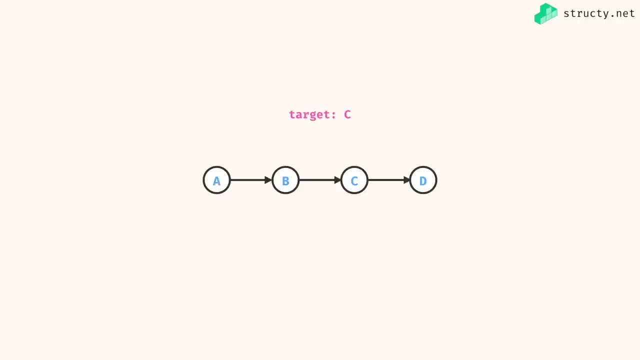 linkless. So for this particular example, if I'm asking you for a target of C, you should return true because C is definitely within the linkless. In another scenario, let's say I gave you a target of G, In that scenario you would just return false because G is not a value of this linkless. 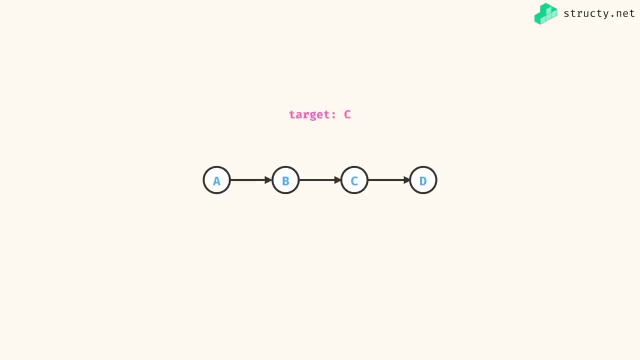 To solve this one. we're just going to use our classic linkless traversal algorithm, So we'll step through it as if we're looking for C. So in the long run, we expect to give back a true here. Well, I know that they're going to give me the head of the linkless as input And I'll create. 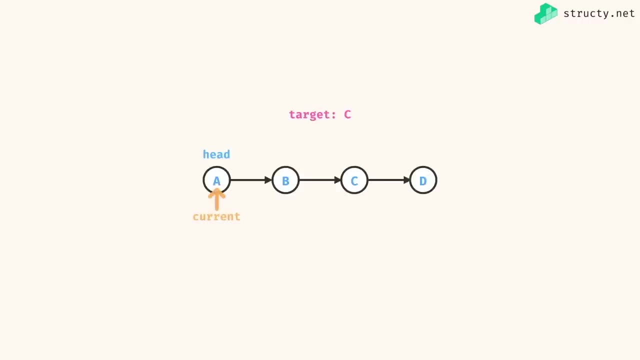 a current variable that points to the head node. Of course I'm going to progressively update this current variable to be the next node over time, right? So what I can do is, whenever I'm situated at some current node, I can check if my current value is equal to my target value. So right now, 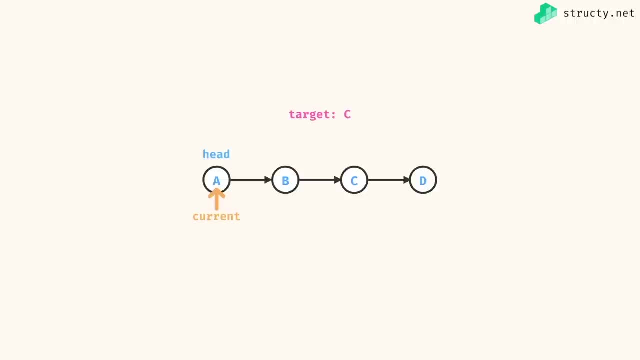 I would check: is a equal to C? it's not, And so I should keep looking through the linkless. I know that current also has a next property, So I'll update current to be current dot next, And then I check: is B equal to C? 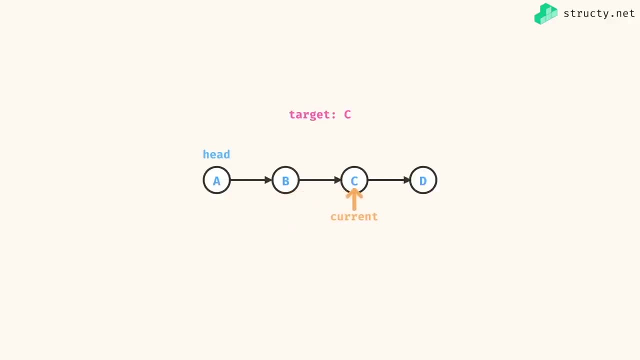 it's not. so I keep going And finally I can hit a point where I see that my current value of C is equal to my target value of C, And so I can just do an early return- true right, Once I find a match. 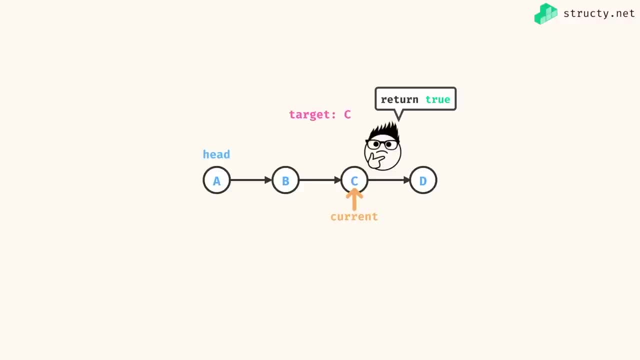 within my linkless. I can just return my final answer. Now let's say we had the opposite scenario. let's say that my target was G. we're going to start the algorithm in the same way we start at current And when we keep looking through the linkless and we set current equal to current, 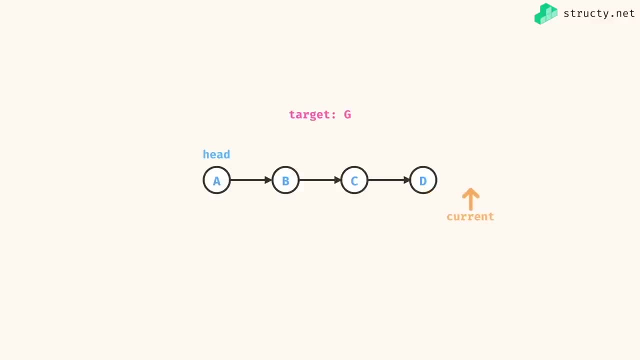 next, eventually, we know that current is going to be equal to null, Which sort of signifies that we've hit the very end of our linkless Right. And at this point, once we finish iterating through the entire linkless, we know that we didn't see the target. 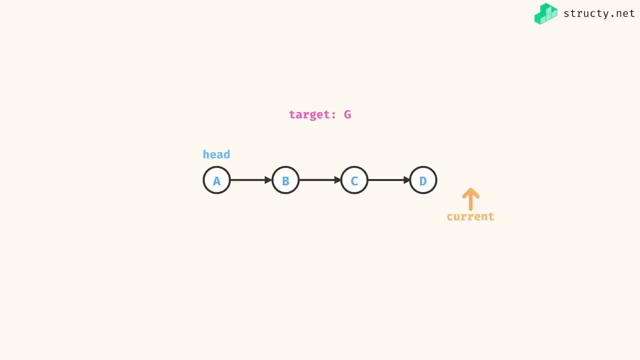 value because we were checking the entire way through, And so at this point we can do: return false. this is a really practical programming pattern, right? Or we check some conditional inside of a loop And if we find something we're looking for, we'll return true early. 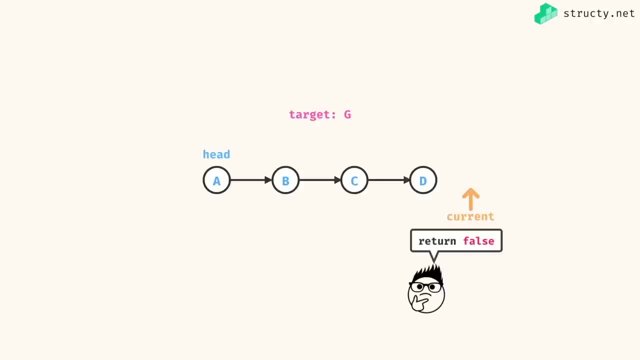 then afterwards, after our loops done running, we'll return false late. We talk about this iterative strategy. we know that if n we're going to return false late, we're going to return false. n is the number of nodes we're just going to iterate through every node of the linkless. So we 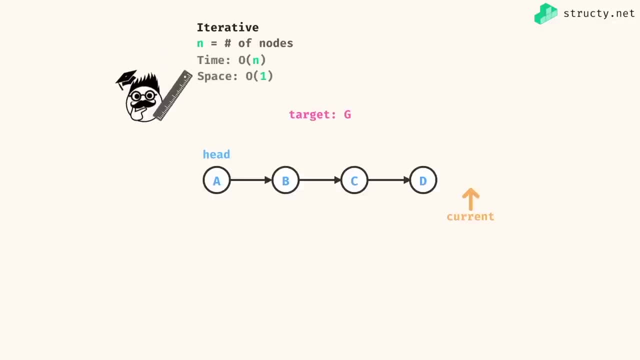 would have a runtime of O of n And our space complexity here would just be O of one, because we're just using a constant number of variables. So that was the iterative solution. How can you also solve this one recursively? So let's say we were looking for the target of C and we had a. 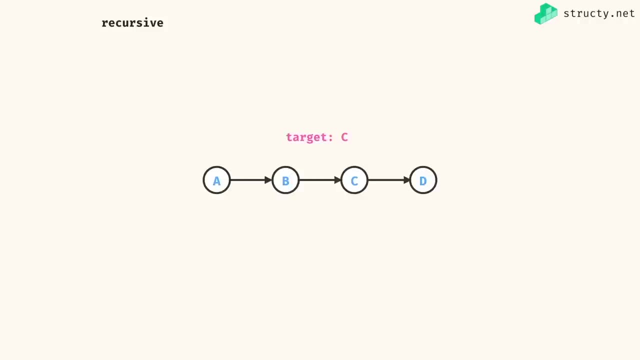 more recursive point of view. So we know we're going to make a top level call on the head node of our linkless And I can just think about some base cases to use here, right, And I know I need two base cases, right. 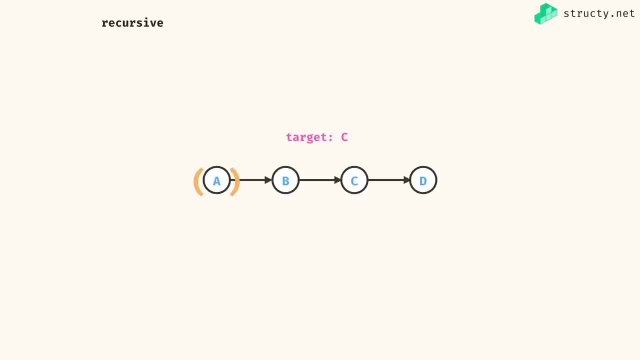 One that can return true and another that can return false. So for my first base case I can just simply check: alright, if my head's value is equal to my target, then just return true. And the opposite scenario, let's say that my head is null- then I should just return false, What I always 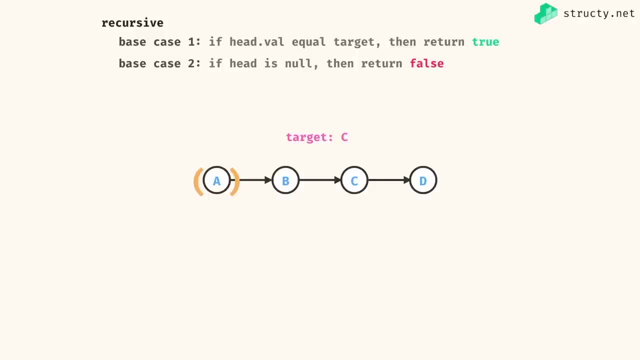 try to do with my recursive code is to think about my base cases as if they're their own valid inputs. So in particular for base case number two, if head is null, then that kind of represents the empty linkless. If my linkless is empty, then I can return false because I definitely can't find the target within. 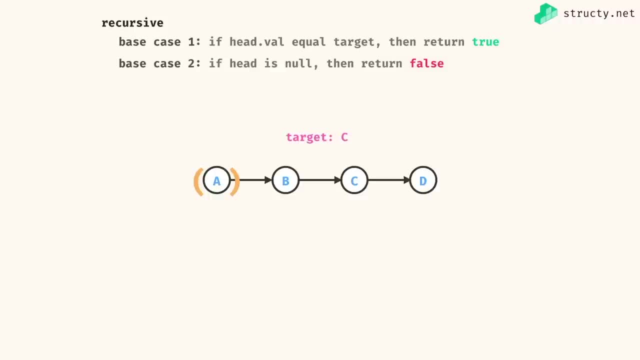 an empty, linkless. So how would this run for our current input of target C? Well, I would check. Alright, is a my target? it's not, so I make a recursive call upon B, same thing, right, It's not. make another call upon C. And at this point I see that my current heads value is equal to my target. 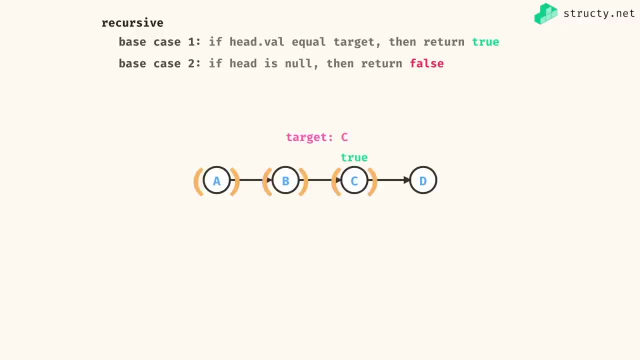 And so this node is going to return the Boolean, true, And I know that this return value is going to return back to its caller of B, And then B is going to pass it back up to a and, of course, a returns it to the very, very top level call. 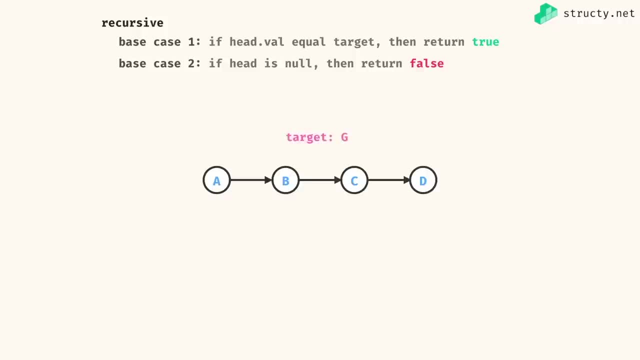 Let's say we had a scenario where our target was not found within the linkless, like G. then we can see the other base case fire at the very end, right. So I know I'm going to make a call on a. a calls B because C. I still don't find the value. 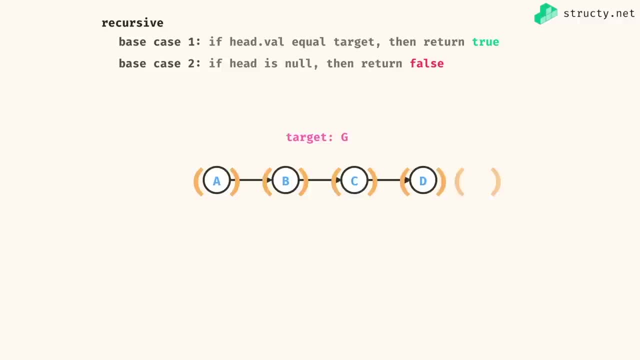 C calls D And finally, when D looks at its next, it's going to pass along null. right, Because these next is technically null And at this point I have just hit base case number two, so I can return false. 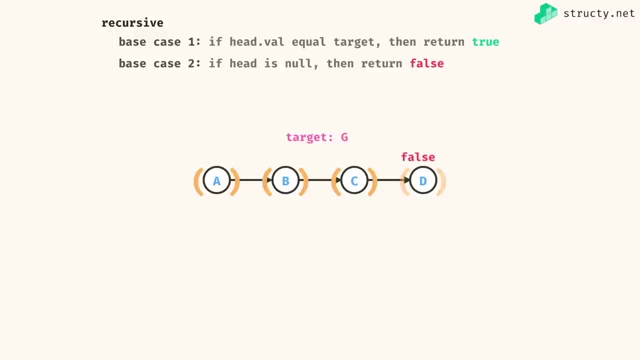 And, like before, I returned these values up the call stack. When we talk about the complexity of this recursive algorithm, we can say that n is a number of nodes. we're definitely going to have O of n runtime because we make a call for every node of the. 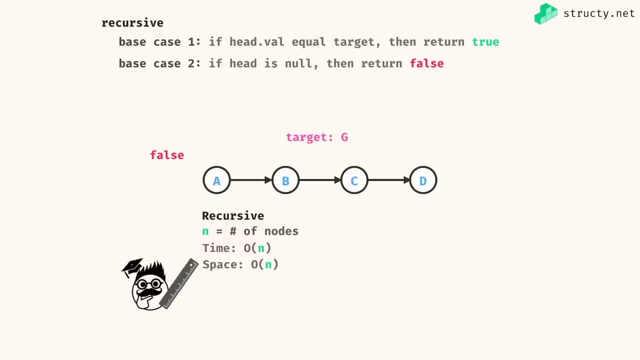 linkless. But we also have O of n space right, Because each of those calls, by the time we bought them out at a base case, we would have to store those on the call. So we're going to have to store them on the call stack. We know that the worst case scenario. 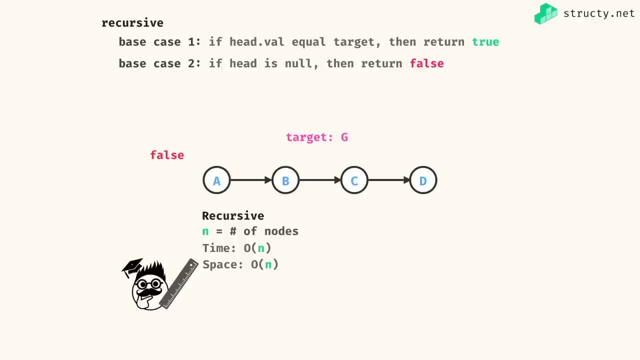 is if our target is not found within the linkless. That being said, I think these are two fair algorithms to go ahead and implement. So give it a shot on your own And if you get stuck, I'll catch you in the walkthrough videos. See you there. 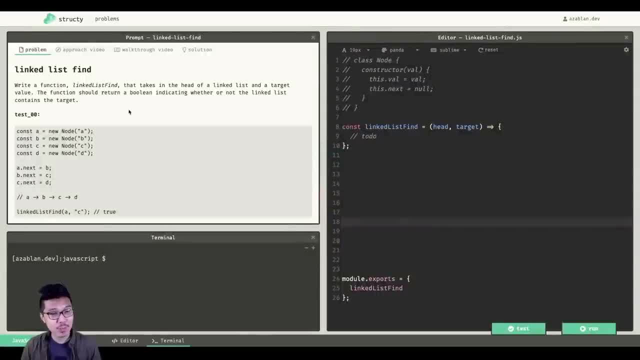 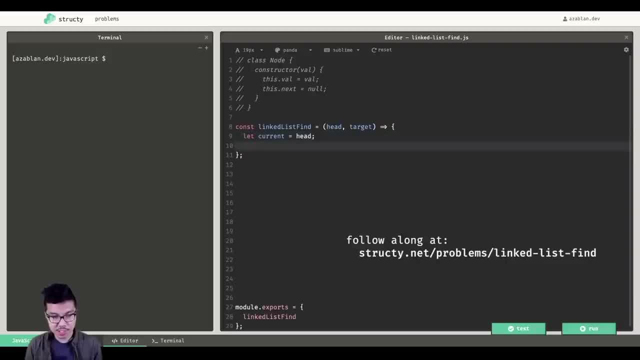 say: let's current equal the head And we'll just lay down the foundation right? We know we always need to iterate. Well, current is not equal to null. And while it's not null, if you want to progress to the next node of the link lists, just set current equal to. 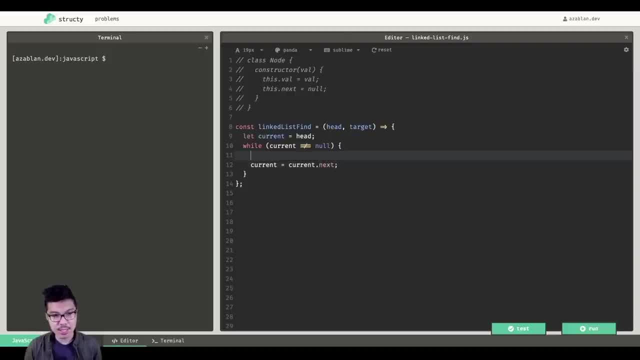 current dot next. Now I just need to work in the logic specific to this problem Right As I check every current node, I want to see if it's value, So if current dot Val, if that is equal to my target balance. 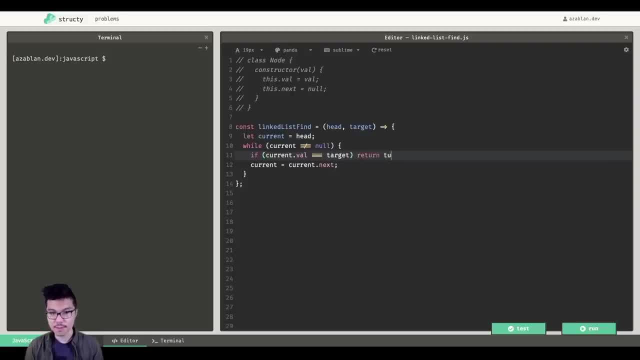 So, first of all, what I want to do is go over everything in the task operator And 강 РазKanna target, And if it's equal to my target, then I can just return true, because I found the thing I'm looking for. What I want to do is return false only after the while loop, right? 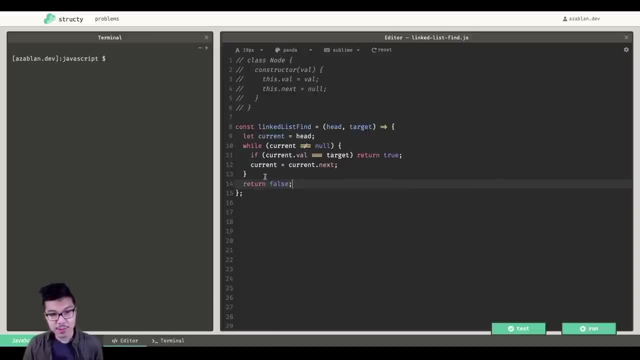 It's important that I return false after the while loop, because only after you check every single node of the link lists can you actually confirm that hey, the target value is not within the linkless. what you don't want to do is write a like if return true and then 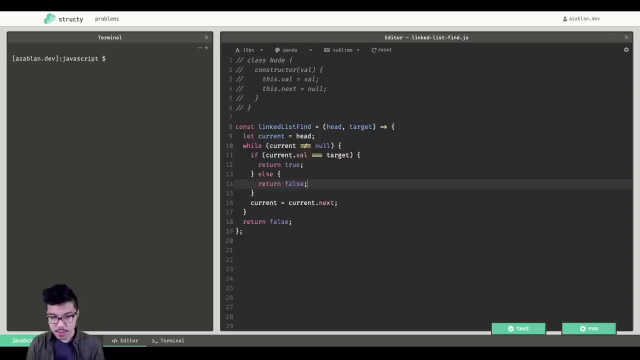 else return false. right, this code would be wrong Because, let's say, you don't find the target value in the very first node of the linkless, then you would just incorrectly return false without even looking at the rest of the linkless. So none of that. we at least. 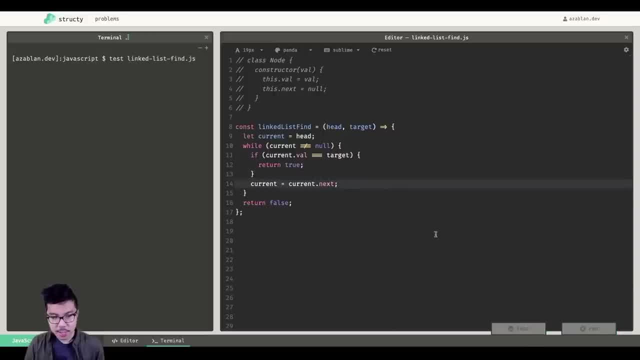 want your code like this, So let's give it a test run, see what we get. Nice, And there we have our iterative solution for this linkless find problem. Let me quickly show you the recursive version of this. it's going to be very similar, So in the approach video we 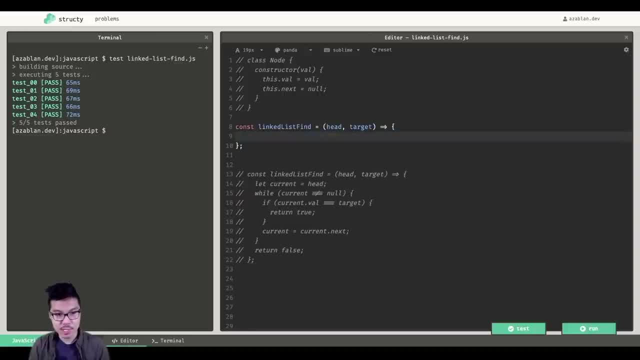 if you haven't watched the approach video, recommend you do. But in the approach video we mentioned that we can solve this recursively by just using two base cases. right, I'll start with the base case if my head is equal to null, right? so that kind of represents. 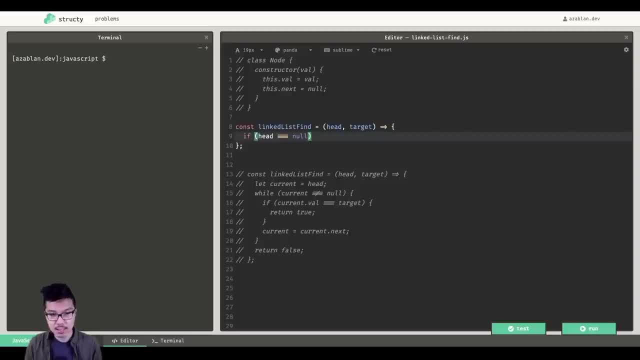 the end of my linkless or also just the empty linkless. So if head is null, I can't possibly find the target within an empty link list, So just return false. Now I need my other base case, right, I need my like affirmative base case. So if head is not null, then I. 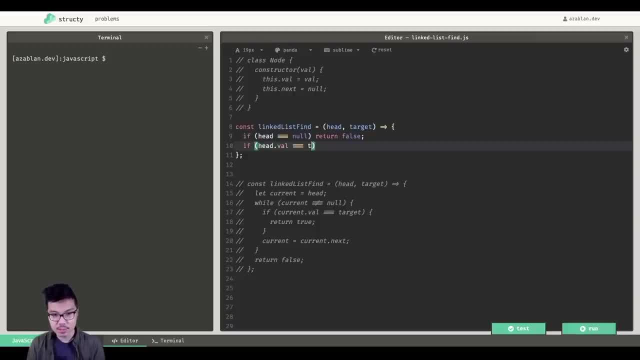 can look inside Of head, I can check if head dot val is equal to my target And I've just found the thing I'm looking for. So just return true. So two base cases here, right? One affirmative and then one that returns false. But let's say neither of these are true, right? So my head? 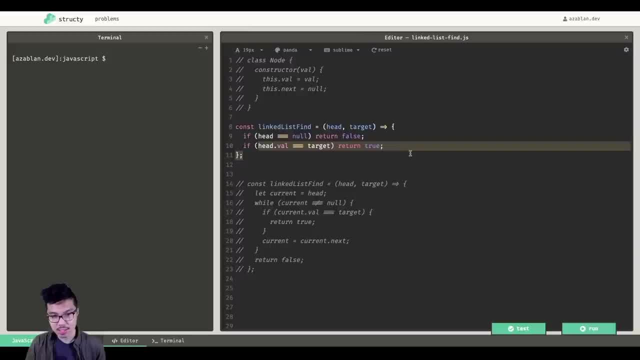 is not null And my head value is not equal to my target. Well then, I need to check the rest of the link lists. So here's where I bring in recursion And I check the next node. So linkless, fine of head dot next And you can pass along the same. 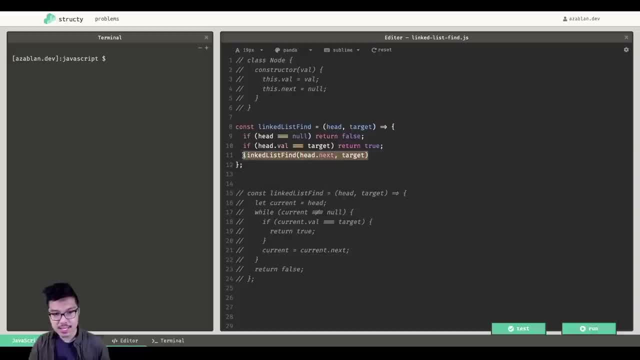 exact target. So this is going to tell me all right, is the target found in the next node of the linkless or in the remainder of the linkless? And I know that this call is going to return a Boolean piece of data right, either true or false. I just want to pass. 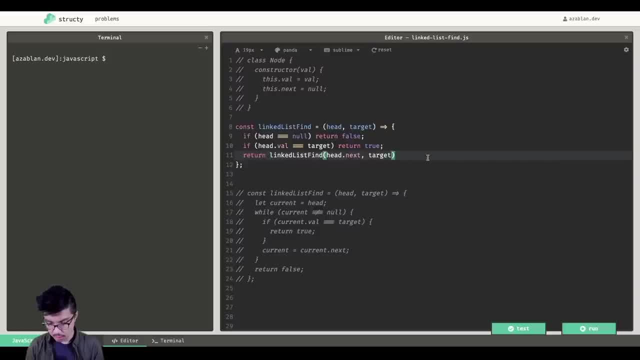 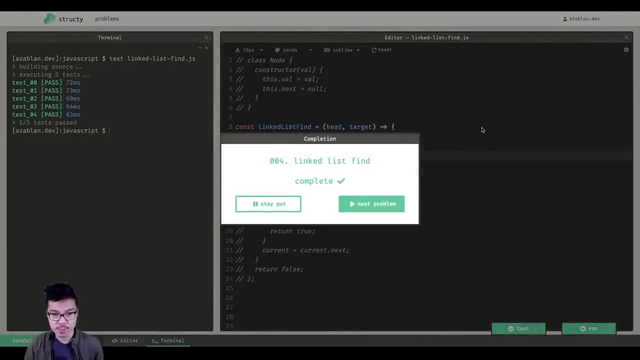 that up. So this should be good to go. pretty concise code: Give that a shot, Cool, And there we have a solution that's recursive For this problem. Do bear in mind when it comes to the comparison of the complexities- Technically we wouldn't want to do that. 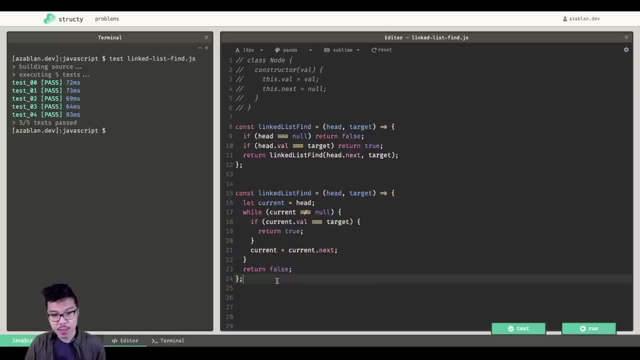 Essentially, we would prefer the iterative version, right? They both have linear time, But the iterative version has constant space, right? So I'm just using like a current variable, whereas my recursive code uses a linear amount of space because of the call stack, That being, 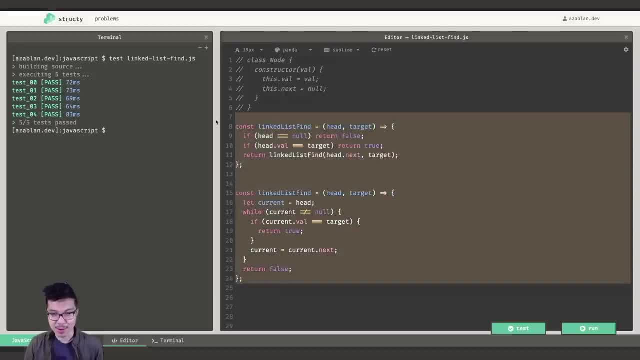 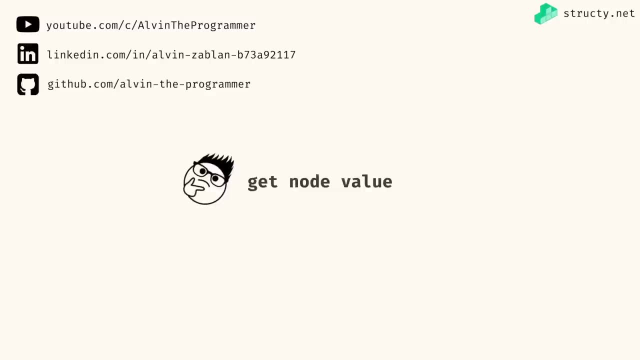 said. what I want you to do is practice both of these solutions and I'll catch you in the next problem. Hey programmers, Alvin here, right now I want to go over the approach we can use for this get node value problem. So in this problem we're going to take in 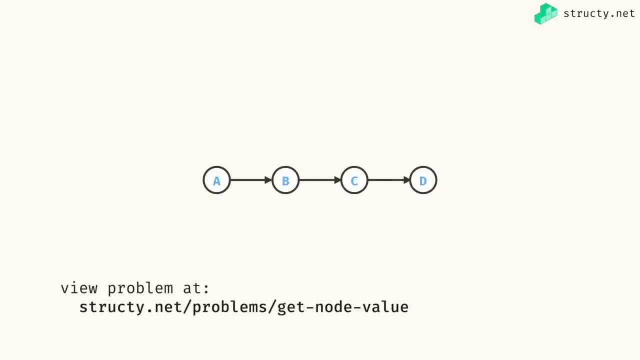 a linkless And what we want to do is also accept an index as input. what we want to do is really return the nodes value at that given index and we will start counting our indices at zero. In other words, we'll consider the head of our link list as having index zero. So for this, 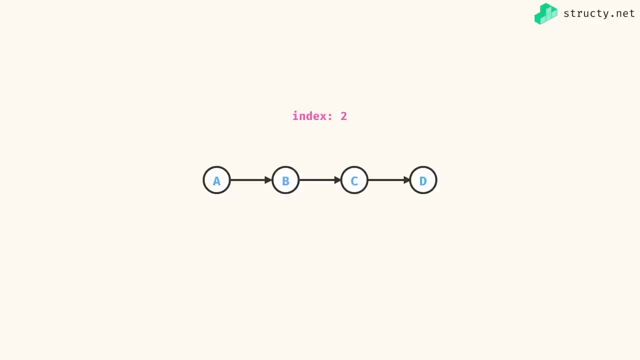 particular example, if I asked you for index two of this link list, you should return the value of the C node, right? So just return the value C And of course I could be giving you any particular index as input. So what this question asks us is: what is the value? 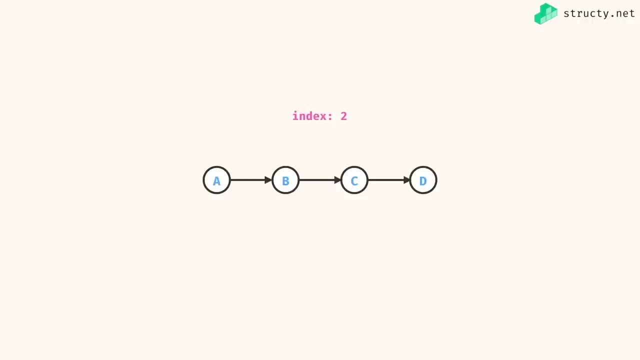 index is pretty straightforward, but how can we go about solving this one? And so what we can do here is a basic counting algorithm. So we know we want to return the nodes value who has index two? So when we initialize our current pointer to be the head of the link, 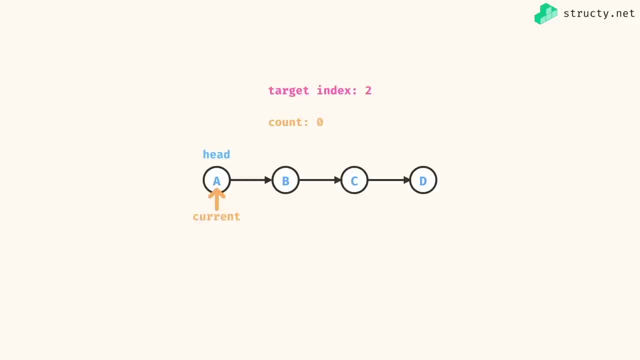 list, we'll initialize our count to zero. Then from here it's just our classic logic, right? I know I can set current equal to current dot next, And when I do that I'll also increment my count. So now count is one. Basically, I have tracked the index of my current index. 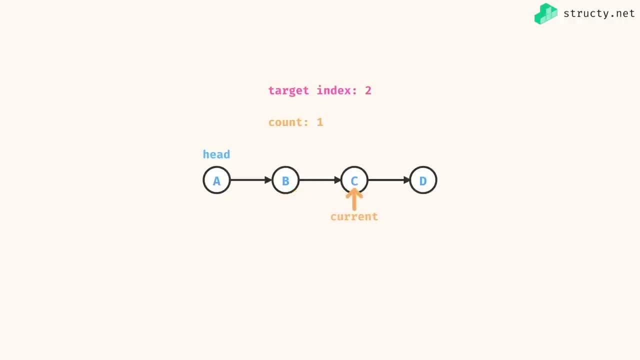 the node that I'm iterating through next iteration, when current goes to C, And of course I increment my count to two. At this point I can see that my target index and my count are equal, And so I can just return the value within that particular node. But think about: 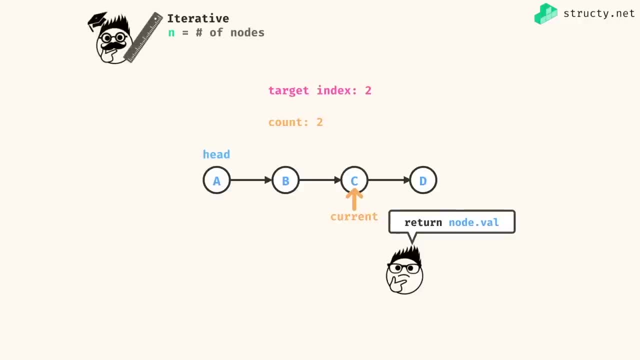 this strategy. it's pretty straightforward in that if n is the number of nodes, the type complexity is simply O of n right, Because in the worst case we just have to traverse through the entire link lists. We can also see how the space complexity for this is constant. 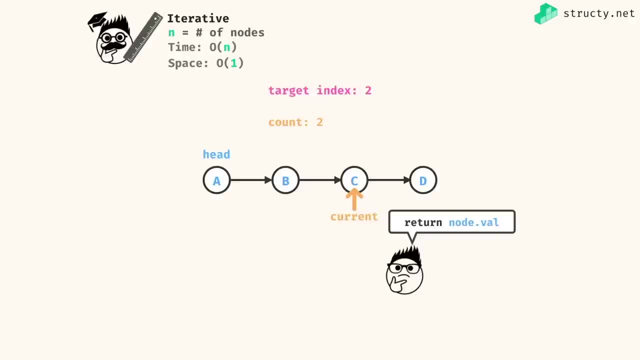 because we're just tracking some simple number variables. So that's how you can solve this one iteratively. How can you also think of this one recursively, though? So let's reframe our point of view here. let's say that we were forced to solve 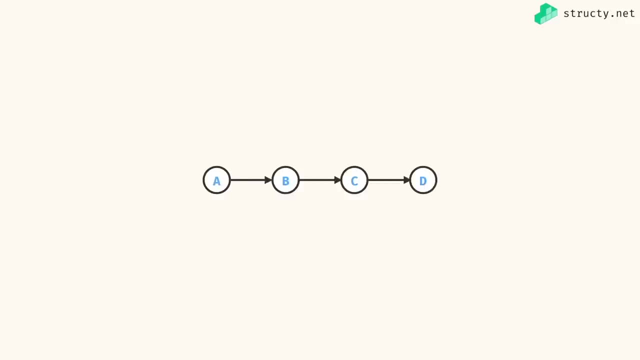 this one recursively And we know we still want to find the value at index two And when I make a call I know that the top level caller is going to pass along the head of the link list, So the a node and also their target index of two. I can use my classic recursive. 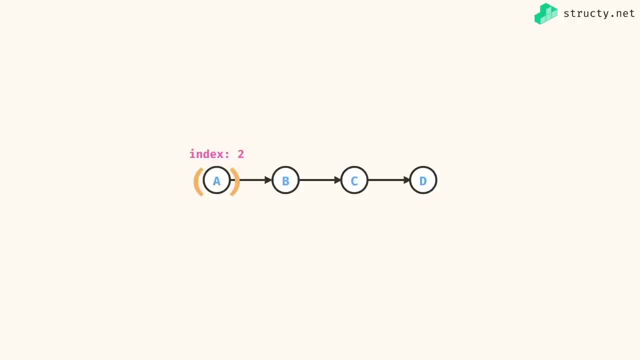 link list traversal algorithm. So I make a recursive call on my next node. When I make the recursive call on the next node, I'm going to pass along the target index of two, And when I make the recursive call on the next node, what I should also do is pass along. 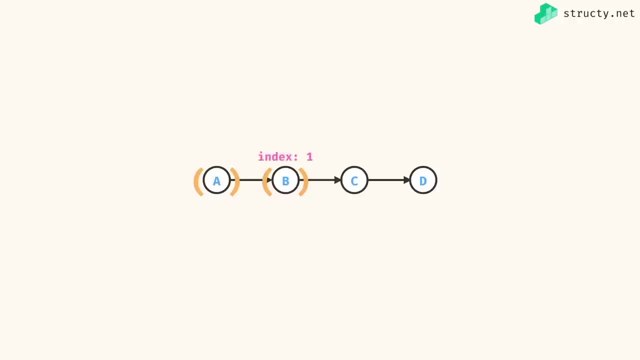 the index but decrease it by one. So now I'm able to see that, hey, this current node of B has index one, And if I keep doing this next iteration, I call upon my next node of C And I also decrements my index down to zero. Once my index is at zero, that basically. 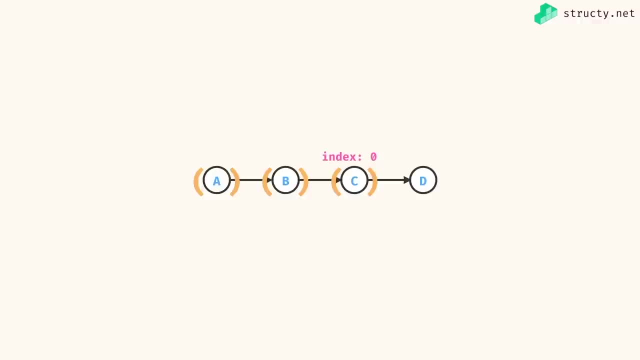 means that I want to return this very node right. So if index is equal zero, we'll return no dot value. that would be our base case, And once we return that value, I know that I'm going to return back up the stack. So 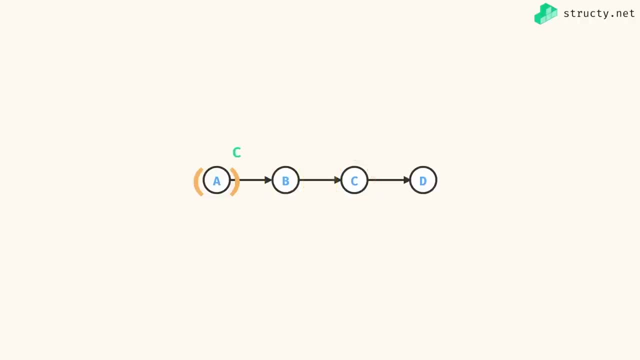 the C value returns to its color, and so on and so forth- Very classic recursive code. So this looks like a nice a recursive algorithm. we analyze the complexity of this. we're going to see that the type complexity is still in here And the space complexity is actually. 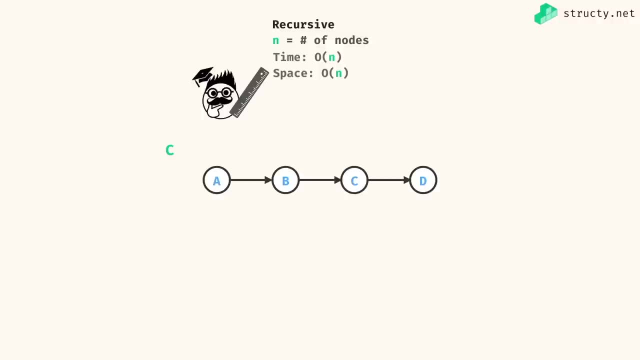 also linear here. here we incur a little more space complexity because we're going to be storing every call upon the call stack. So what I want you to do is, on your own, try, give it a shot and implement both the recursive and iterative solutions for this problem. And 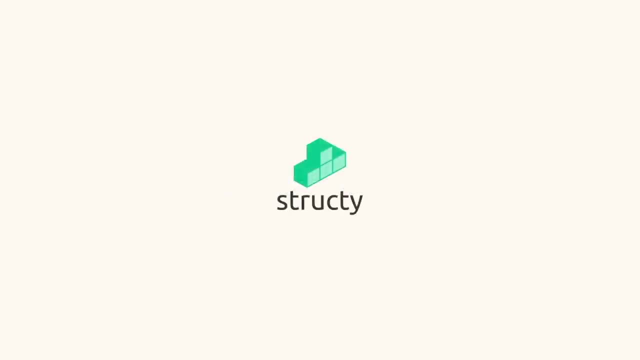 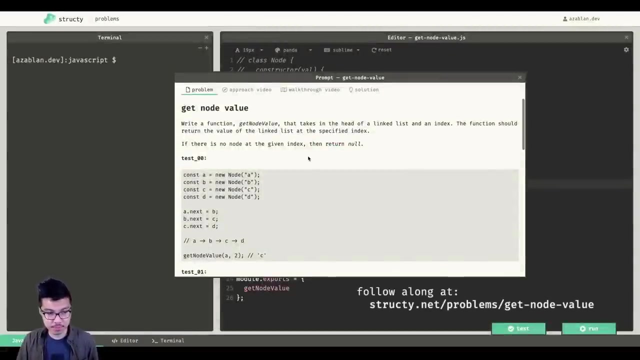 if you get stuck, I'll catch you in the walkthrough videos. Hey programmers, welcome back. right now I want to go over a JavaScript solution you can use for this get node value problem. So hopefully you already watched the approach video. If not, highly recommend you do that, And we'll start by. 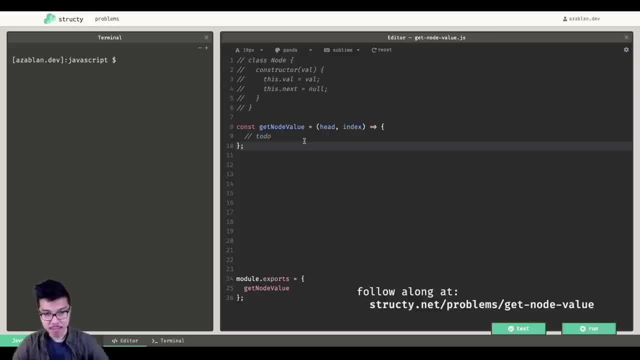 implementing, maybe, that recursive strategy off the bat. So I'm going to need two base cases here, like we said in the approach, And one of them typically is always going to be: if our head is equal to null, that means I've hit the end of my linkless or I have an empty linkless And what I 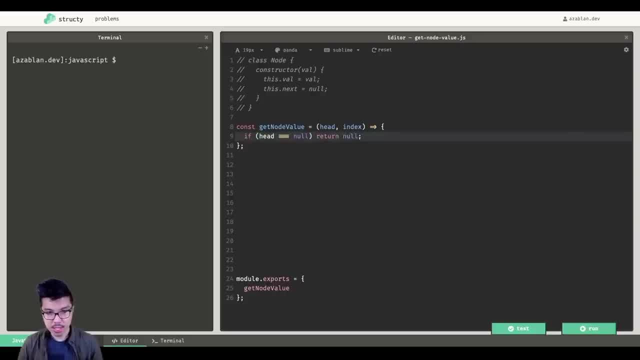 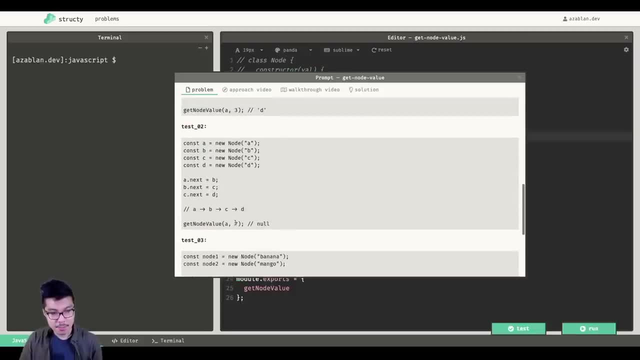 should do is just return. No, that will actually cover a few scenarios. If I look at the examples here, sometimes we may actually get past a very, very large index. So notice: here they're asking for the value at index seven, but the link lists only has four. 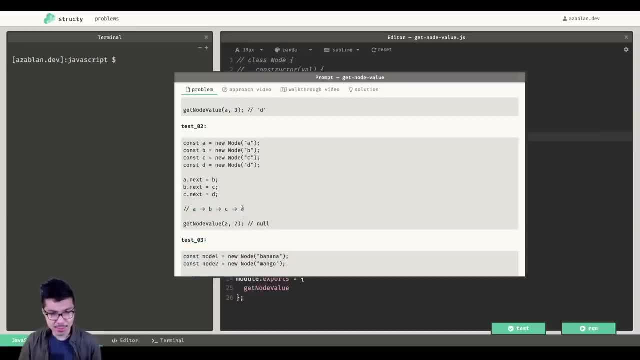 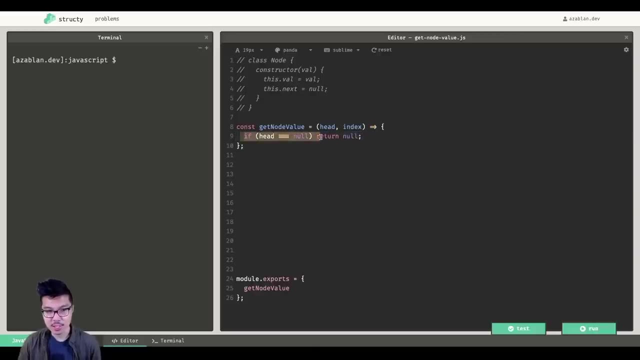 different nodes. that means the index of the last node, D, would be 30123.. So if ever our target index is out of range, then we should just return null, And so this should help me satisfy that, because I'm going to return null once I fall off the edge of the link list. Nice, We're gonna need. 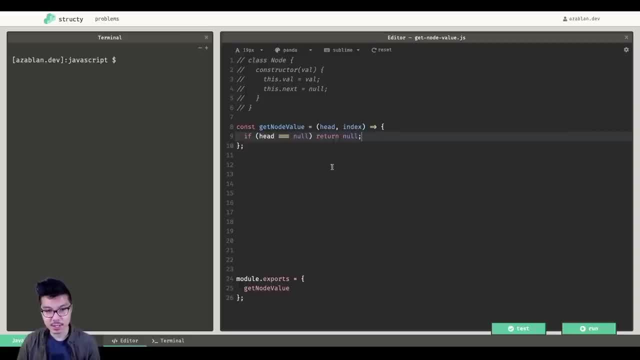 another base case: what if we actually find the particular node that we need to return its value for? So I know over time I'm going to decrement my index, like we said in the approach, so I can check if my index is equal to zero, then simply return this current node, the current node. 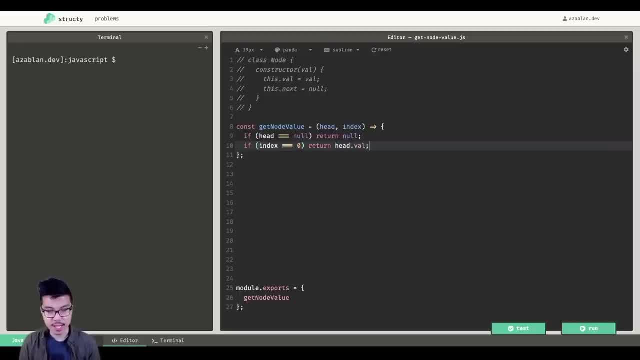 would be head dot Val right, returning its value. Nice. So bear in mind, we're counting down here, And so in my recursive code I need to call my function get node value, pass along the next node of the link lists and then pass along index minus one, And I know that this call is going to return. 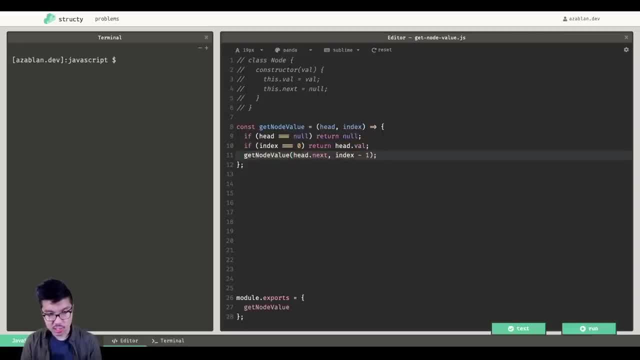 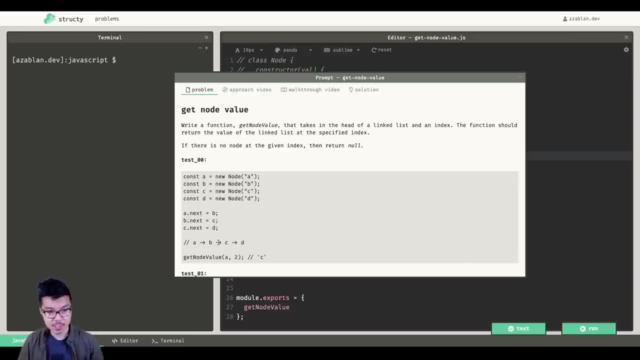 the value of the node at the given value, an index. So I should just return whatever that comes back, as If I do a quick Sandy check here. bear in mind we're counting downward. So for like this example- example 00, we know. 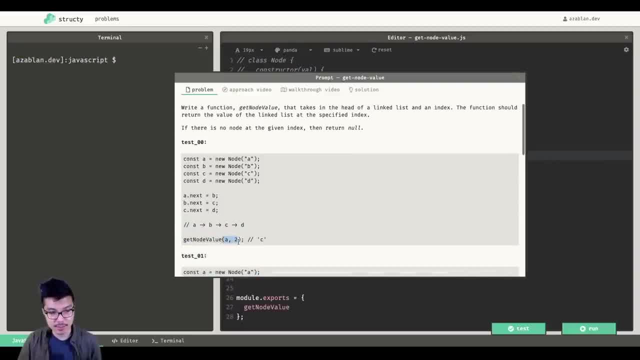 that a is going to have an index of two- right technically, because we're going downward- And when I make the call for B, it's going to receive index one. when I call on C, C is going to receive index zero, which means I should just return that back up the stack. 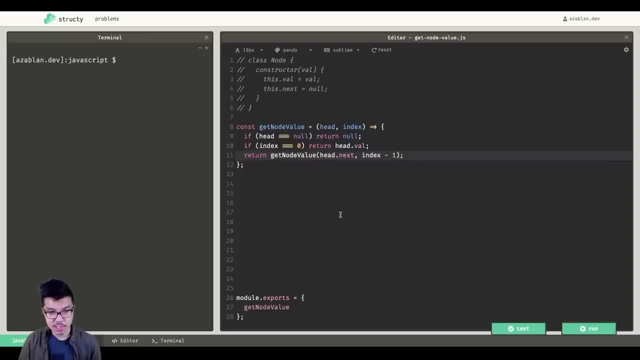 So kind of counting downwards here in the reverse. But this should be a nice solution. Let's give this a test run. Bear in mind that this solution has a linear time complexity and also a linear space complexity. we can actually cut down on the space if we write. 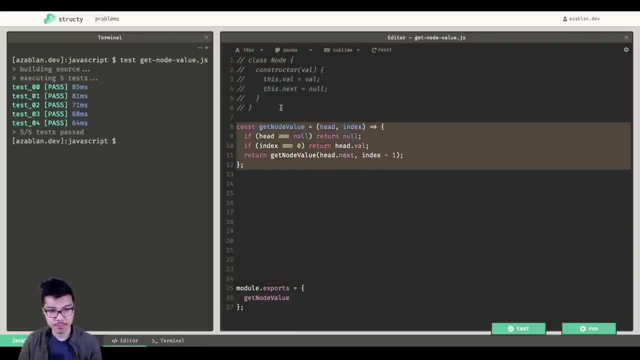 the iterative version, So we'll show you that right now. So the iterative translation you should be very familiar with, probably wondering why are we doing such simple problems? Well, it's about to get more difficult right. To me, it's all about the foundations, So our 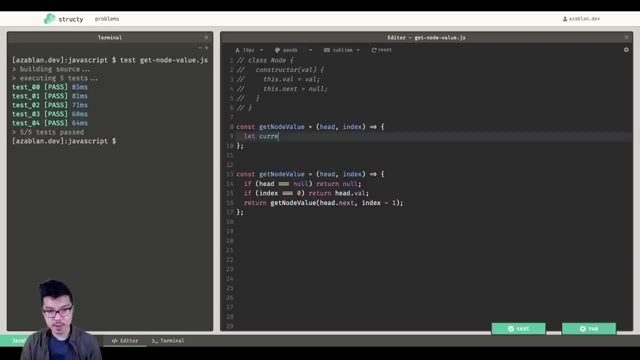 classic strategy is: is for iterations. set your current variable to be the head node right, And I'll just lay out the classic traversal. So while my current is not equal to null, then keep on going To progress to the next node, the sequence. what I should do is set current equal to current. 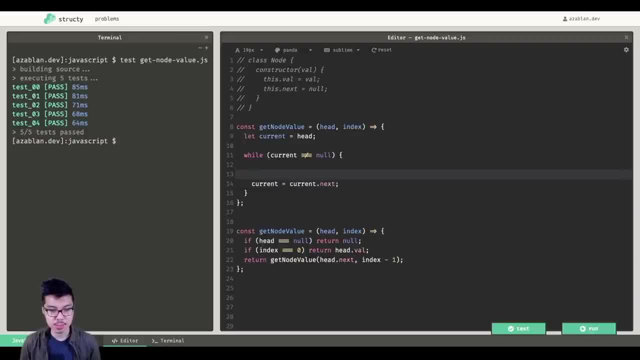 dot next. And now I need to work in the problem. specific logic here. right, I know I want to return the node at the given index And for these iterative patterns, all counts upwards, I'll set some count variable equal to zero, just like this. And whenever I progress to the next, 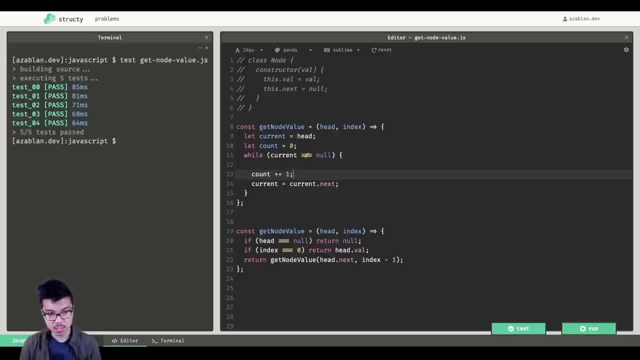 node of the linkless I'll set: count plus equals one. so I'm counting upward. So when I get to some point when my counts is equal to my target index, then I can just return this node right, So I could return this nodes value. So again, we're counting upward in. 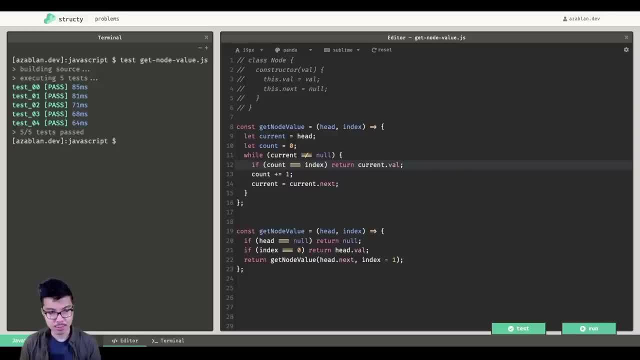 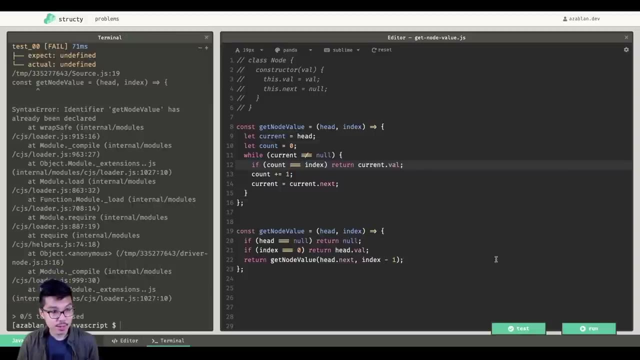 the iterative version, whereas in the recursive version we counted downward. nice, whatever, Let's go ahead and run this code. There was one thing that probably won't pass, but we'll give it a go, See what happens. So I'm getting a little error here. get node value has already. 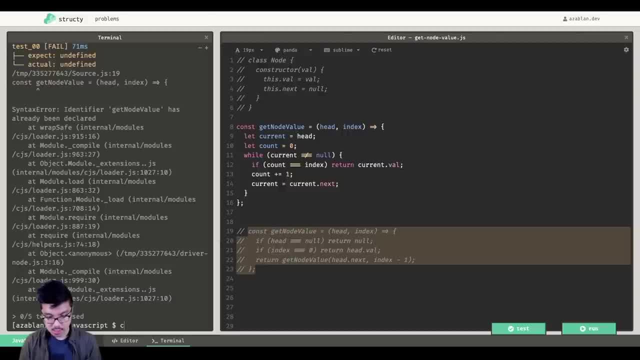 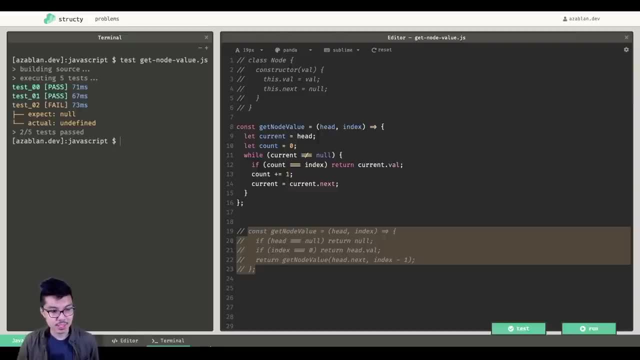 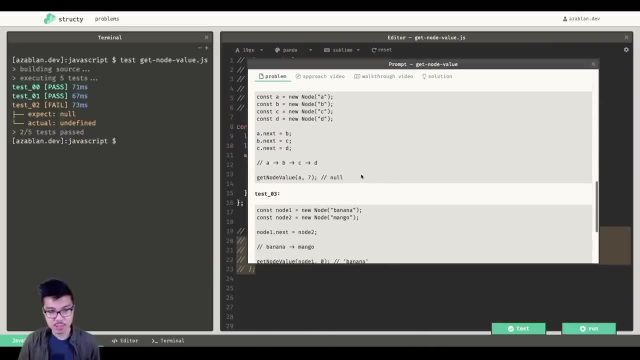 been declared, because of course I haven't defined twice, So we'll try that again. can't read declare your const variables, So we'll run it And we're failing test 02, which is the test where our index or a target index is too large. So here's 02.. So we should have. 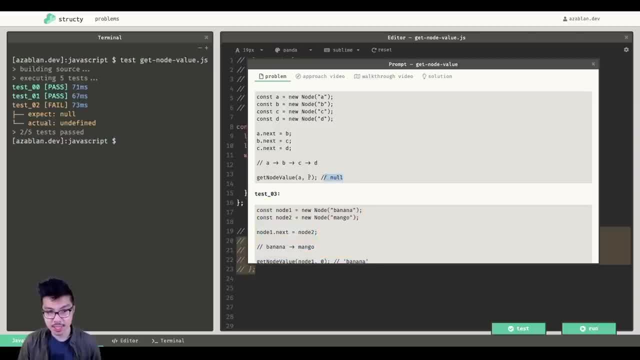 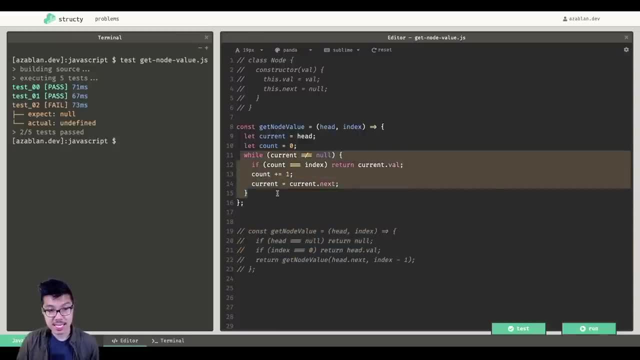 our function return null If we can't find the node at the specified index. right now we're returning undefined, which is happening because this while loop is actually ending right. we're going to hit the very, very tail of our link lists And so our while loops. 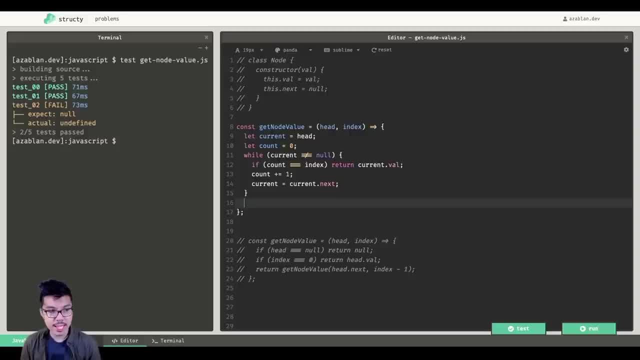 over and we're just going to hit line 16.. When we fall off the edge of our function evaluation, we're just going to by default return undefined. So to fix this it's quite straightforward: just by default return null. And that should satisfy that scenario. Let's. 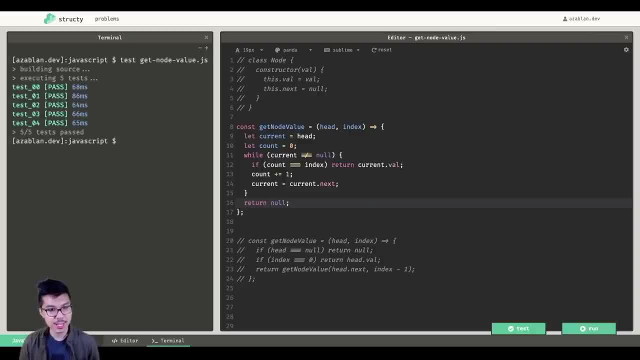 give it a run there, Cool, And there we have an iterative solution. So for this iterative solution, it has a linear time complexity, just like the recursion, but it has a better space complexity. right here we consider this constant space because we only use a handful. 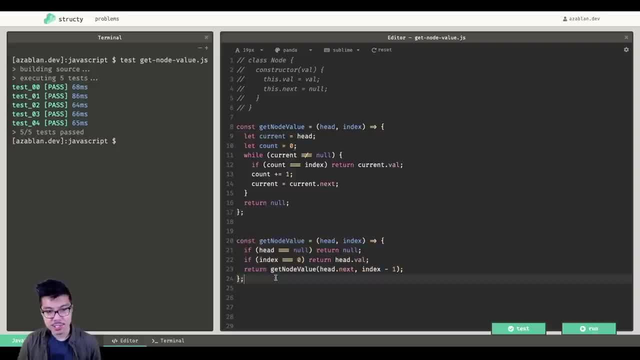 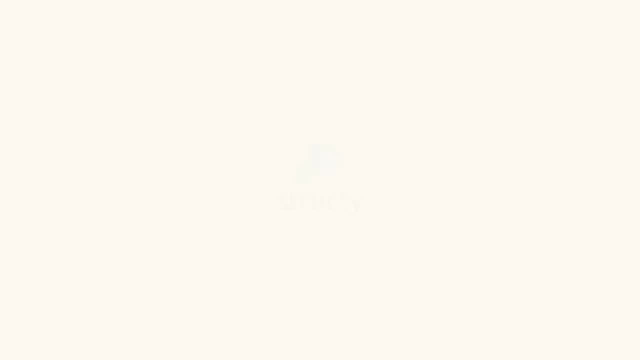 of variables like current and count. That being said, what I want you to do is practice both of these implementations, Because in the next few problems we're going to be looking at how we're going to implement these problems. it's going to get a little more involved. I'll see you there, Hey programmers. 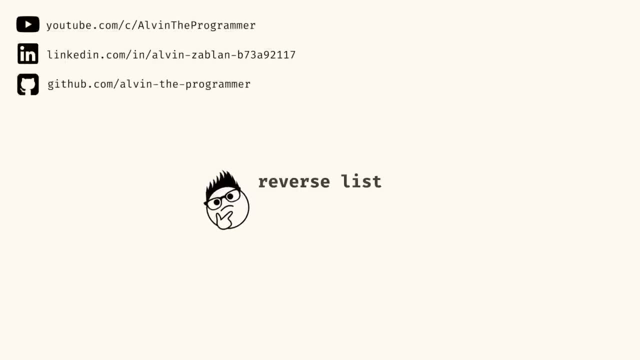 welcome back. Right now let's go over an approach we can use for this reverse list problem. So in this problem we're going to take in a link list as input. what we want to do here is actually reverse the order of the nodes in this link list. So if our input list contains: 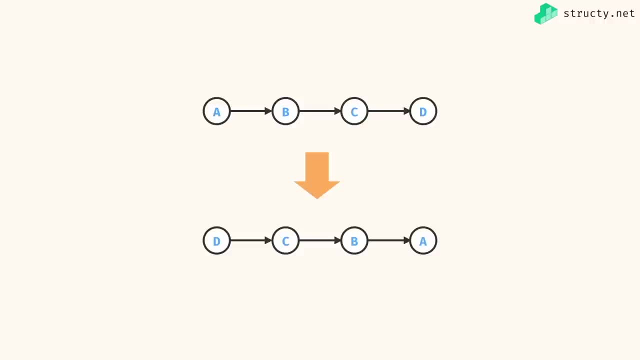 the values ABCD in place, meaning we want to mutate now the existing link list in place. we want to actually change the order to DCBA, Just ending up with the link lists in reverse order In this function. what we should do. 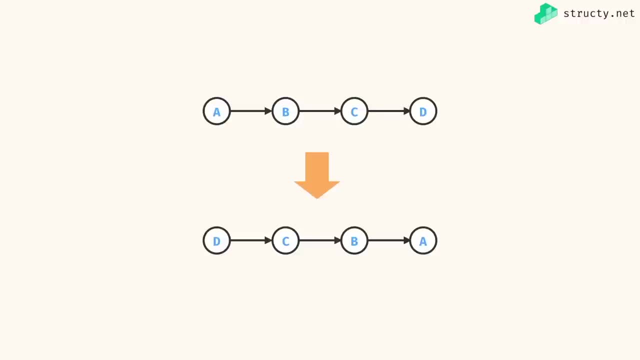 is also return the new head of the link list. So technically, your function for this input should return the D node. So let's come up with a strategy we can use to solve this one. When it comes to the tools we can use for a link list, we know more or less. we always. 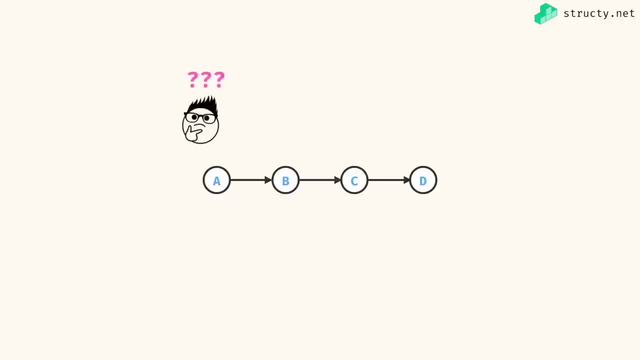 have to iterate or traverse a through the entire link list And we know that that requires at least one pointer. Typically we call it current. The trick here is to actually use multiple variables. So let's say I began my classic current pointer pointing at the 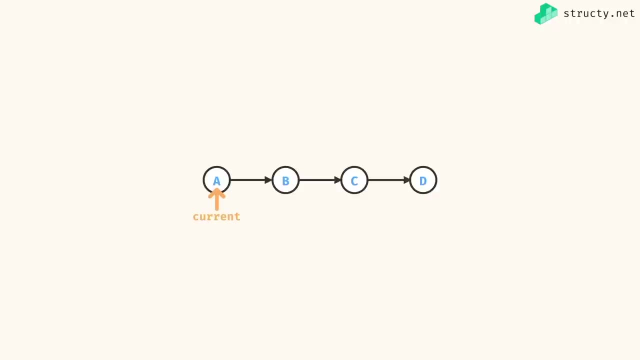 head of the link list. What I'll also need is to track the previous node I visited At the start, because I haven't visited any other nodes. we can make this previous pointer point to null And we know this entire time. if I have access to current, I also have access. 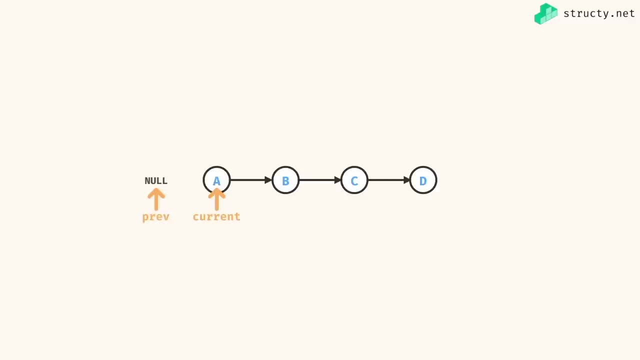 to the next node in the list right by just accessing current dot. next, we're just going to label that as a temporary variable here. Next- and you'll see why in a little bit. So I know I need to have the long term effect. 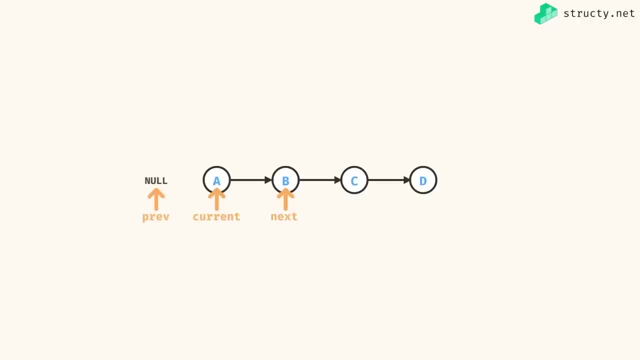 of just reversing all of the next pointers in this link lists. In other words, I need to make a point to null, And so what I can do is literally just set current dot next, in other words, setting the arrow to point to previous. ending up with this. Now it should. 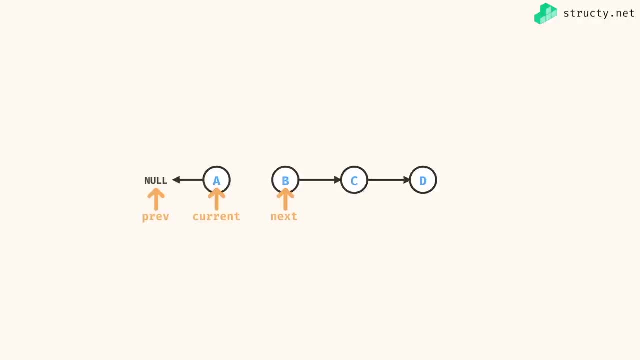 be abundantly clear why we save the B node with that next variable: because once we reroute currents dot next to point to null, we would lose access. So what I can do now is shift my point of view. I can set my current to be the next. 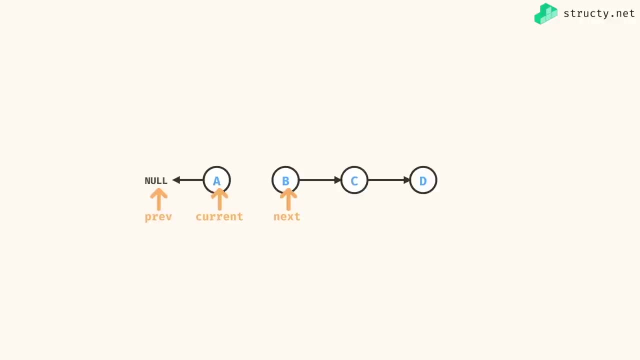 and set my previous to be the old current, just shifting my point of view like this. And now I can set current dot next to be the previous node, once again rerouting this pointer. And this process continues As we get toward the end of the linkless. we have to also remember 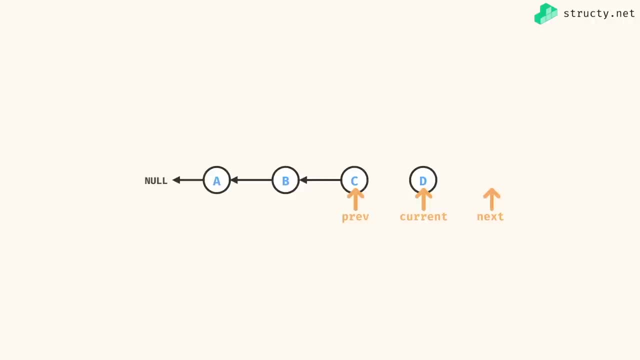 is technically, since D is the old tail of the linkless this entire time it actually did have a next pointer, just happened to point To null, And so at this point I can actually continue my general algorithm. right, I still. 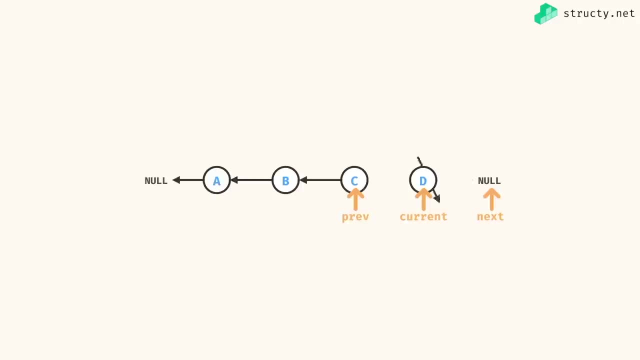 set current dot next to my previous rerouting this pointer- and I can actually continue one more iteration If I set current to be the next. it's now the case that current is actually at null, which means we hit the end of our linkless and we can stop our algorithm. 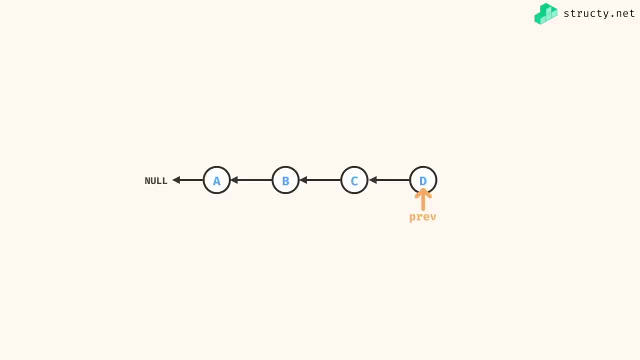 If we look at the current state of our linkless, it is in reverse order: right D points to C, points to B, points to A, points to null. So I can actually return the current value of the linkless And if I want to return the 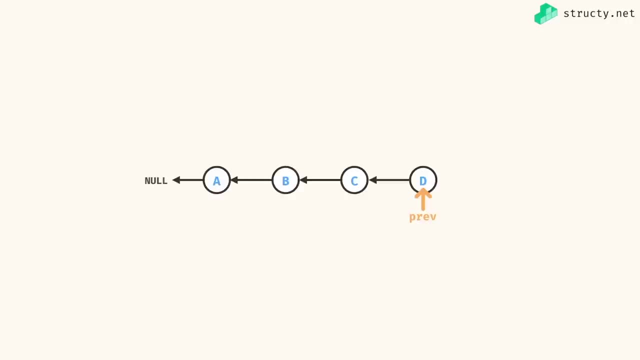 new head of the linkless, I can simply return the final value of the previous variable. So that actually works out pretty elegant If we do the analysis for this algorithm, if we implement this in an iterative way and we say n is the number of nodes we know. 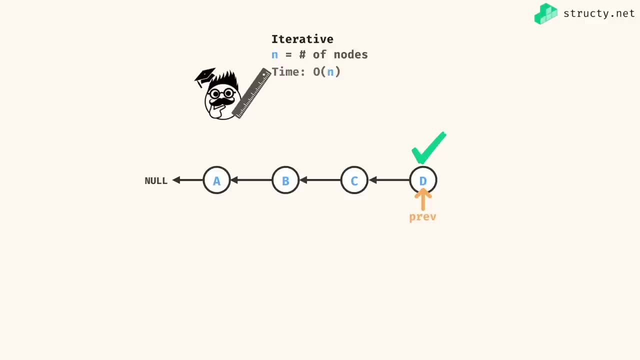 that the runtime is just going to be O of n really just traversing through the entire linkless, once we can say that space complexity is constant because we only need a fixed number of variables. So overall this is a maximum efficient algorithm To reverse a linkless. when we go on to the code walkthrough for this I'll actually show. 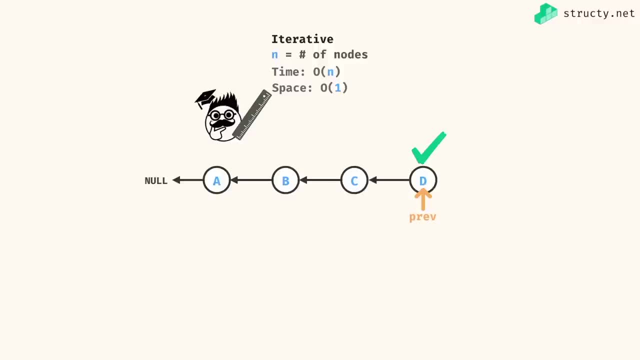 you how to implement this iteratively and recursively, bearing in mind that the recursive would actually suffer a slightly worse space complexity. But before we get there, try to give this a shot on your own. implement this. If you get stuck, I'll catch you in the walkthrough. 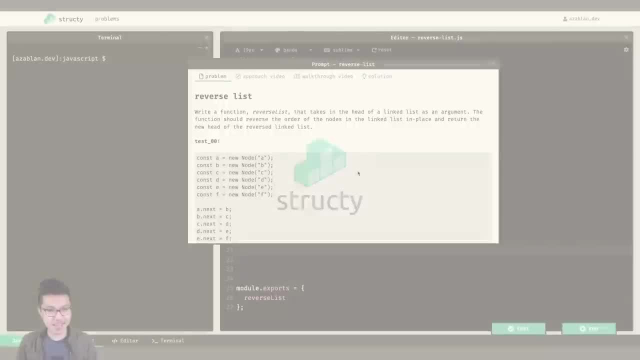 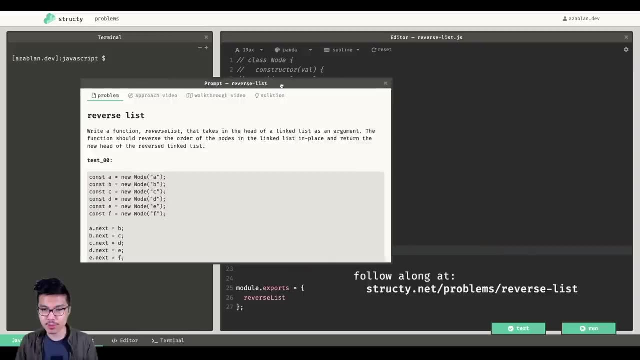 video. See you there. Hey programmers, welcome back. right now I want to go over a JavaScript solution we can use for this reverse list problem. So if we already watched the approach video, if not, I highly recommend it, Because we're going to implement that strategy pretty closely. So I'll start with the iterative. 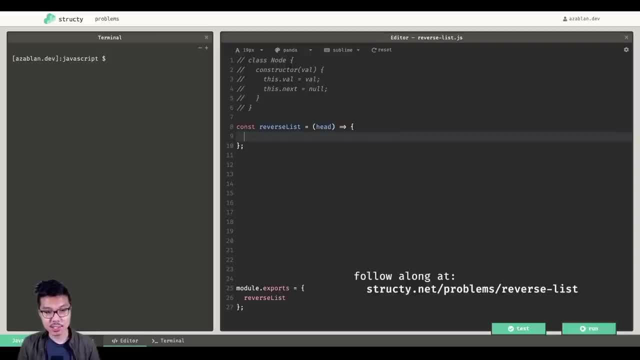 version here And we know we just need to lay down, at least initially, our classic linkless traversal. So we're just going to keep my current variable, initialize that to head and loop, while my current is not equal to null And I know that the basic code would always. 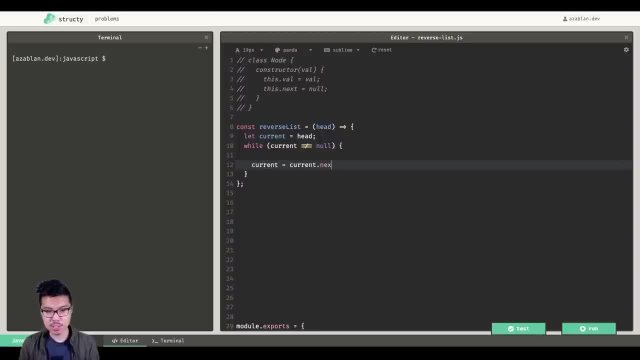 be set current, equal to current dot. next, that would just move sequentially through the linkless. But now we need to work in a few other variables, right? So the key here is to have some variable- we'll call it previous- and to initialize it equal to null. And if 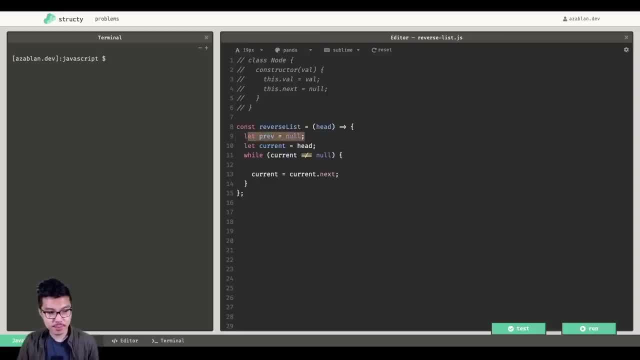 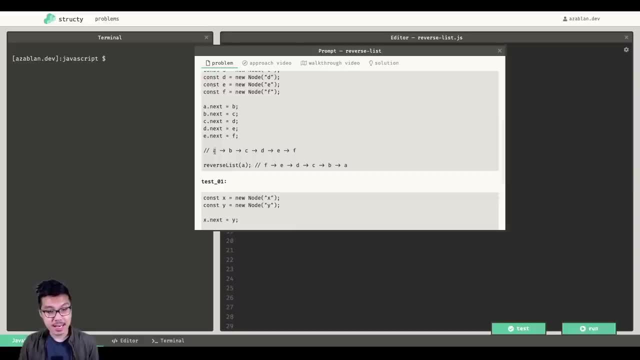 we were wondering why null is a great default value for this previous. just think about what needs to happen on the very, very first iteration of our while loop. So we know that our current is going to be a and in the long run we know a's next needs to actually point. 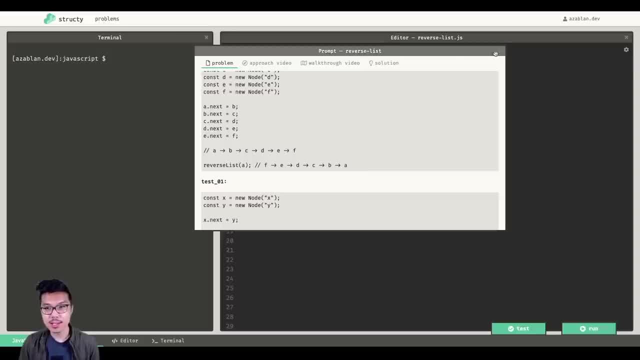 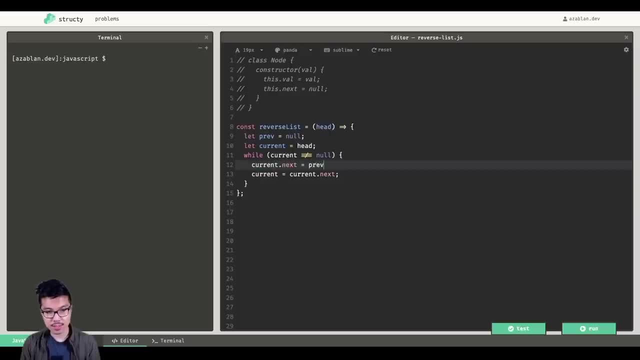 to null right because it needs to become the tail. So if we initialize previous with null on the first iteration, we can immediately just say current dot. next, equal to null equals previous right. that would actually have that arrow point to null, which is good to go. 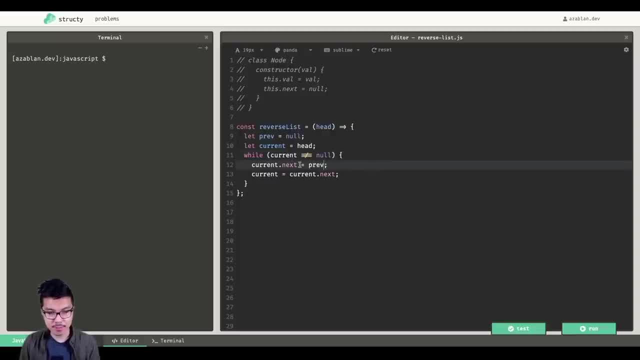 But then at this point we need to make sure that we have some proper references here. So before we just reassign current dot next, if we just overwrote it willy nilly, then we would lose access to whatever the actual next note sequentially was. So I'll save that to a variable. 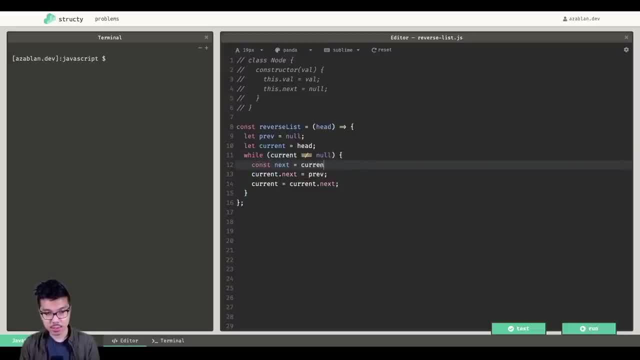 I'll say maybe const next equals current, dot next, And then, after I overwrite it, I can still make progress to the next note of the link lists by simply setting current equal to next. Awesome, So that's looking pretty good, And not only do I need to progress: current. 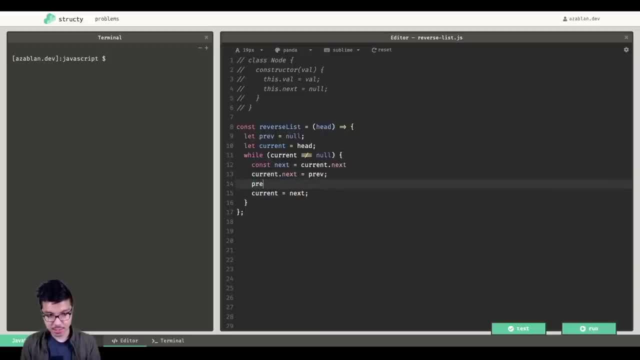 but previous should now also point to current, shifting my full point of view. So some pretty tricky logic over here. Let's go ahead and maybe analyze a little bit closer What it's doing. please mask your here. So let's say we had a link list that looked like this: 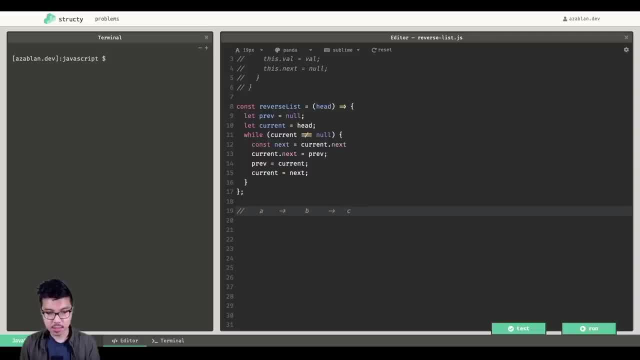 a points to B. points to C. we know we have initially current over here, right, so current is pointing to a. we know that when I save that next variable it's going to point to this B over here. So I'll save that And technically, at the very start we initialized: 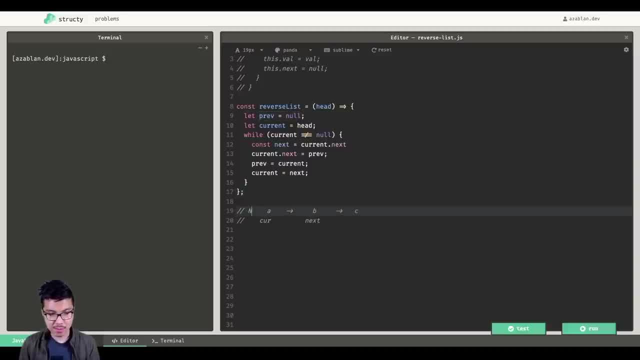 previous to be null. So I'll just use like capital N represent null And I know previous is going to point to that like this: Awesome. So on the first iteration we have all these variables set up and I set current dot next equal to previous. current dot next is represented by this arrow. 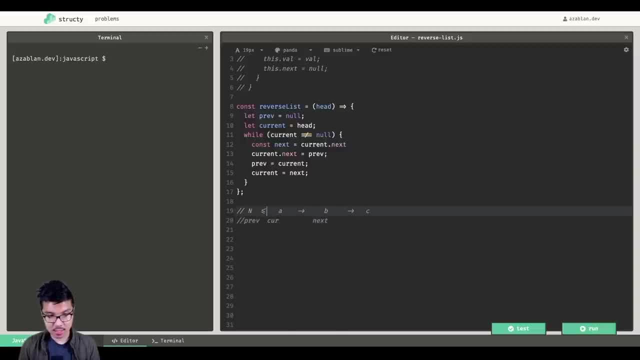 So when I set current dot next to be previous, it has this visual representation right, just setting it the opposite direction. And once I do that would actually lose this arrow. And now you can probably see why we saved next for B right. That way I don't lose access to the rest. 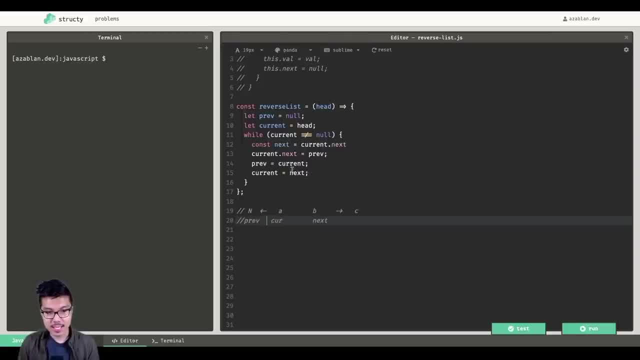 of the link list. Cool, At this point I can set some variables right. I can make previous the current, So I'll set it like this. Then I also set current to the next. So basically, just shift over the point of view. And if you look at the state of my drawing now, things are actually perfectly. 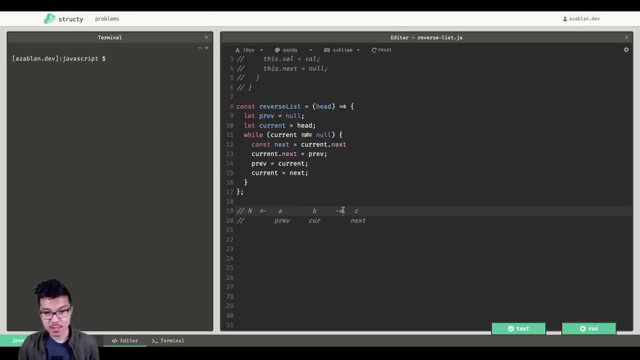 aligned for the next iteration. I would just set current dot next to be previous once again, and so on and so forth all the way through the very end of the link list, And we set in the approach once we actually end, when current is equal to null, you exit the while loop. 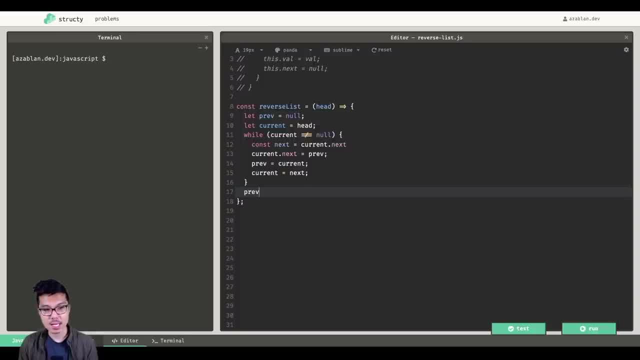 and previous would actually contain the new head of the linkless, So I'm just going to return previous over here. it does make sense that previous would be the new head of the link list Because after I exit the while loop I know previous is going to be. 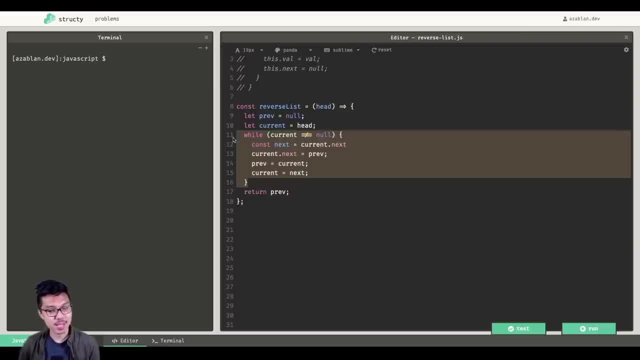 the original tail right, And if I'm reversing, the tail becomes a head and vice versa. Cool, So really just a spin off of our classic linkless traversal. I will tell you that the logic here it can get pretty tricky, especially with these temporary variables. So we'll give it a test run. 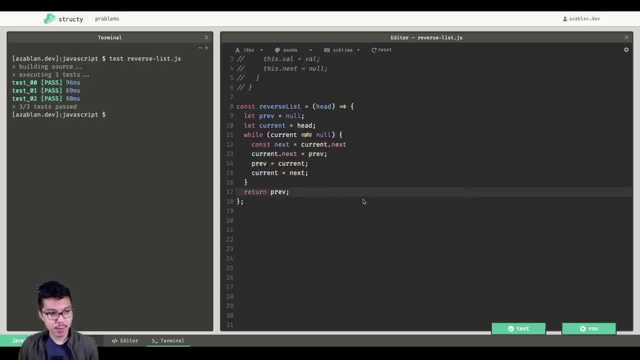 see what we get, And hopefully we'll have this nice O of n runtime O of one space solution. Awesome, there we have it, And so what I'll also do now is show you the recursive version. it will have a slightly worse space complexity, although the code is. 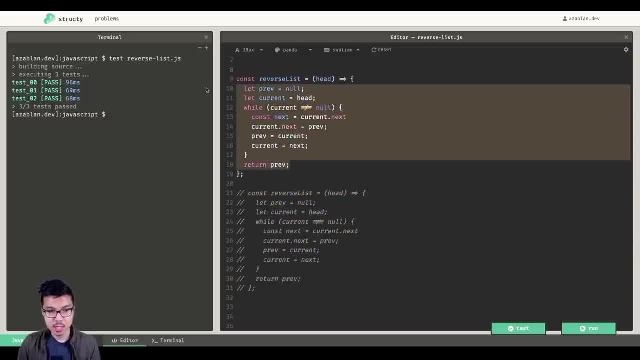 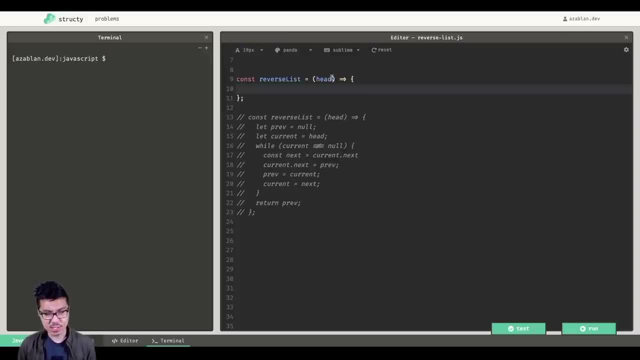 noticeably more concise, So I think it's still worth practicing. So, really, we're just going to translate the same premise into its recursive version, right? So you know, I'm going to still need, like, access to two variables or two pointers, And the way I established 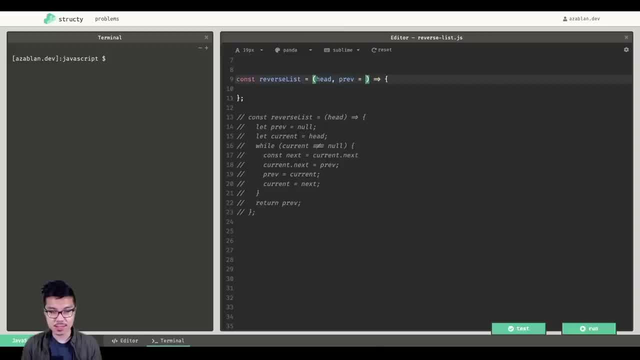 that recursively is by using a default argument here. So I'll set previous equal to null. So if you're unfamiliar in JavaScript, this is how you just do a default argument, right? So if someone does not pass in a second argument when they call reverse list, by default it's going to be set to. 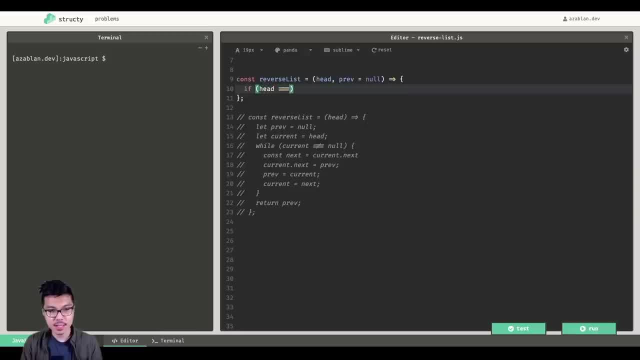 null And I can start with a classic base case. right? If head is null, then I've hit the end of my link list And what I can do is actually just return previous. For the same reason I returned previous over here. right, previous would actually be the new tail. 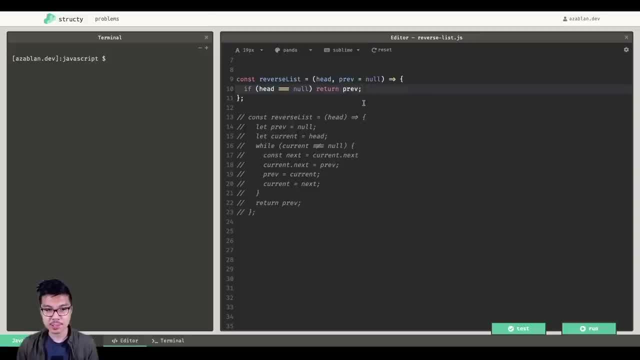 And when it comes to actually writing the recursive code, I'm just going to try my best to translate all of these iterative patterns into their recursive analogs. So I'm going to save a reference to the head next, just in a temporary variable, Because if I overwrite it by saying head, 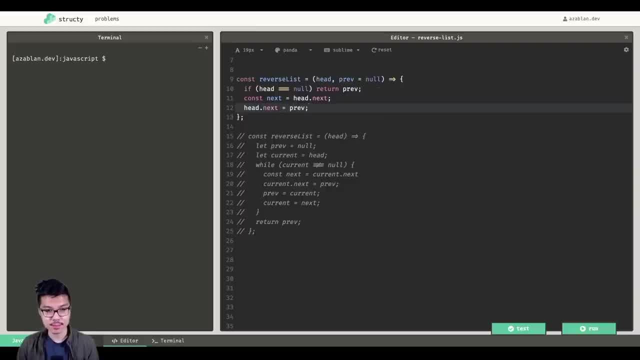 dot next equals previous. I would lose access to it otherwise. So now I at least have a way to call recursively and traverse through the rest. So I'm going to just call it, do this, And then I'm going to call the new list of the link list. So 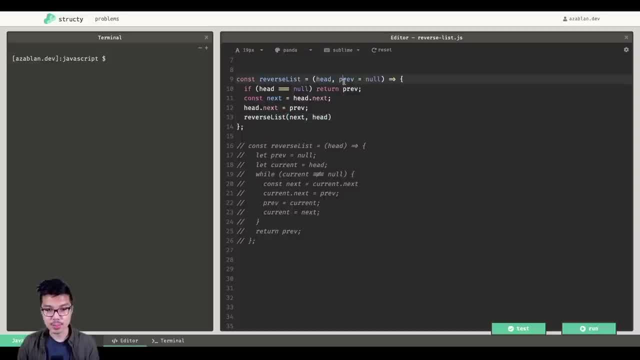 pass in next as the new head and pass in head as the new previous, really just shifting that point of view. Once again, I think about the return value for reverse list. I know it's going to return a node right. it's going to return, hopefully, the new head of the link list, So I just want to pass. 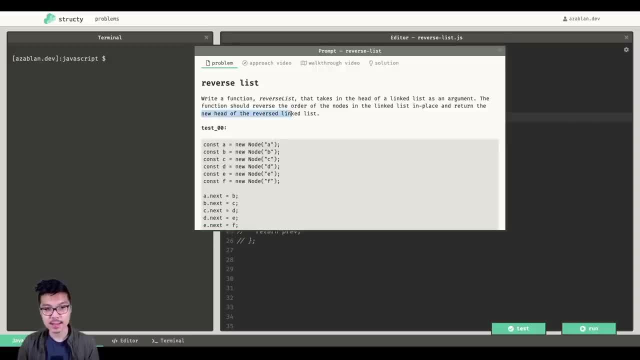 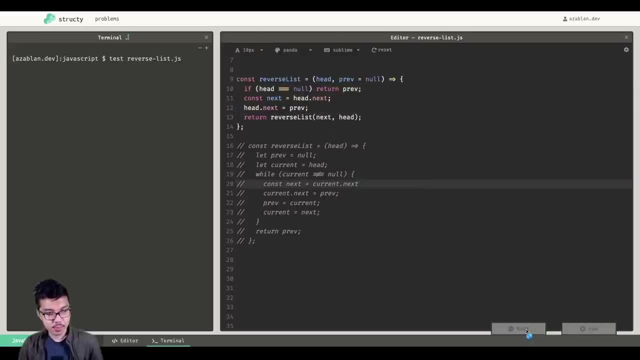 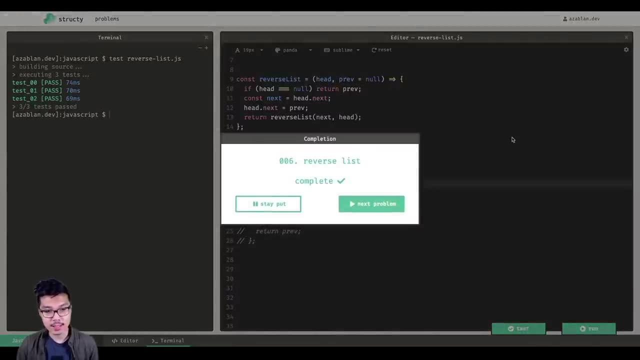 up that return value. Do stay aware in this problem. they say your function should return the new head. satisfy that. So we'll give this a run. Nice, And here we have a O of n time recursive solution that is also O of n space, right? So apples to apples comparison if you wanted to get the most. 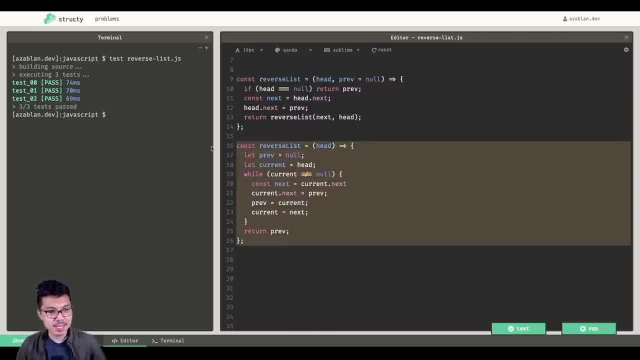 efficiency, you should prefer the iterative version. That being said, I still think there's a nice value to practicing both of these, And this is actually a pretty common interview problem, So make sure you have this down pat before we hop into the next problem. I'll see you there. 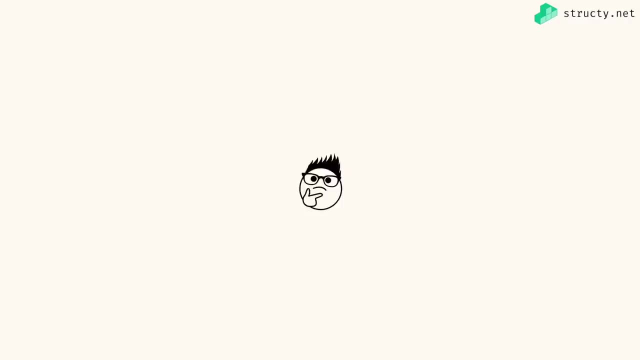 Hey, programmers, Alvin here. Right now I want to go over the approach we can use for the zipper lists problem. So in this problem we're going to take in two link lists. what I want to do is zipper these two lists together. In other words, I need to, in place, reassign all of these. next. 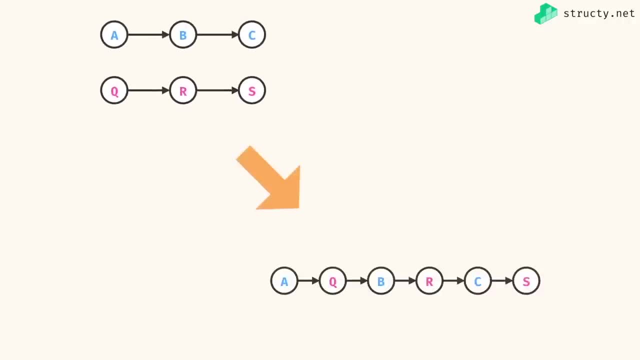 pointers such that we alternate between the nodes of list one and list two, And also looks like we should always start with the first node of list one And then, from that point on, simply alternate. That being said, let's take a look at another example. 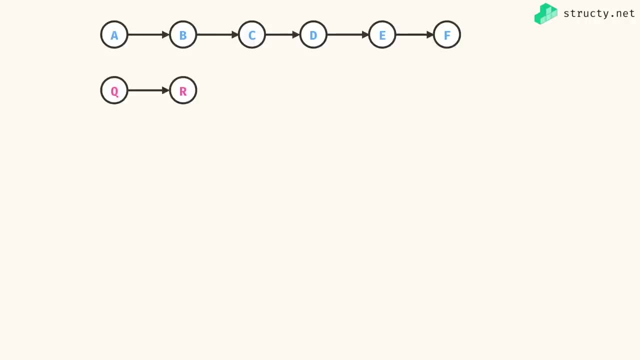 We don't have many assumptions we can use when it comes to the lengths of both of our lists, except that we know that each list is actually not empty. But besides that, what if one of my lists was longer than the other? Well then, what I want to do is alternate as much as I can. 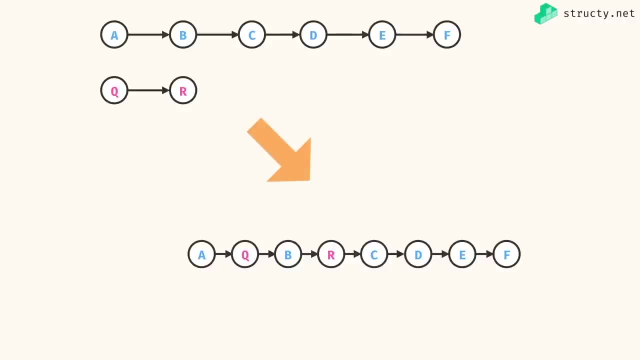 and then just terminate the link lists with the remaining nodes. So notice, I alternate with a qbr at which point I don't have any more nodes in list two, So I just take all the remaining nodes of list one and add them to the very end. 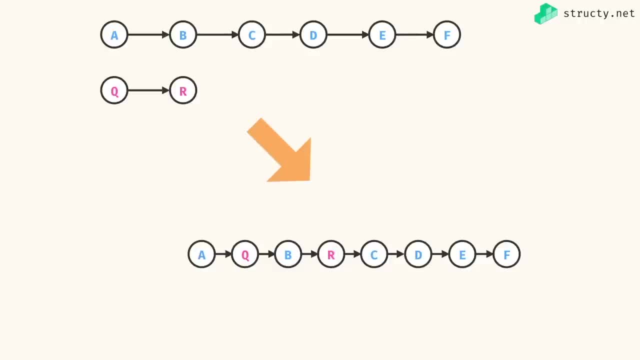 And so we'll want to keep that edge case in mind when we come up with a strategy for this one. So where do we even start with a problem like this? Well, you should be familiar with our core linkless pattern, right? We just know how to traverse sequentially through a linkless And. 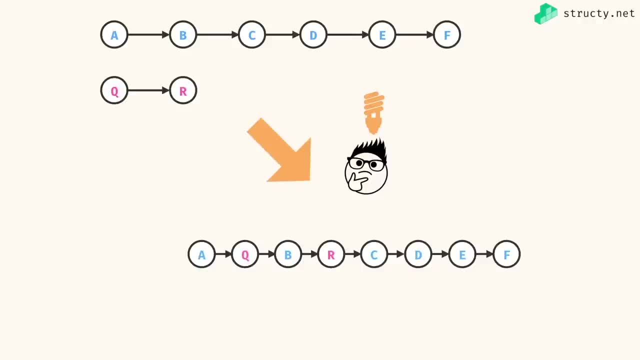 so what I can do is actually maintain two pointers at a time right, One for list one and another for list two. So let's say we started stepping through this example. I know I'm past both of these head nodes- head one and head two respectively- And then from there I can set up. 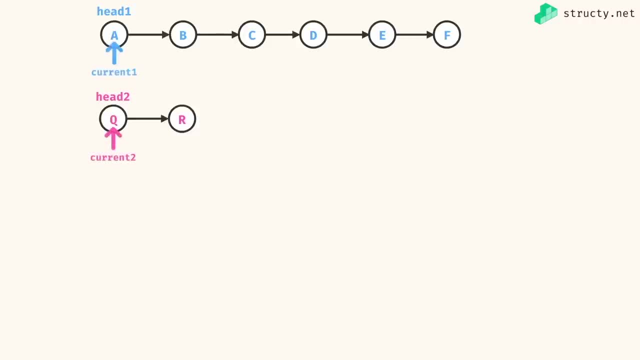 some respective current pointers And so, given in the examples, we always want to start with the head node of list one. So I'm just going to start that down here, And what I'll need to do is also track the tail of my output list. right, Although we're just reassigning all of our pointers in. 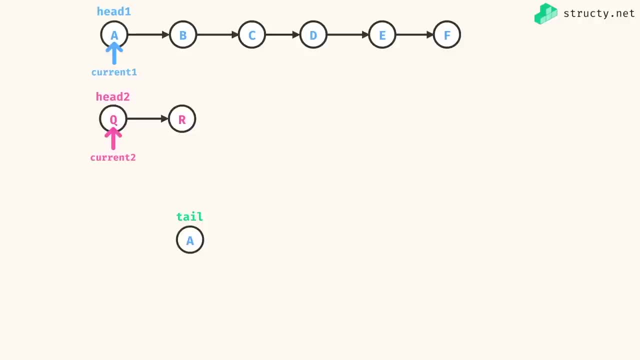 place. we're going to need a reference that way we can figure out how we can add new nodes to our current output. we'll say, And since I already begin my chain with this, we're going to need to add new nodes to our current output. we'll say, And since I already begin my chain with this, we're. 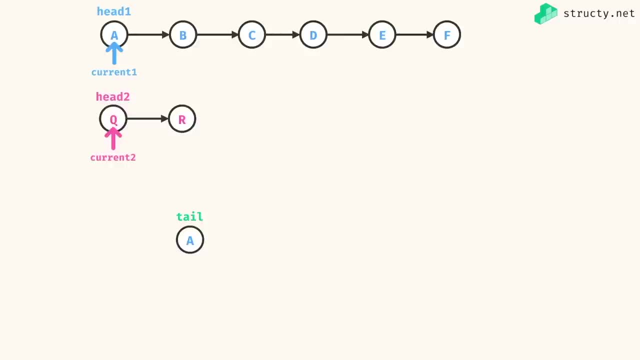 going to need to add new nodes to our current output. we'll say: And since I already begin my chain with this, we're going to need to add new nodes to our current output. we'll say: And so first node of list one, then I need to be sure that I actually progress- current one, And so 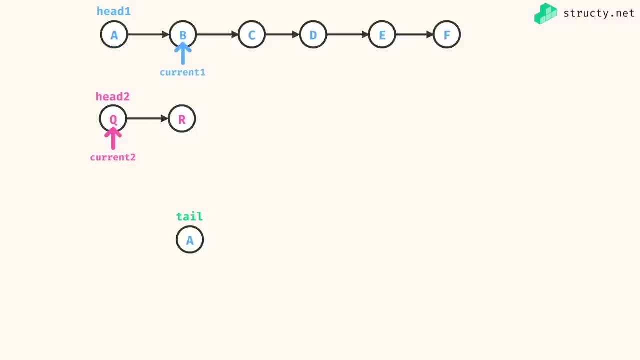 current one should really be pointing at this B node. And so, now that I have at least a starting node, how can I come up with a general algorithm here? Well, if you want to establish a simple alternating pattern, then what you can do is just use a counter variable, have it start at zero. 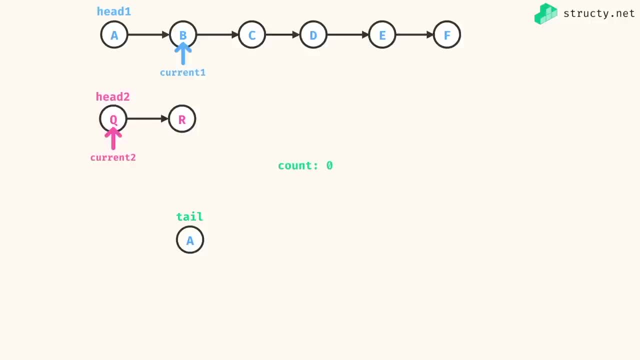 And then, based on whether or not the count is even or odd, that would tell you from which list you should take your next node. And so, since I already begin my chain with this, we're going to need to begin with a node from list one. what I should do is, whenever my count is even, I'm going to grab a. 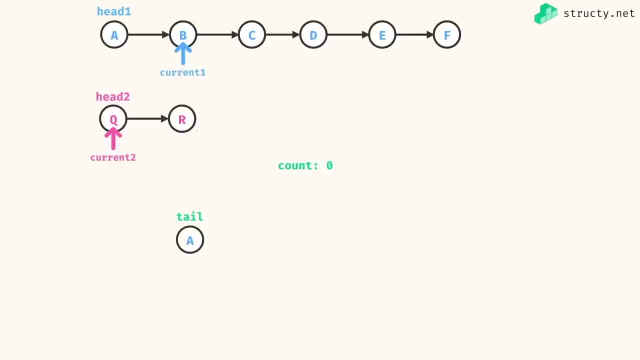 node from list two. when count is odd, I'm going to grab a node from list one. So right now, count to zero. zero is technically an even number, And so I'm going to take my next node from list two. So I look at my current two pointer and it tells me I should just take that Q node and add it as: 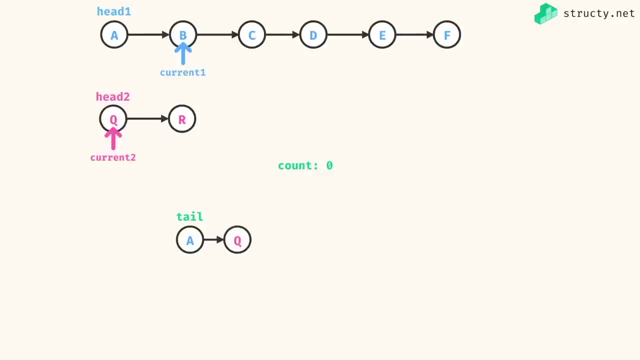 the next of my tail, And so now that I've consumed a node from list two, I need to be sure I progress current two to its next, just like this, And I also need to make progress on some other pointers here. I need to progress my tail also to its next. that way I can get set up for the next iteration. 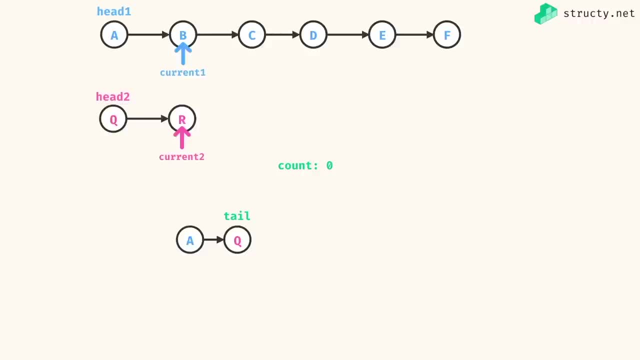 of the algorithm. At this point I need to increment my count by one. So now count is one. Since my count is odd, I should take a node from list one. So I look at my current one pointer and I add B to the tail, just like this, And I make progress on all of my variables, right? 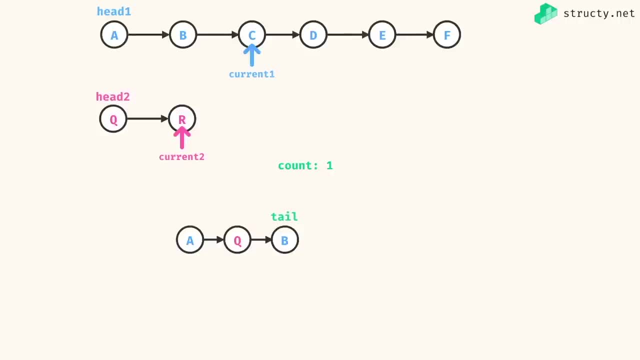 So I'm going to progress current one, I'm going to progress my tail and increment my count to two. Since it's even now, I should take a node from list two. So I take my R from current two And when I set current two to 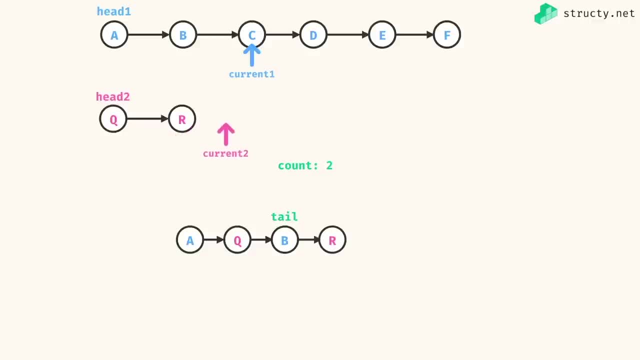 its next, it's going to become null. When I set tail to its next, it's going to be set to the R, And then I increment my count. So now my count is three, And now I have an important scenario. it looks like I've exhausted all of the nodes. in list two. We spoke about this scenario. 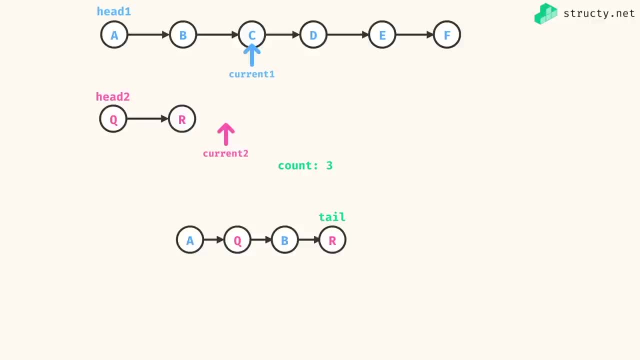 right, Whenever we finish all of the nodes of one of our lists, we should just terminate our output with all the remaining nodes of our other list, the non empty list. And so at this point what I can do is just take my current one, basically this C chain and everything after it. 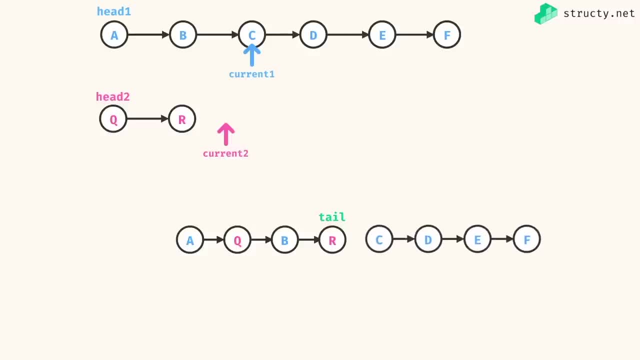 and just put it after the tail and my output, just like this, And of course, I want to complete the connection over here, And this would actually be the correct output. And so, overall, our strategy was to make it a little bit more complex, And so I'm going to take my current one and I'm going to 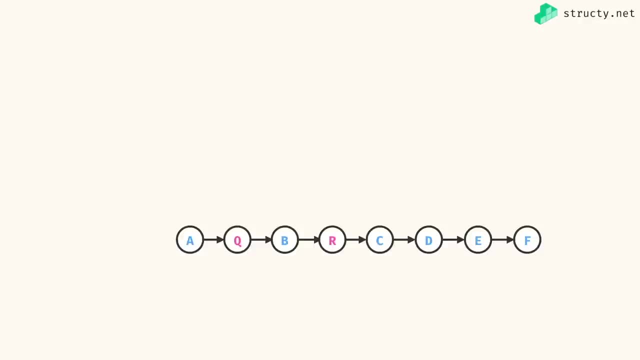 maintain pointers to both of our respective link lists and maintain accounts right. depending on whether the count is even or odd, then that'll tell me from which list I should take my next node. And along with that, we also need to maintain some tail pointer we can use So we can actually build. 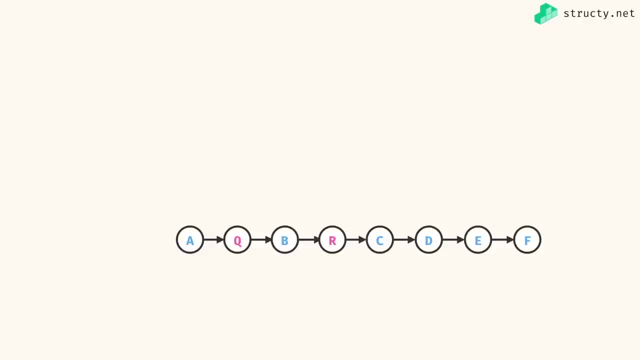 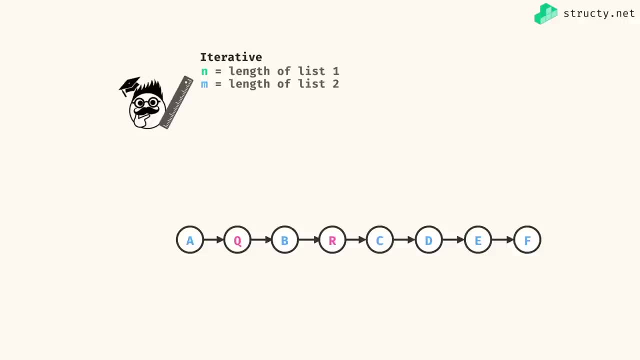 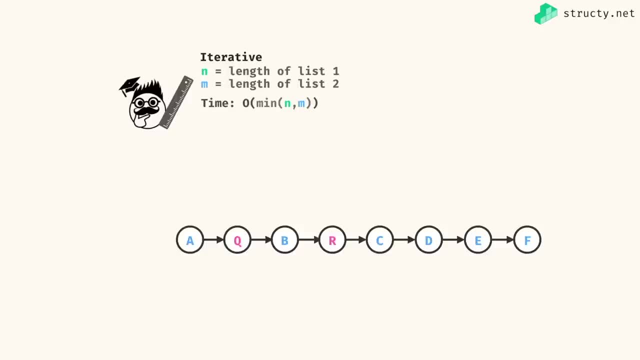 complexity is the minimum between n and M. Recall that when we just step through this algorithm, we really only needed as many iterations as the shorter link lists. Recall the algorithm we just traced through. Now, once we hit the end of one of our link lists, we know we just finished the. 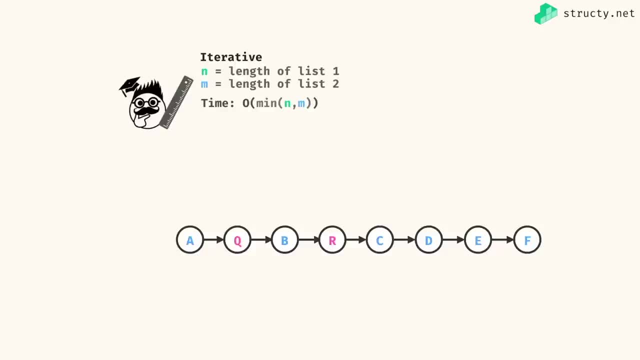 algorithm by taking the remaining nodes of the other list and just tack it on to the end, And that finishing step only takes a O of one time. So really, as soon as one of our link lists runs out, which will always be, in general, the shorter one, then I can just finish my algorithm. I actually don't have to iterate. 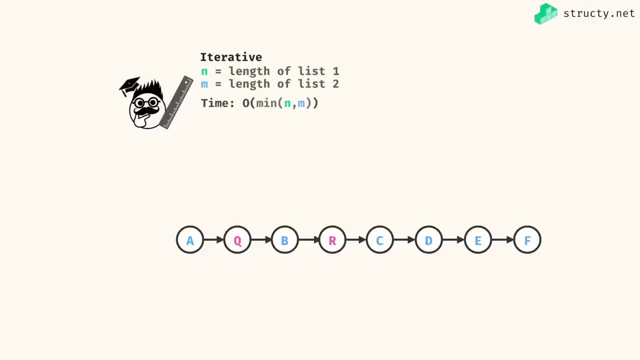 fully through both of them And I would still consider this technically. you know, some form of a linear runtime For the space complexity. we can see how the space here is just constant right. we're not actually creating any new nodes, we're simply rerouting all of these next pointers. 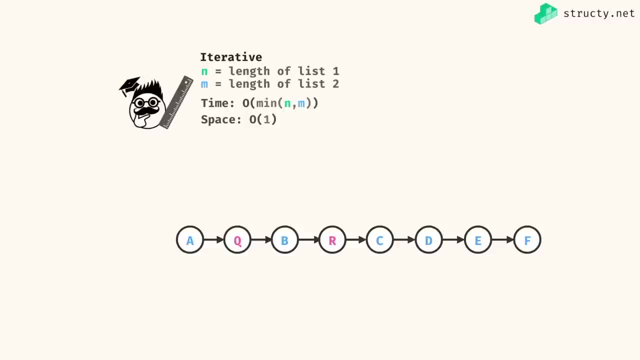 And, in terms of our variables, we only use a fixed number of them, And so, overall, this seems like a reasonable strategy, And what I want you to do is try to code up this one on your own. it's going to be some really interesting code, a new pattern for us, that is, And if you get stuck, I'll catch you. 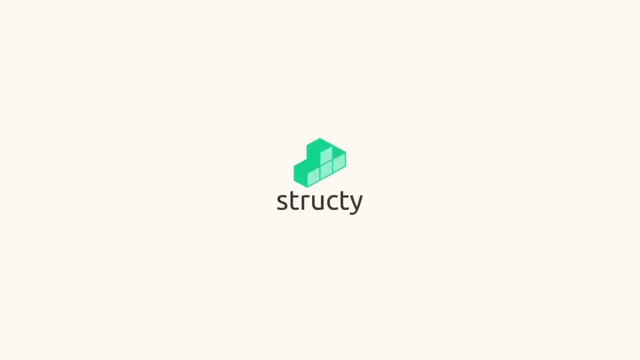 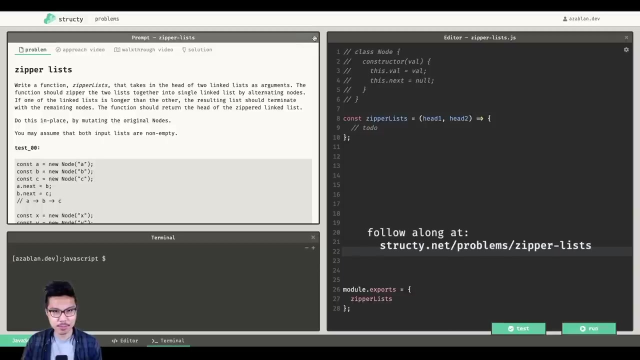 in the walkthrough videos. See you there, Hey programmers. Alan here. right now I want to go over a JavaScript solution for this zipper list problem, So we'll jump right in, hopefully, watch the approach video And we'll start with an iterative version of this. The way we're going. 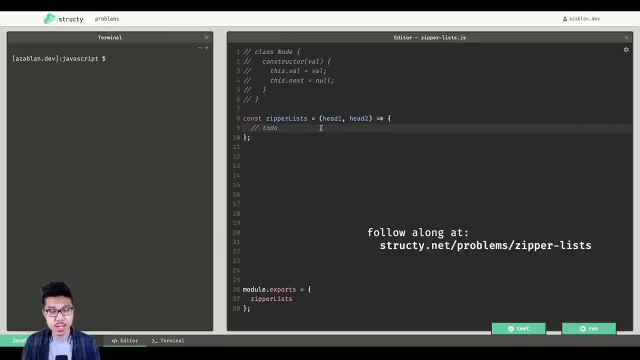 to attack this one is by doing our classic linkless traversal, but do it twice over for a head one and head two simultaneously really. So I'll set my let current one to start at head one And I'll also set let current two to start at head two And I'm going to need my main loop. 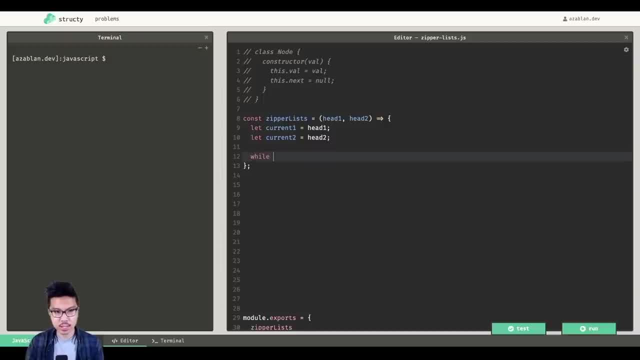 just to iterate through the linkless So I can check, while current one is not null And current two is not at all. So notice, as soon as one of my linkless hits its end, this loop would actually stop. Right, Cool, What we want to be sure to do is set up also a way to create the output. So 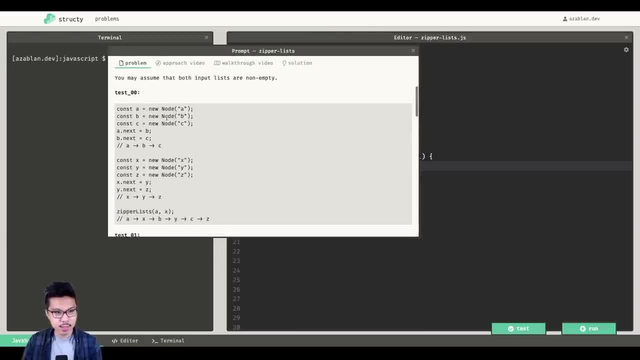 look at the prompt. we always start with the first node of list one. So in this particular example I'm zippering ABC and XYZ. I always start with the A here And when I use that to get the ball rolling on my resulting list. we're not going to create any new nodes, But we do have to rewire. 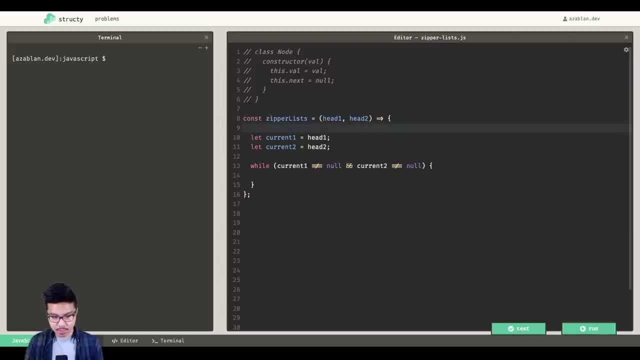 all of these next pointers. So what I'll say is maybe, let's say, head over here must be the head of our output, because I know I need to return that by the end, Something like that. I'm going to start head really as head one technically, and then 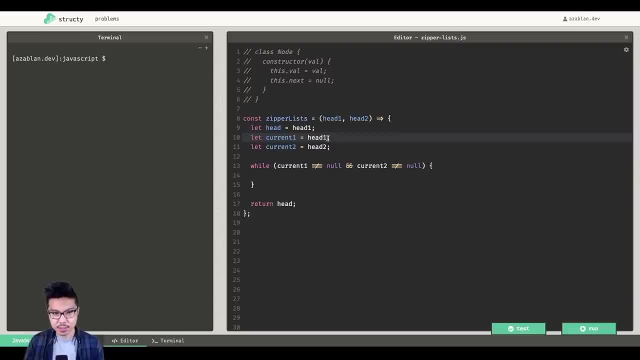 current one will actually have to start one after that, like we said in the approach. So I'll set current one equal to, we'll say, head dot next. that'll be a good starting point from there. And in addition to having this head pointer, that's because I want to return, you know. 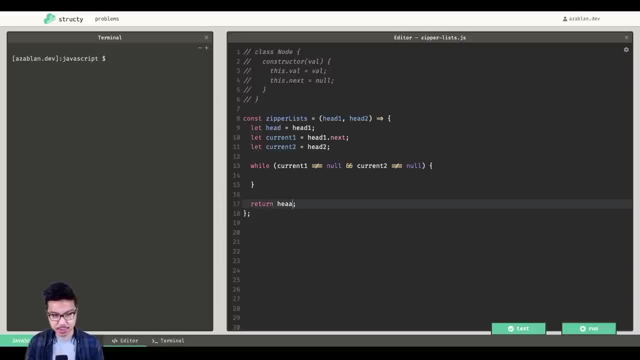 the new head of the link list, which I guess would be the same as head one, now that I think of it. so maybe we don't need this variable, But we do need is a pointer that we can append after right. So I'm going to say: let tail, I think. as a matter of fact, I'm gonna set tail equal to. 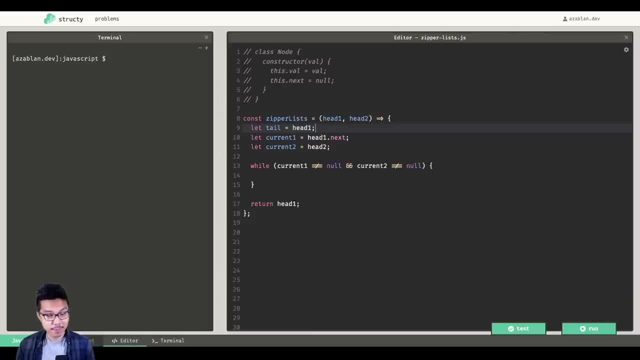 head one. So I know head one is going to be the first node in my output And over time I need to add things after the tail building up my resulting list. So that's looking pretty good. Now we'll go ahead and increment our counter add. 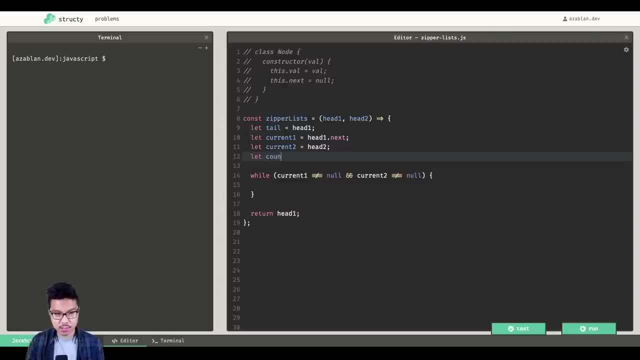 that into the mix here. So we'll say: let's count, begin it at zero And, depending on whether or not our count is even or odd, that can tell me whether I should take a node from list one or list two. So 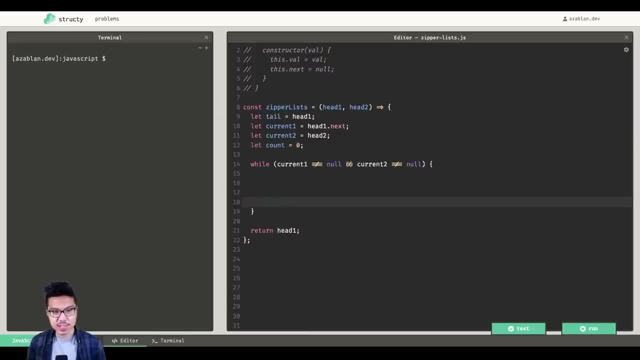 I think we're ready to hop into our main code over here. I know I should end any particular iteration by, of course, incrementing the count right. Count plus equals one. I'm just going to put that down there So I don't forget. And I will start by checking the parity of that count right Whether. 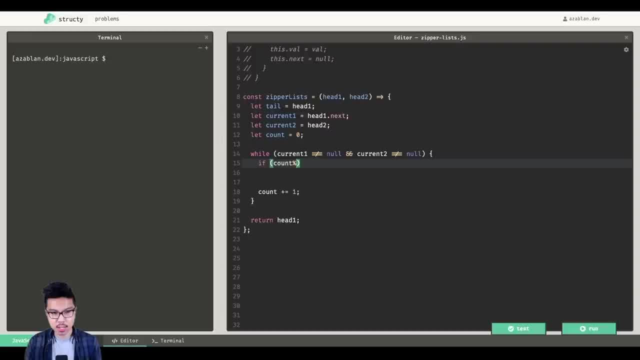 or not. it's even or odd. So I'll simply check. if count mod two is equal to zero, right, So that means it's even then else it's odd. So bear in mind I started my output list with a node from: 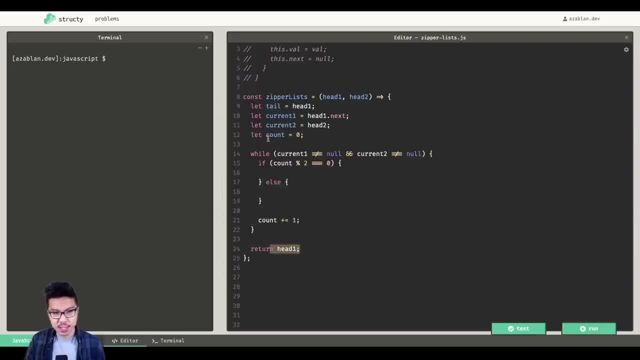 head one from list one, And initially I start my count equal to zero. So I guess when my count is zero, I'm going to start my count equal to zero. So I'm going to start my count equal to zero, So I. 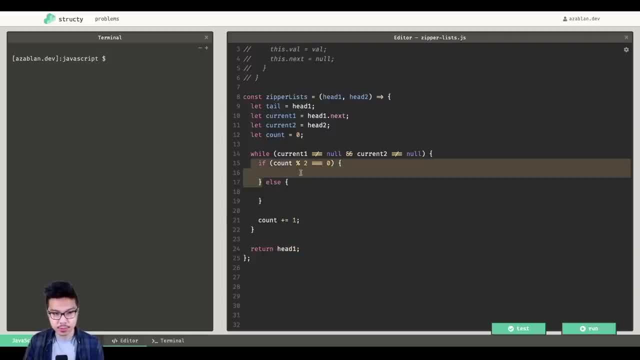 guess when my count is zero, I'll take something from list two. So what I can do is take whatever current two is pointing at. So current two. And I want to make that the next of the tail right tails helping me build the output. So simply, tail dot next equals current two. Nice, Then from there. 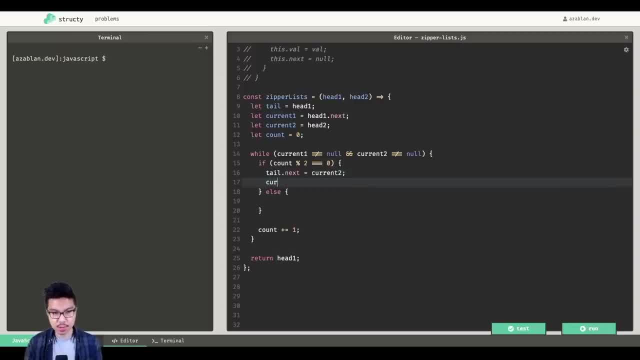 since I just used up something from list two, I need to progress that. So current two equals current two, dot next- And I know that this code over here, when it's odd, is going to be symmetric just for current one, And in addition to that we need to make sure that we also move our tail, pointer. 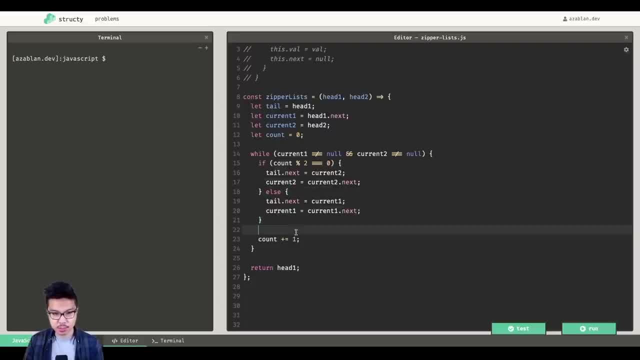 that's going to happen in either scenario. So I can put that mutual code over here. I think I'll say tail equal tail, dot next Nice. So this should help me construct my alternating pattern. But we have to worry about is based on my while loop. this while loop is: 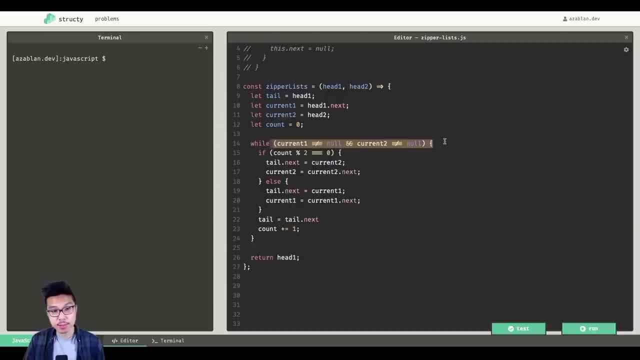 going to terminate or end. So I'm going to say tail dot next equals tail dot next. So I'm going to end as soon as one of my current pointers hits null, and it could be the case that only one of them is now on. the other one is still pointing to same data And, like we said in the 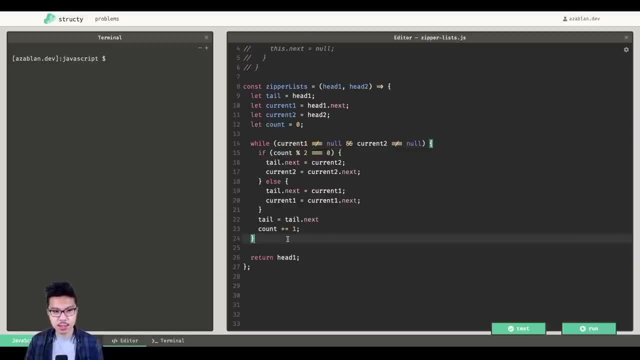 approach. what we should do is just tack on all of the nodes of the other list to our final output here. So what I'll do is I'll check here. all right, if, let's say, current one, if it still has stuff, so it's not equal to null, that I can just take that stuff and add it to. 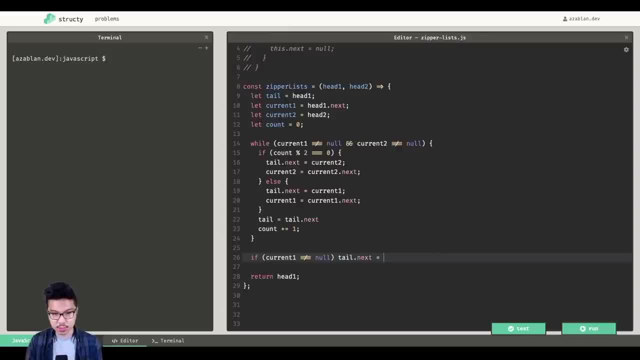 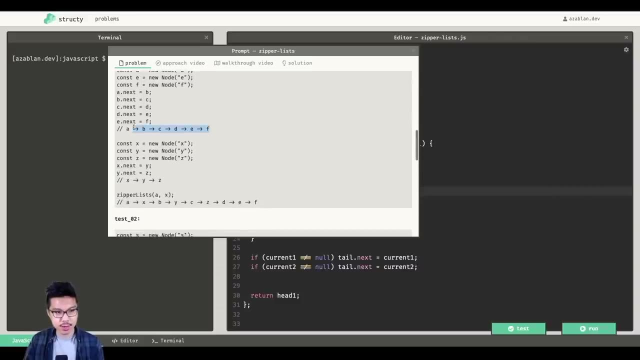 Well, dot next equals current one And symmetric for current two, of course. So if I look at the prompt over here, we're thinking about a scenario like this one. right here, we know that current one is way longer than current two, or at least one is longer than list two. 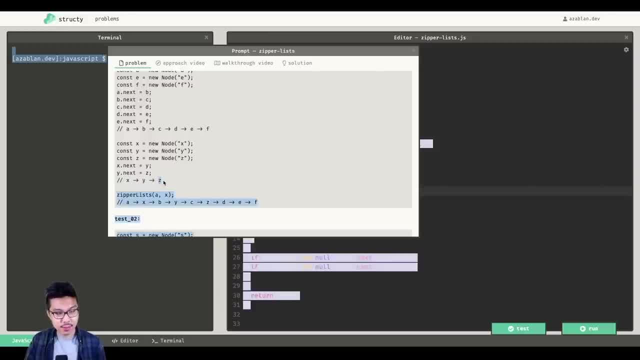 And so by the time we get to the end of list two, we know that roughly we're going to be at about this C node or this D node in list one. we just want to take all those remaining elements- looks like D- and add it to the end of that list. Notice, I just end in D, F, Cool. 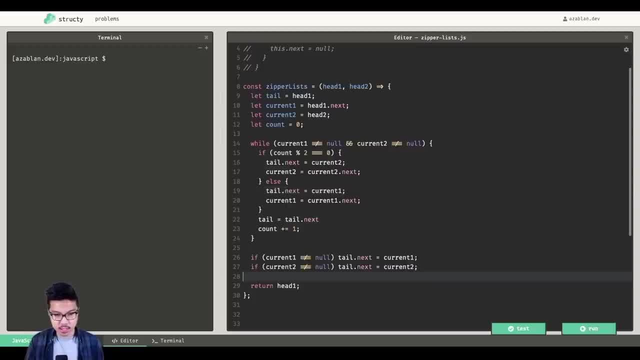 And we just need to check both sides of that. Awesome, I think at this point let's give this a nice test run. Good, always debug it together. It's not too long of some code, but it does have some interesting patterns- Awesome. Here we have a nice iterative solution. 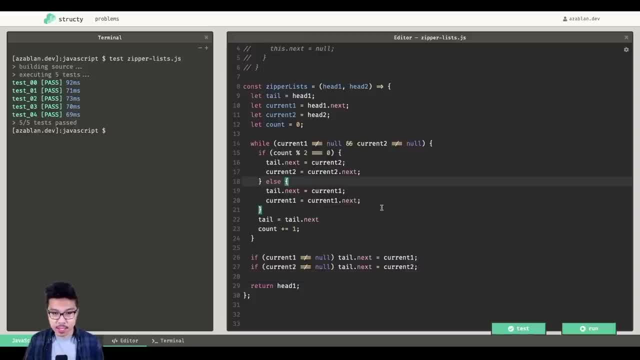 for zipper lists. For this code we're looking at a linear runtime and constant space, So I think we'll do is. let me also show you how you could solve this one recursively. It's very similar in strategy, somewhat shorter code, And I'll leave it to you whether or 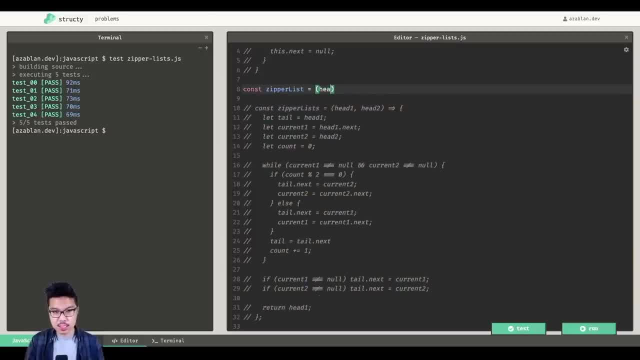 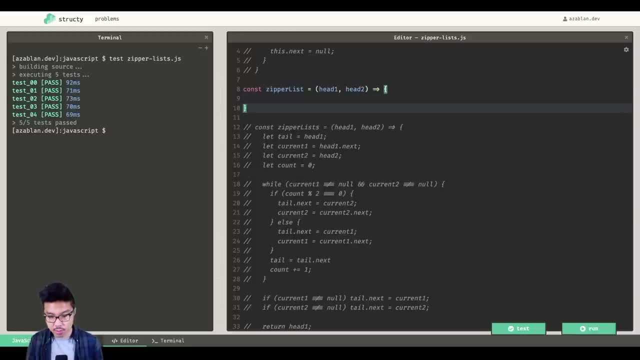 not. you think it's more simple or not. We will have to concede, though, that for any recursive code, especially for this one, we're going to have some additional stack space used, So we would have a linear space for recursion as well. So I'm going to do my best to translate. 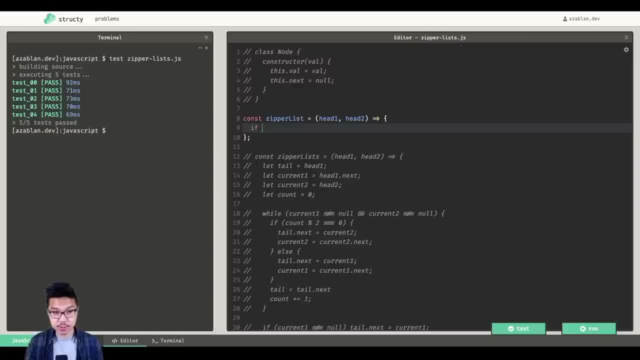 these patterns. So I know I should stop my recursion. We'll say: if head one is no and head two is no- So that's very similar to what we just said in our iterative version- And if they're no, then you kind of hit the end. 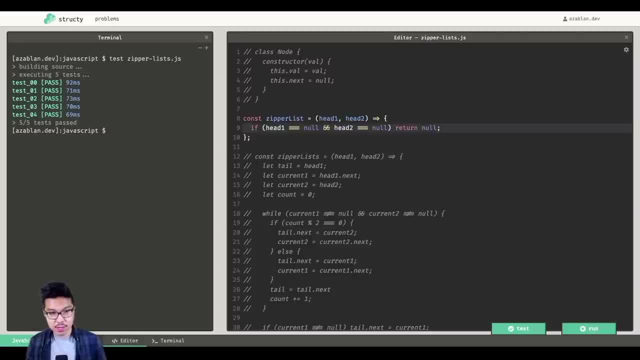 you can just return. no, what I have to be sure I do is for my function. it needs to return like the new head of the linkless, And so I'll just have some base case here where I return. no, Because basically a link list contains like many sub lists. 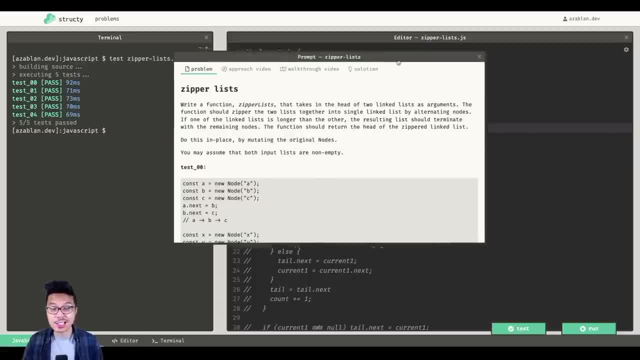 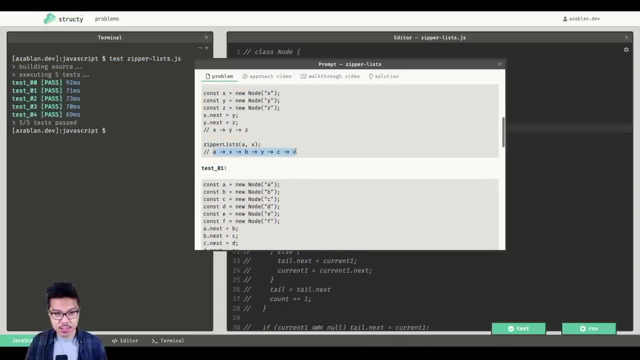 Right. What you should be doing as you solve link list problems recursively is if you think of- let's say this- as a link list- going from A through Z, then going from x to z is also a link list, going from B to z is also a link list. So that's how I kind of break. 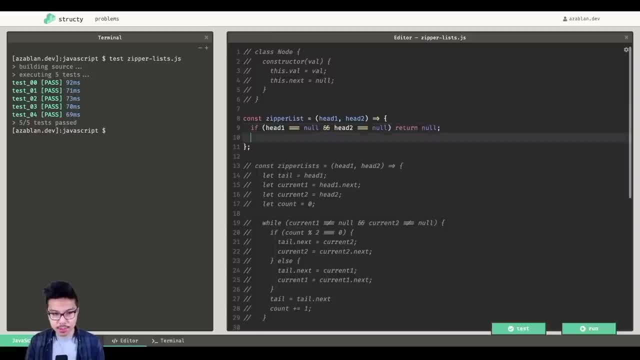 down my problem size. So if they're both null, then return null. But what if only one of them is null Right? So what if head one is no Right? And that would mean, if head one is the only one that's not, that means head two has some stuff. well then just return. 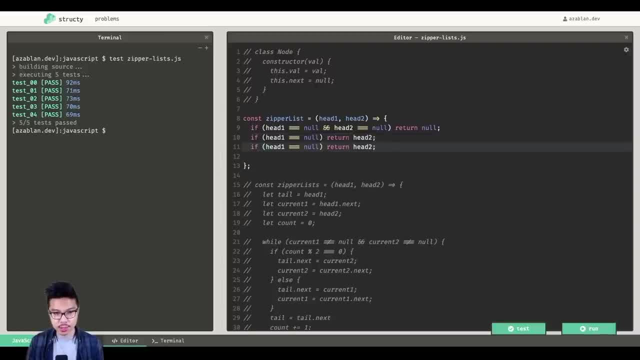 the remainder of head two and make that symmetric for the other side, right. So if head two is no and head one isn't, then just return the remainder of head one, And what this base case over these base cases will let me do is accomplish some logic, just like this. 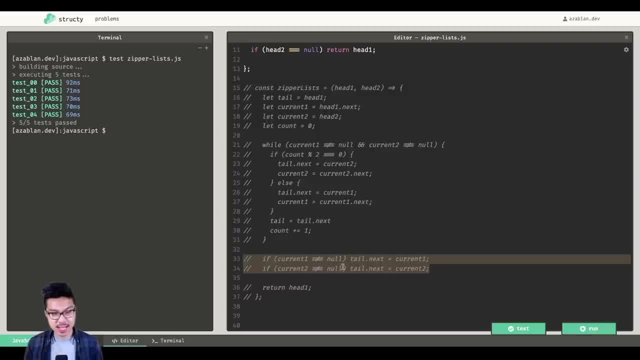 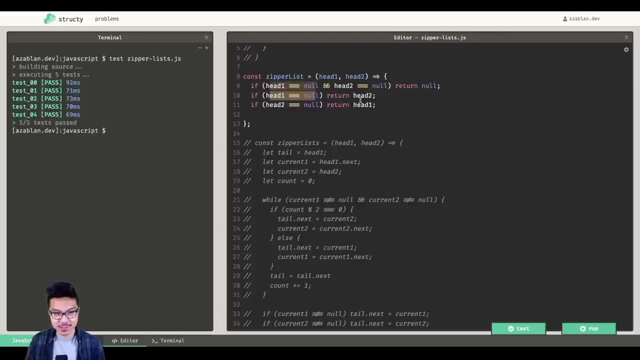 right, How can I take all of the leftover nodes in the case of one of my lists running out and just tack it on to the end? Right, If one of my pointers are in the middle and it runs out, I'm just going to return the other pointer. Cool, which would be the leftover. 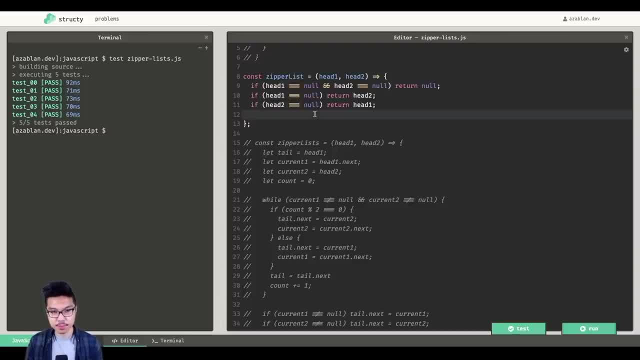 chain. Now I need my recursive code, So there are a few ways you can write this. Instead of using the modulo trick and checking for even or odd, what I should be able to do is take two nodes at a time here. So let's say, I know I need to make my head, had one really. 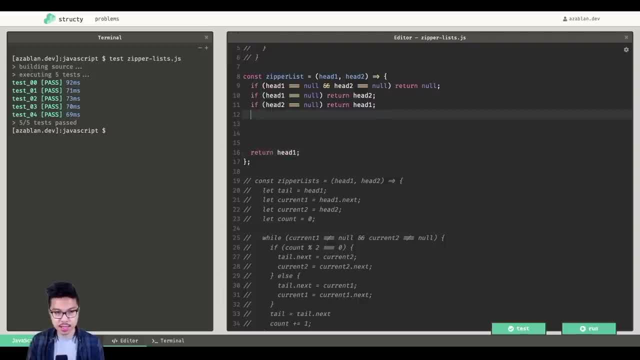 so I'm going to return head one, I think, at the end, and I need to make head one dot next, and then I'm going to make head one next point to whatever head two is Right, And as soon as I do that I would actually lose access to the original head one next. So I 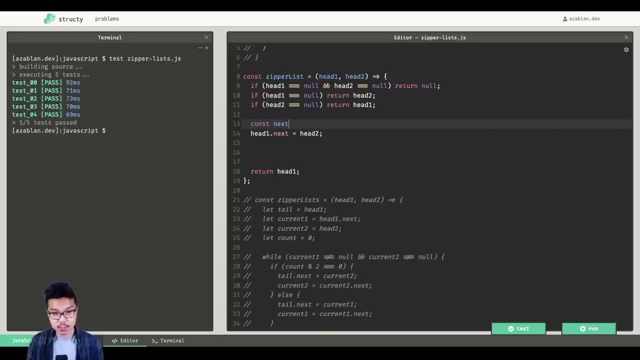 should have saved that. So I'll say maybe const next one equals head one, dot next. before I overwrite it, And I guess why not while we're here, we'll also do the same for next two. pretty common thing we have to do for a linkless problems right Before you overwrite. 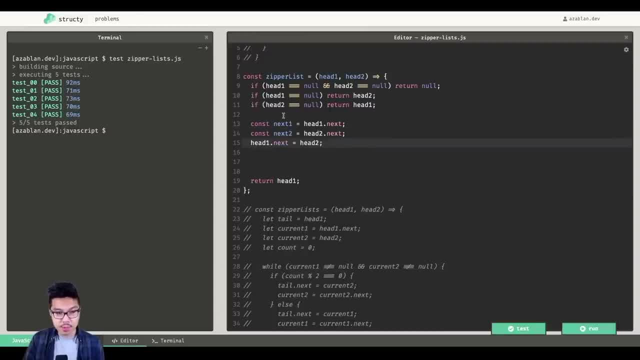 a pointer. maybe save it in case you need it still. So I'm making head one, next point to head two, And then from there I know I need to call recursively zipper list on next one And also next to it. should be right. And then from here I just chained head one to head two. I know zipper list is going to. 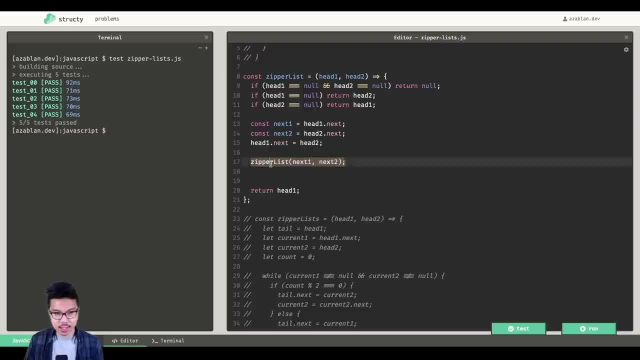 return the head of the remaining linkless. I just need to chain that to head to so head to dot next equals that return value because again I'm going to return a node from this recursive call. So this code is looking pretty good. Let's go ahead and test it. It is quite a bit shorter, So we're. 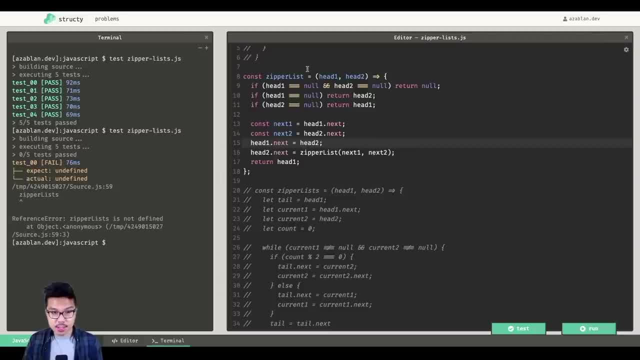 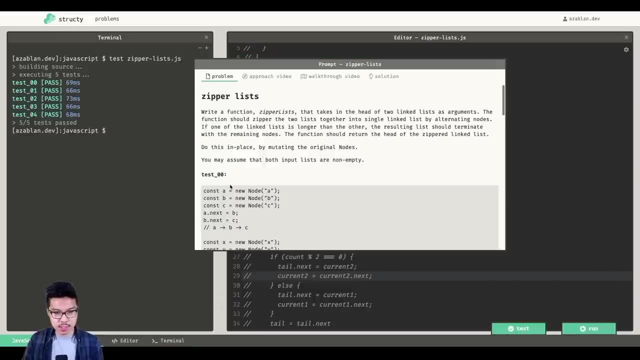 getting an error. zipper list is not defined, Because I need s here, That's on me. Give that a go again. Little typo there, Nice, And here we have a nice recursive solution for this. And so just make sure, on the same page here, maybe it's worth stepping through at least one iteration. 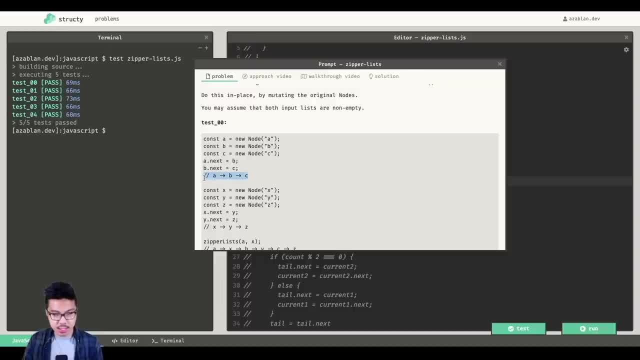 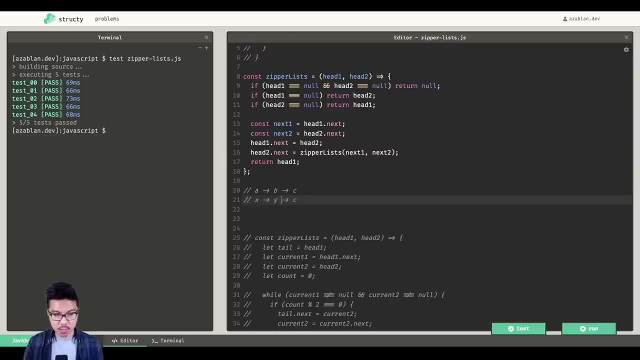 together. And so let's say I had these. let's add ABC and x y z, trace through at least one stack frame of this. So ABC and then x y z. Alright, so I know, in the context of my pointers I have h1 over here. 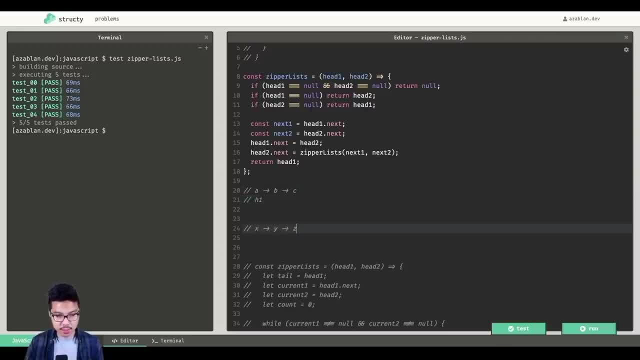 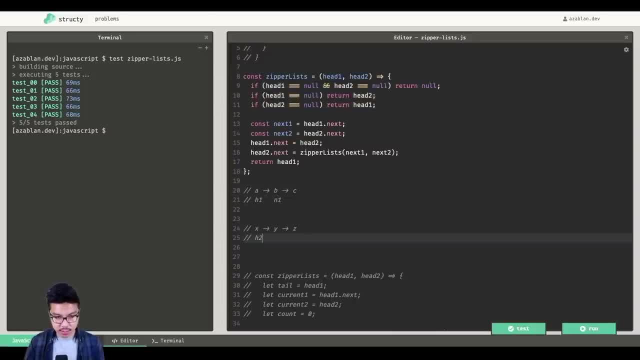 nothing fancy here. I have next one over here, I have next two over here And in the core logic of actually alternating, what I do is I take head ones dot next and point it to head two. So I don't want to just kind of merge them together in line over here, So kind of separately. 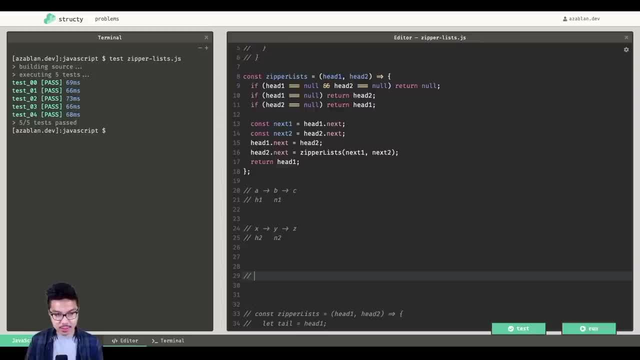 although you know I'm not creating new nodes- would look like this: head one is a. I said it's next to x, So that already looks good to go, And then from there I set head twos next to whatever the recursive call is when I pass along: next one, next two. So at this point, 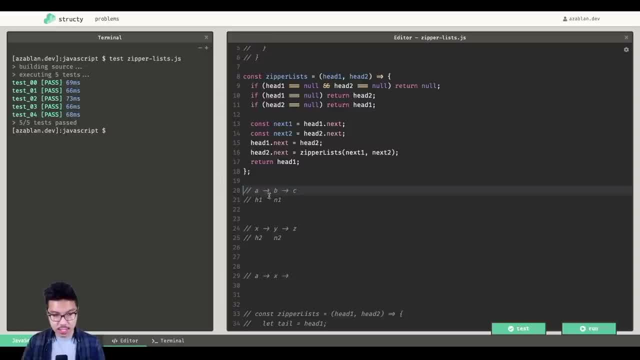 I can kind of ignore these right, So I'll take out just this, a node. And now h1, or head one points to be the same thing over here. h2 points to y, And let's say we step through this iteration. 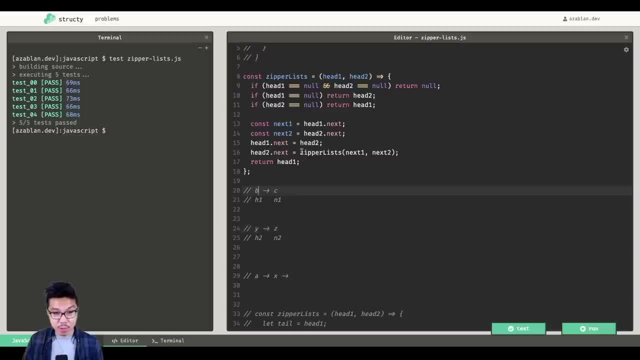 well, same thing. I just take head one and I know I'm going to return head one, right. So eventually it's going to return over here. It's going to say b points to y right, Because head one is b, h2 is y, head one dot next equals. head two, And that's good to go. 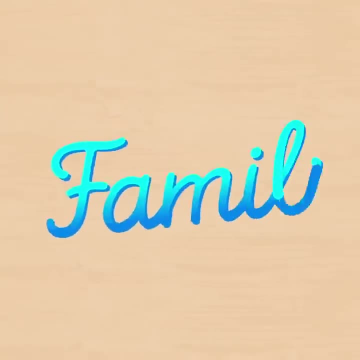 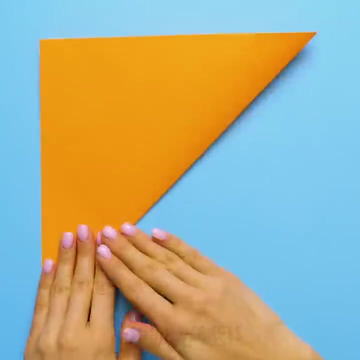 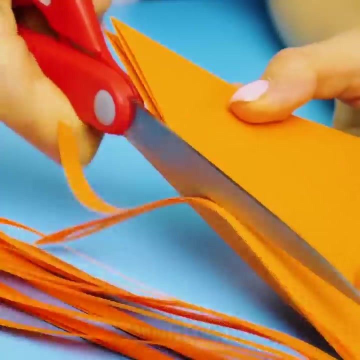 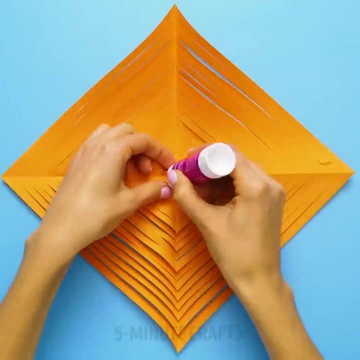 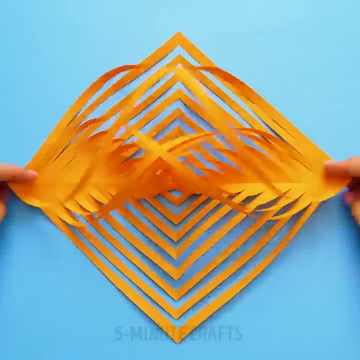 I know I messed it up, but in my soul I feel a love for you that's out of control. Sometimes I feel like I can make you whole. I just can't change my emotions. There isn't anything I wouldn't do To prove that everything I say is true. Emotions: Baby, I know this might sound insane, But, baby, you're gonna love me again. Love me again. Yeah, I paid my dues to show you I'm not the same. It has cost me much, but I would do it again. So, baby, come on, love me again. Love me again. I know I messed it up, but in my soul I feel a love for you that's out of control. Sometimes I feel like I can make you whole. I just can't change my emotions. Come on, love me again. You're all I need.